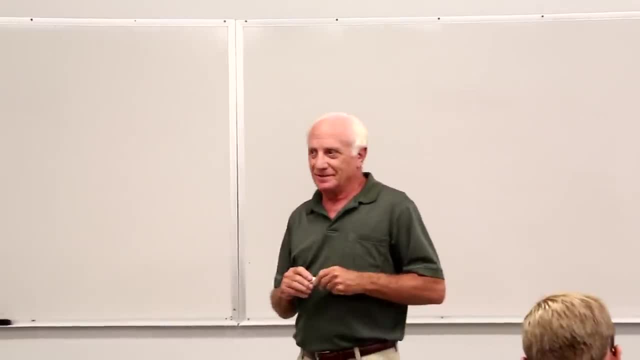 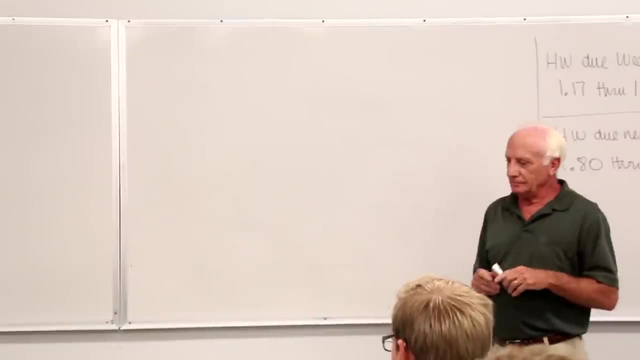 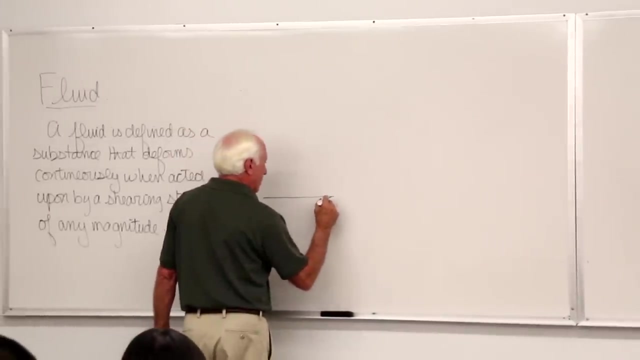 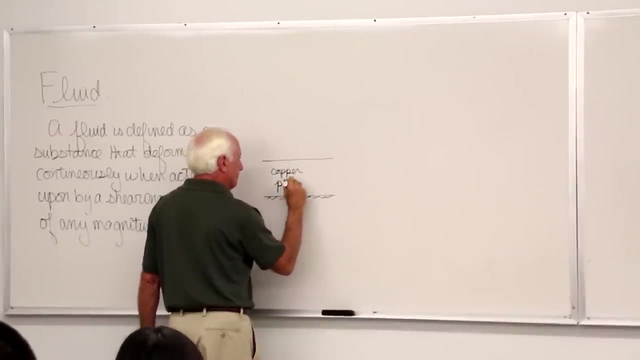 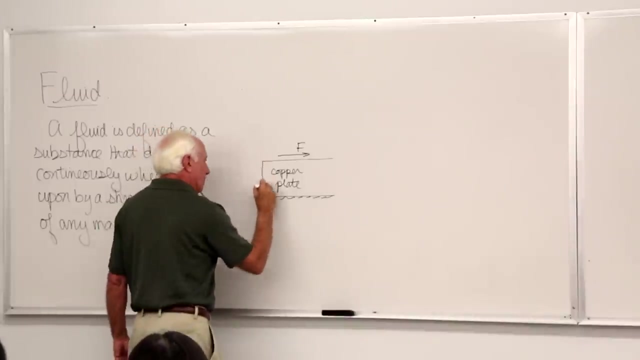 How many people here have had ME 218 strength materials? Almost everybody, of course. Take out a piece of copper plate- copper plate, I don't know, an inch thick, six by four, something like that. apply 400 pounds on the. 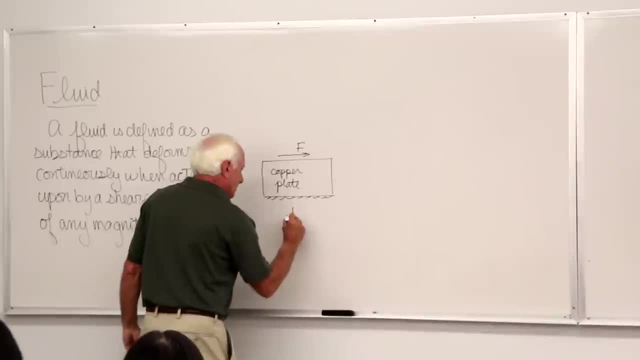 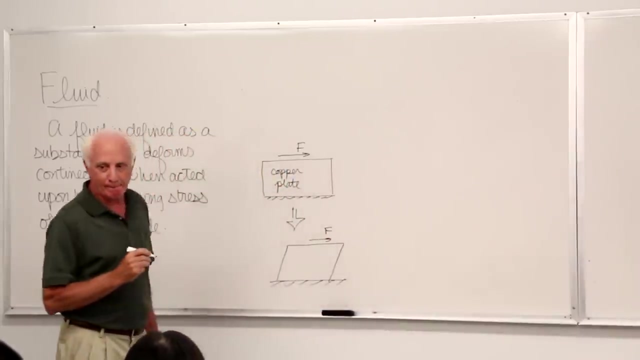 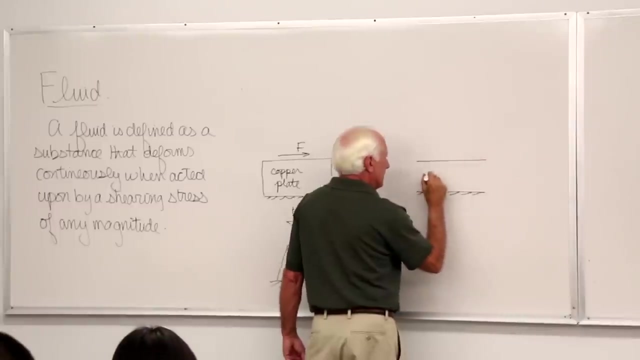 top of it. This is fixed with a base When you apply that force to it. you know any 218, for instance. there's the plate. Now again, here's the ground. Now I take a layer of water, I apply a force. 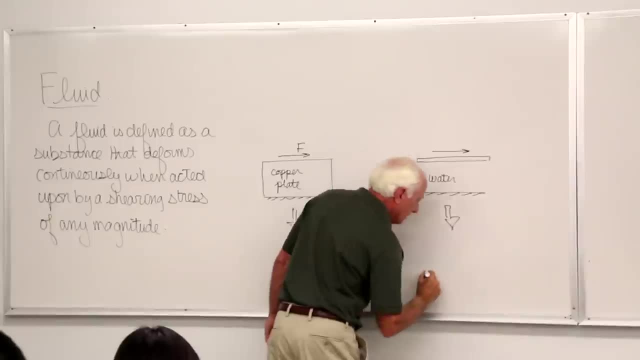 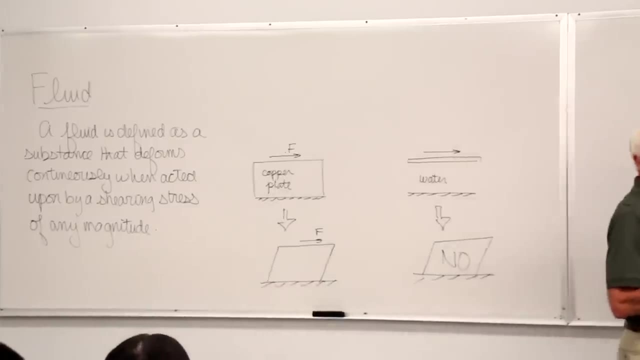 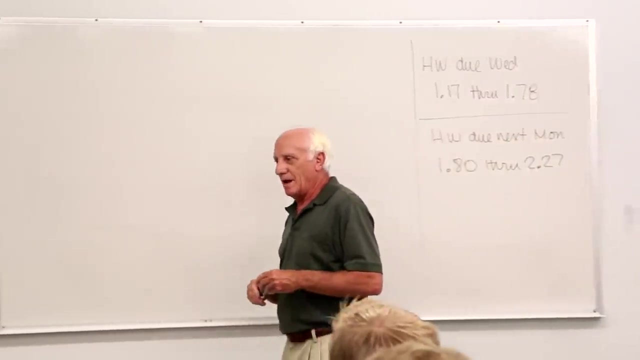 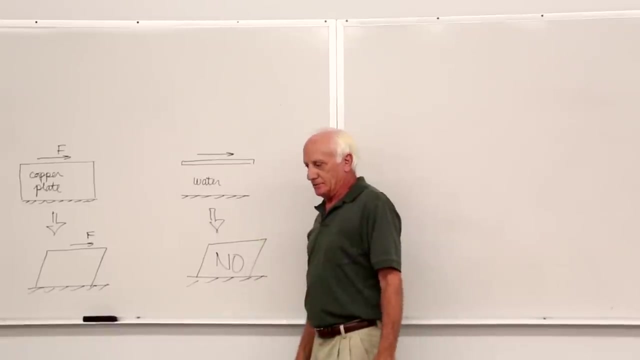 This is fixed with a base. It doesn't look like that. when I'm done applying a force to that plate on top of water, Think what would happen if you applied a force to that plate on top of the water weight. I applied 10 pounds. 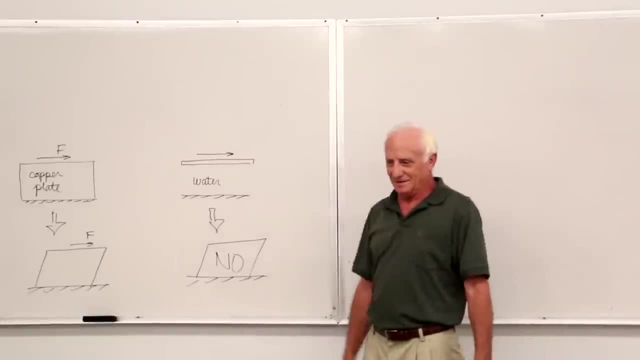 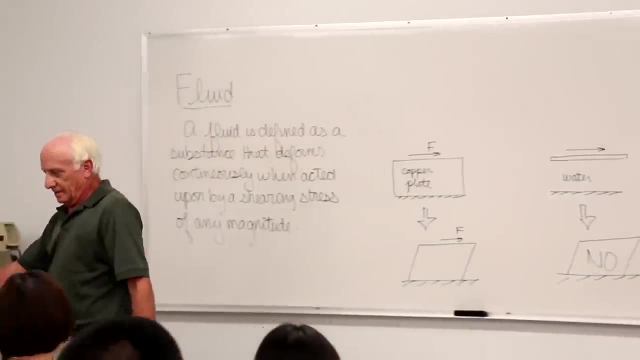 Would the plate ever stop? Of course not If you applied 10 pounds. this is a room flooded with water. this high, I'm walking in the water on my knees. I put a styrofoam plate on top of it. I push on it. 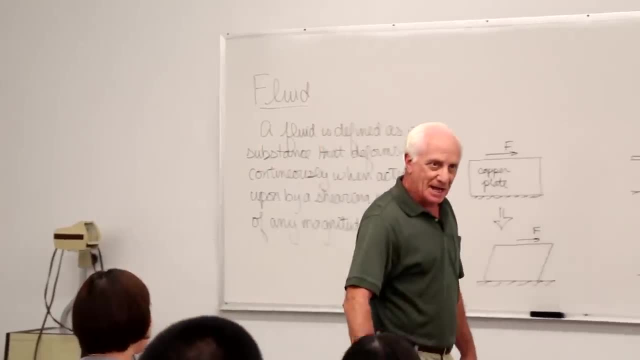 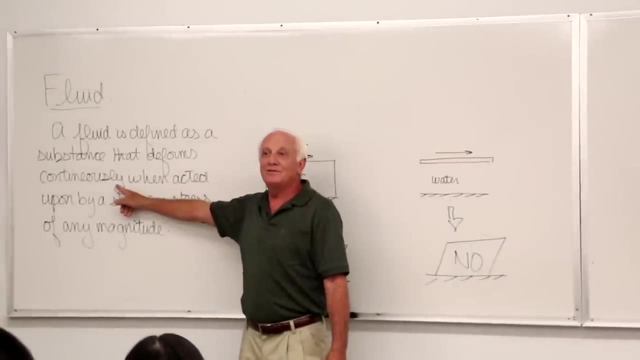 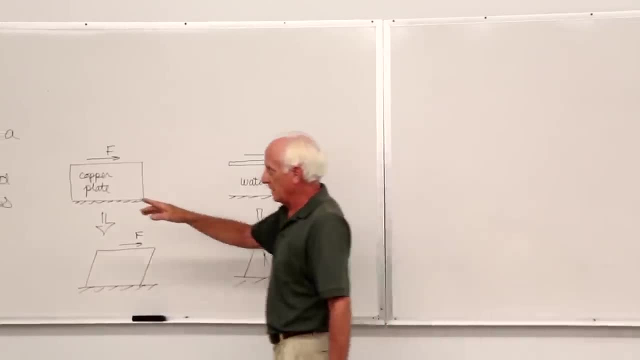 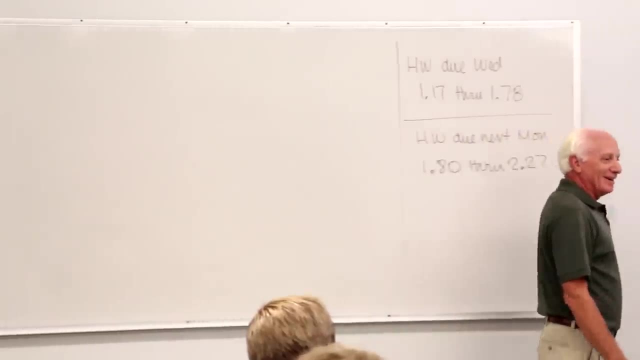 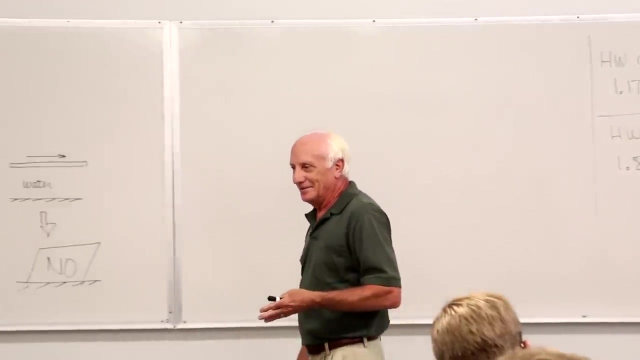 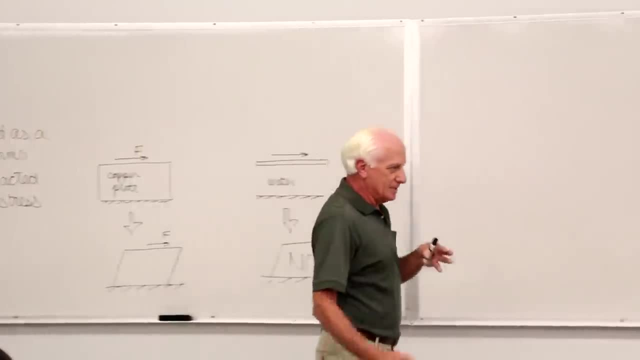 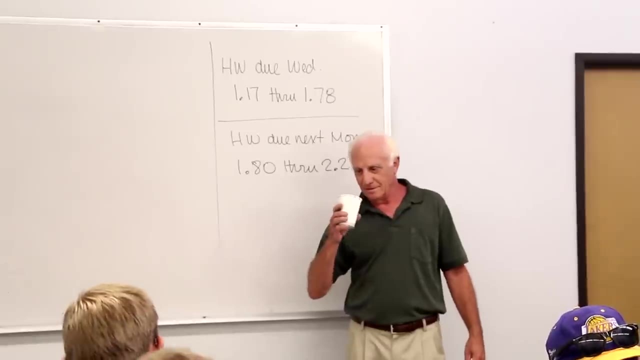 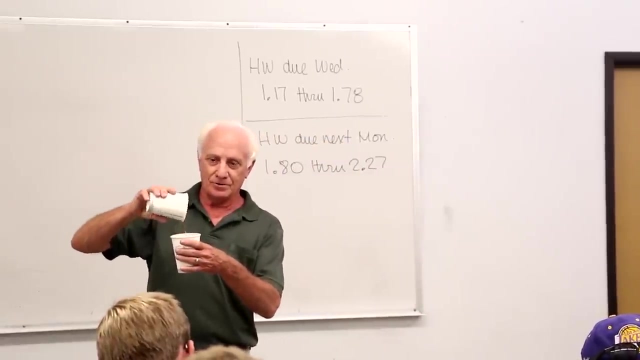 fluids. Now, there's different kinds of fluids, though We're, all you know, used to fluid water. Okay, Okay, I'll be working out of there. It's working really nice. it's working really nice. What's in this cup? 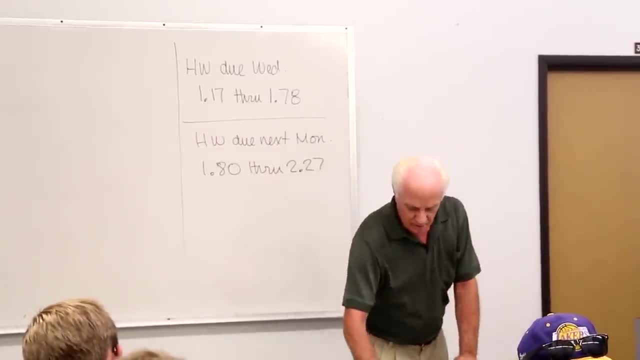 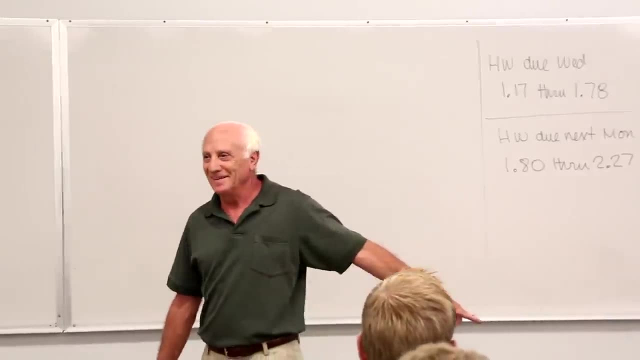 What's in that cup? Now fill that cup there with cold air. Try and pour that cold air in that cup over there. Oh, it won't do it. It won't do it, It'll spread out when it comes out. 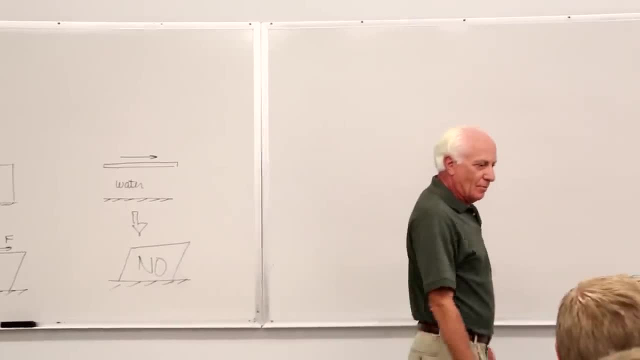 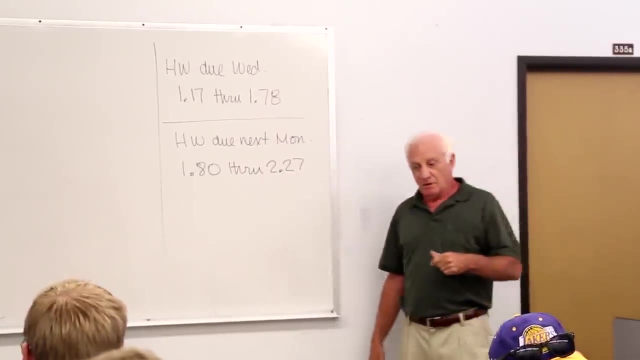 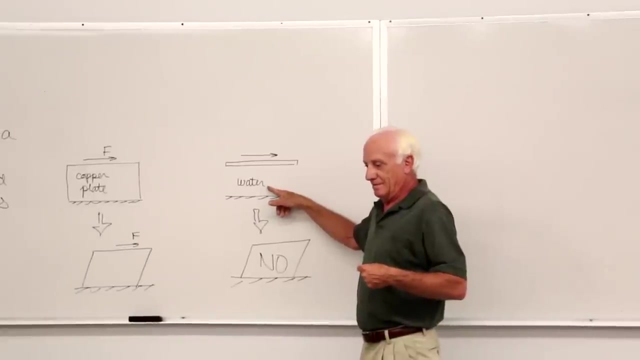 It'll go all apart in a big plume. Why? Because the molecules are not attached to each other as strongly as they are in that liquid. Are they both fluids? Oh sure, Of course they are. Put air in here. Push on a plate and air. 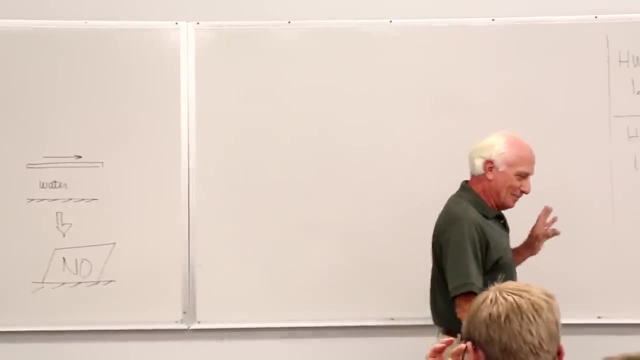 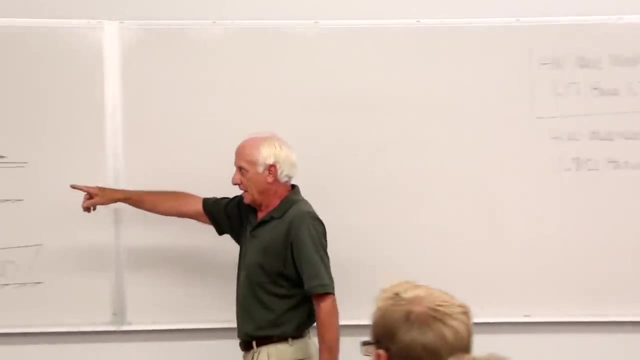 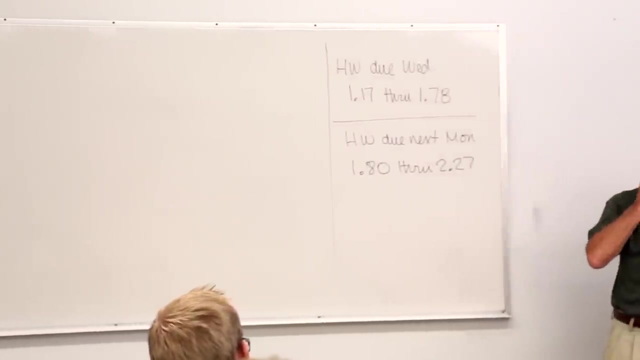 It was done. Yeah, they're both fluids, Liquids and gases, But not solids. Not solids. Well, maybe not quite, Maybe not quite. Take the cap off The toothpaste, Turn it upside down. Does it run out? 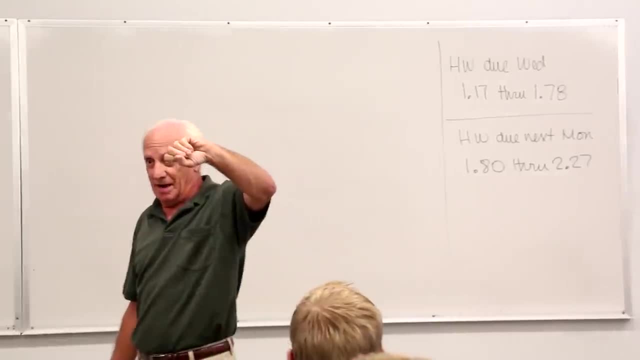 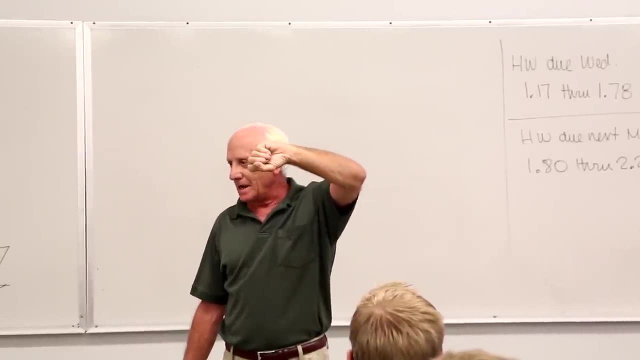 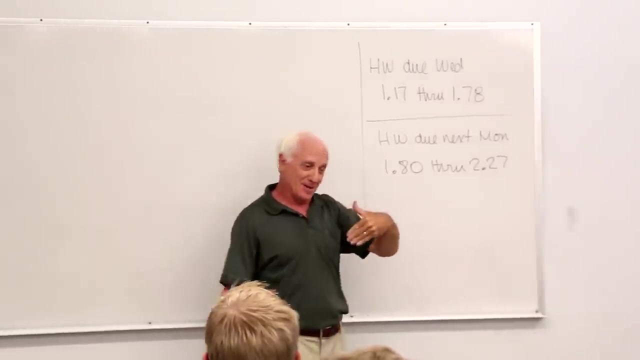 Really No. This has been in the car for a few hours and there aren't any temperatures. No, What makes it come out? I've got to press on the tube. Okay, so it takes an initial stress, shearing stress, to move it, to get it moving. 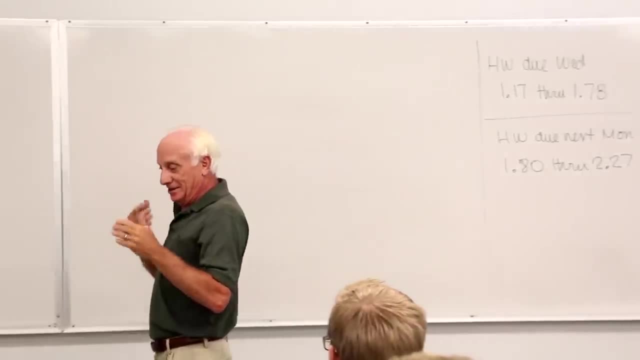 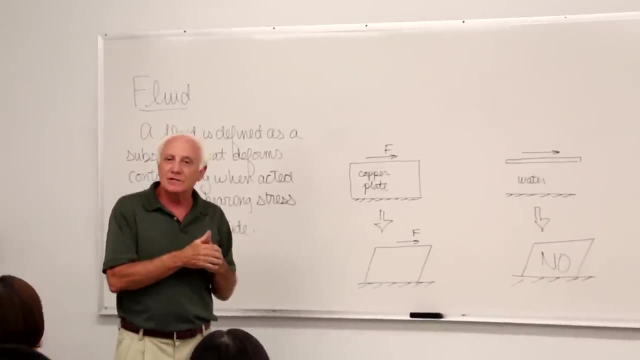 Once it's moving, it moves pretty good, But it takes that initial shearing stress. It could be, you know, some very thick things, like some epoxies. you know You can come check it out. They don't come out until you squeeze a tube or a plunger. 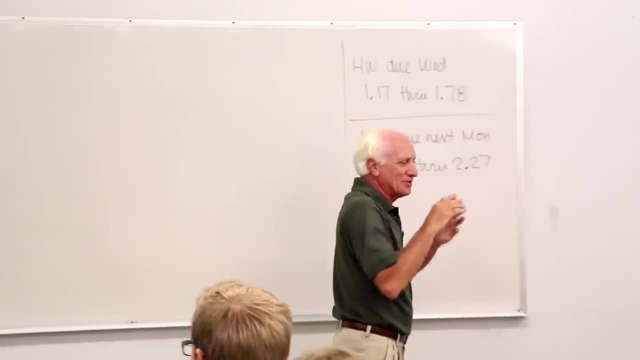 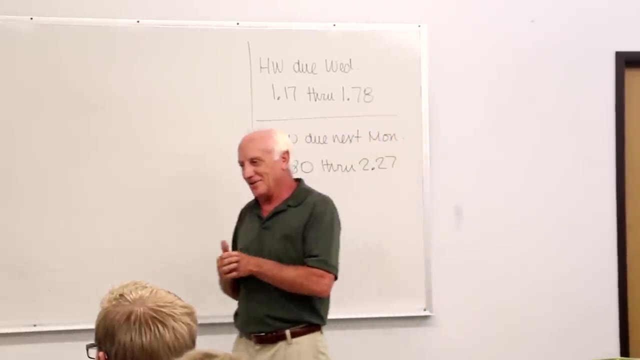 So yeah, those things are kind of like fluids, but we won't discuss those in this class. We're not going to worry about, you know, toothpaste and epoxy and things. We'll worry about water, air oils, things like that. 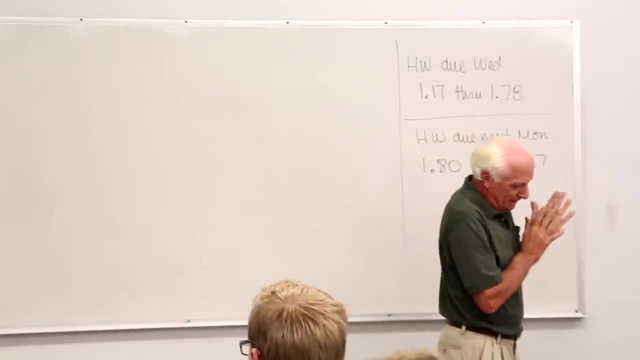 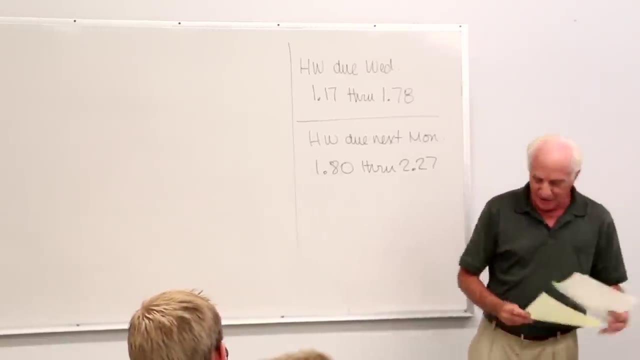 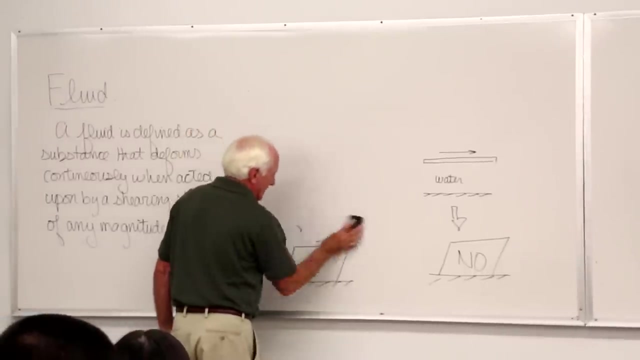 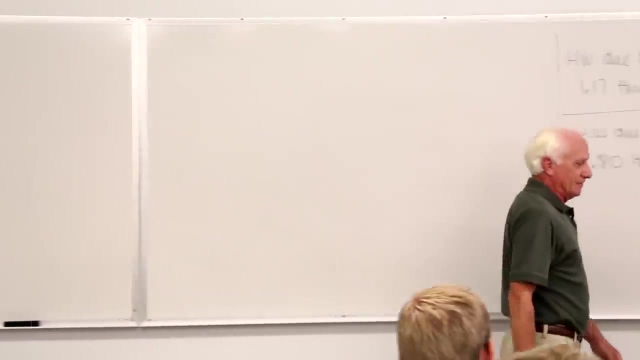 Helium Freon, you name it. So that's a big difference in that And we're going to talk about that. But we're also going to look at two sets of units. You know a lot of textbooks now. they are almost always almost all in SI, which is so much easier than the British system. 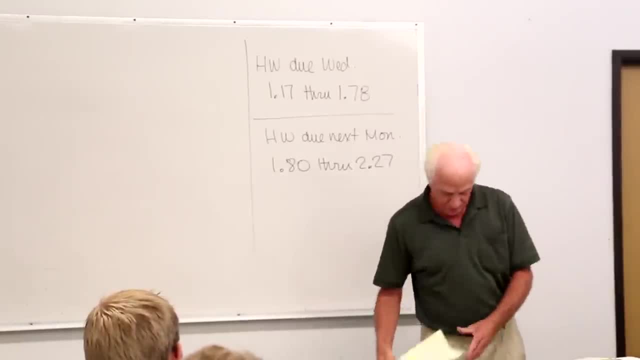 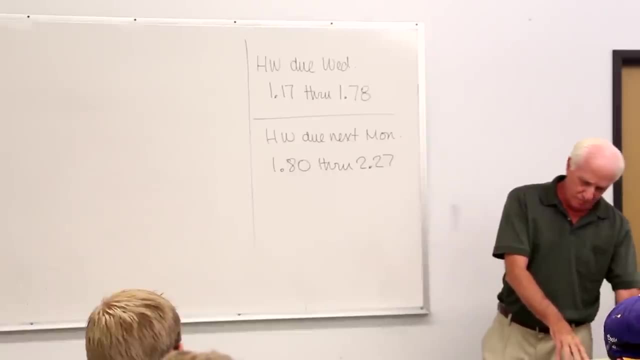 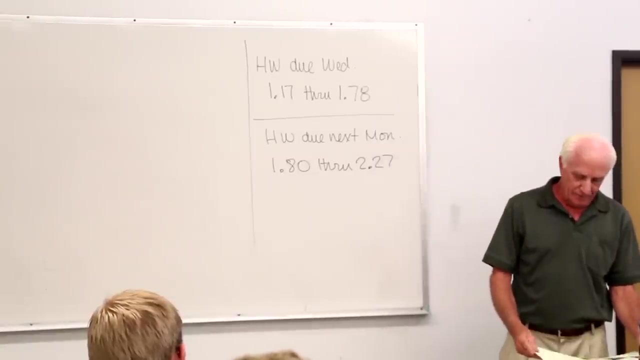 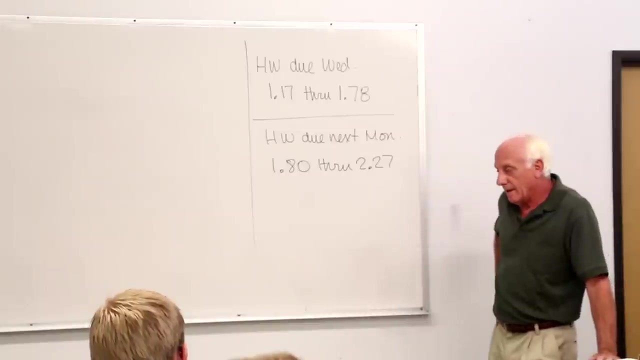 So much easier. But unfortunately the real world doesn't go that way. So our textbook- I forget the percentage, but it has quite a few. I'll call it English, it's British gravitation- Quite a few problems, whether they're example problems or homework in English, and then a lot of SI, a lot of SI. 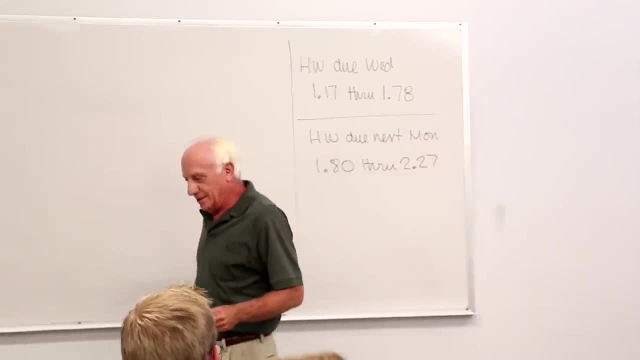 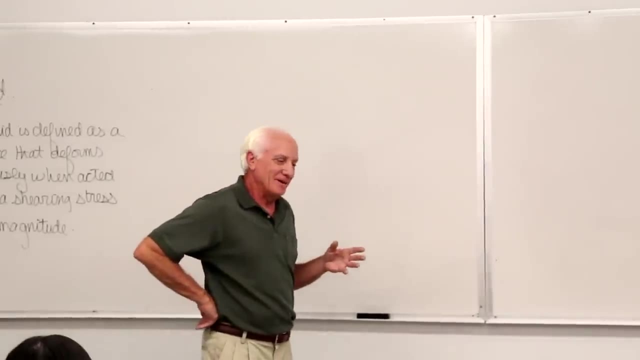 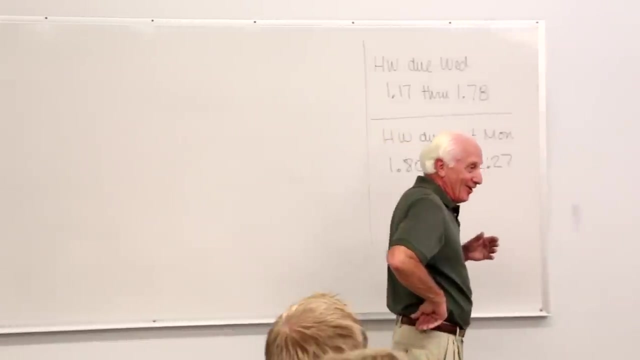 But you graduating, have to be conversant in two languages, Otherwise you're not going to show off very well in the real world. You have to know two languages, Forward and backwards, Really really well. The easy one is SI, The hard one is English engineering. 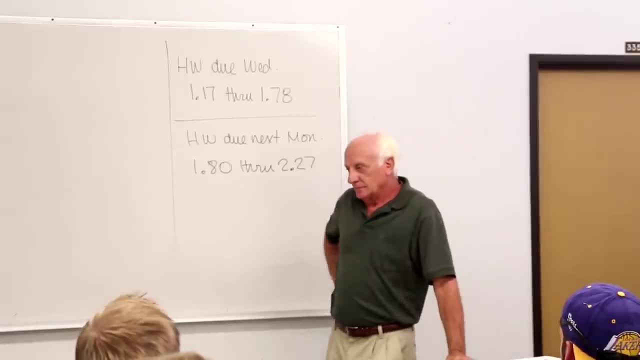 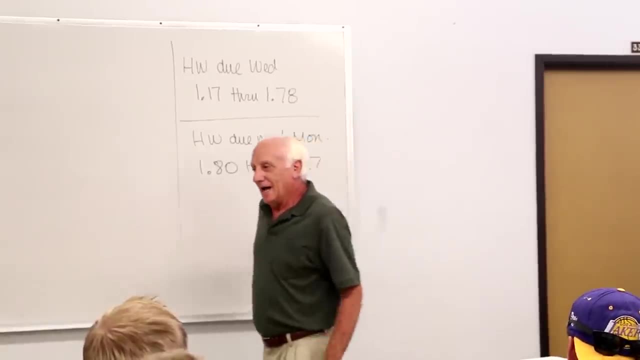 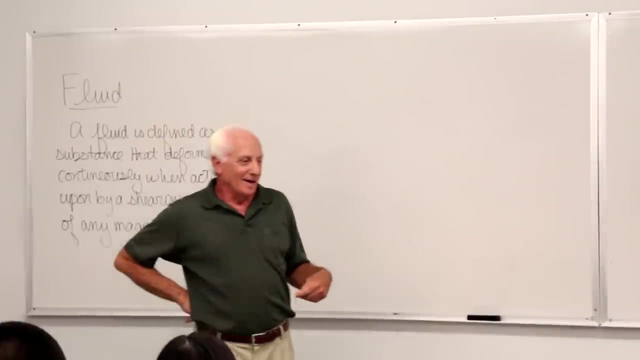 For instance, how many centimeters in a meter? Well, I'm trying to guess that. Okay, How many millimeters in a meter? I'll tell you about a thousand. How many cubic centimeters? 50 centimeters in a liter. 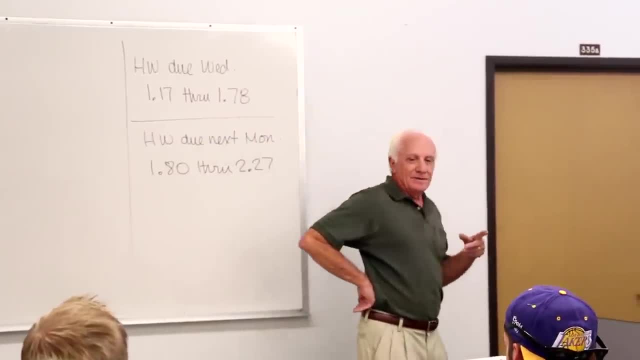 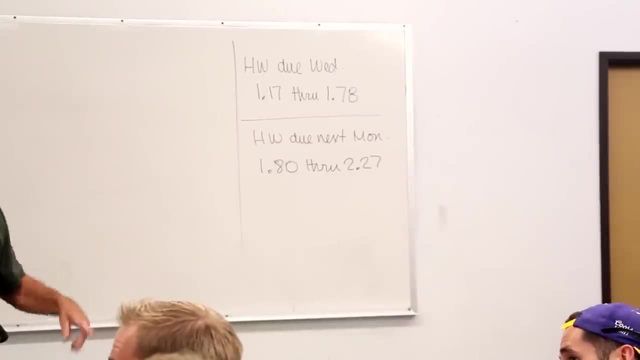 I'll tell you, It's a thousand. Do you get the point? Everything in SI. would you go out there and fill that door please? Okay, thanks, Everything. every conversion factor. Okay, we'll tell the other one. 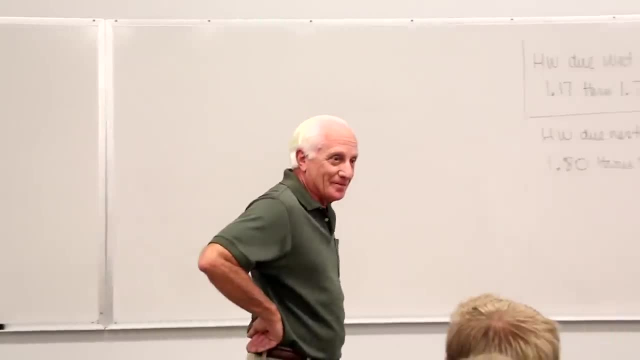 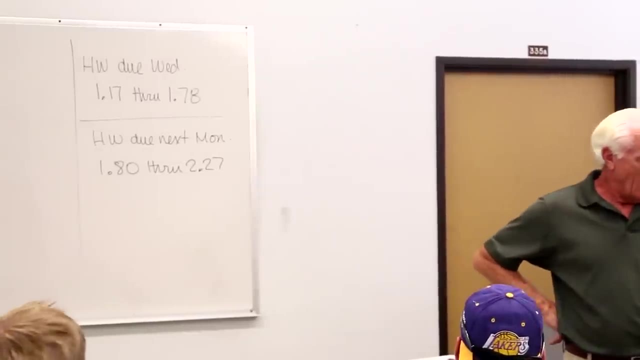 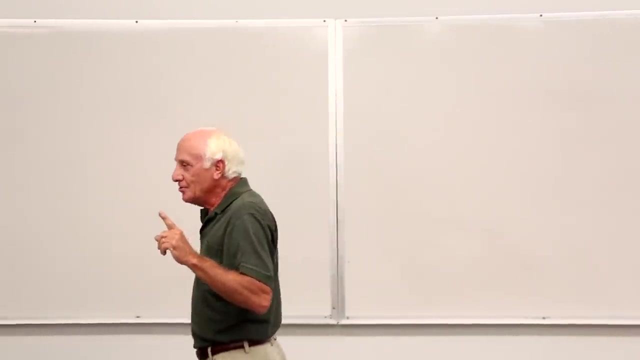 One joule divided by one second. What is it? Joules per second? One, Yeah one. Is it one? Yeah, it's one, Okay one. Everything in conversion SI starts with a one times ten more power. You can't get any easier than that. 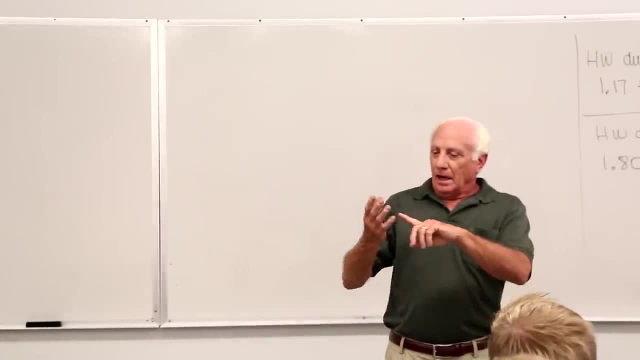 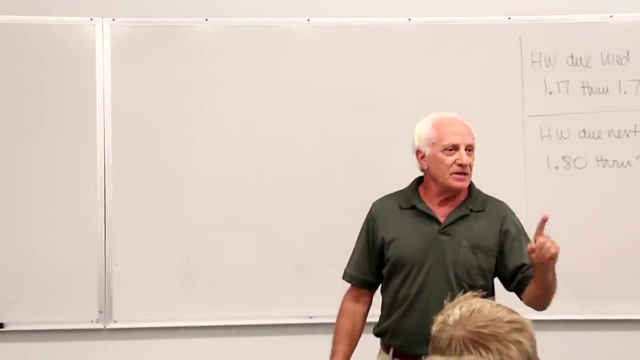 Now you tell me this: How many pints in a quart? How many quarts in a gallon? How many gallons in a barrel? Ho, ho ho. Nothing starts with one, Nothing. Well, memorize that stuff. No, no, no. 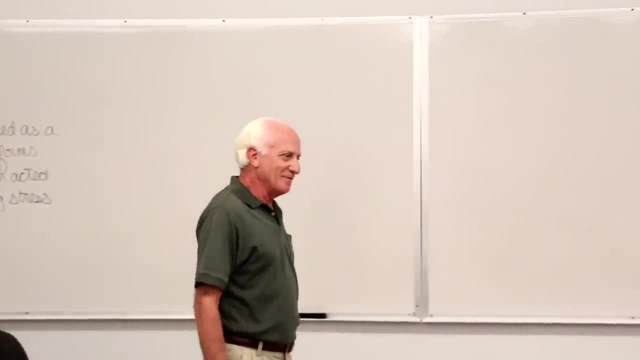 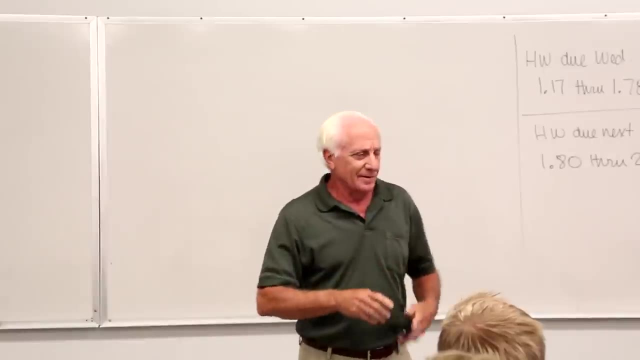 You don't memorize this right here, You're doing it. It's still kind of embarrassing if you think: well, I don't know, but I've got this thing in my pocket. Yeah, I'll tell you in a minute, okay. 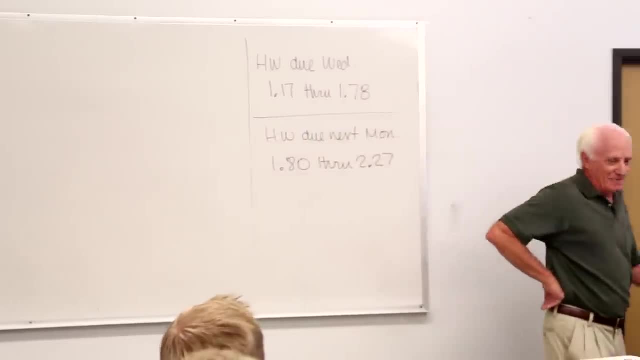 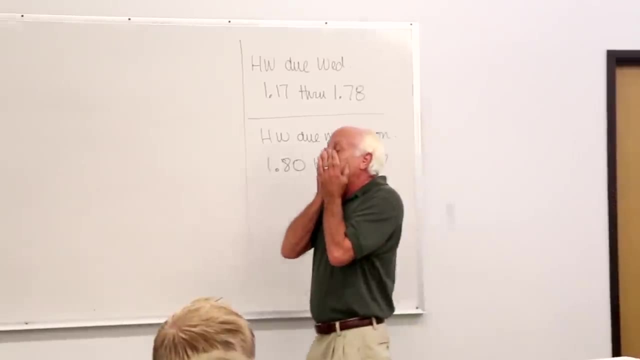 Gee, that's okay, but I mean 55 gallons in a barrel. No, it's awful. It's awful. Oh power. How many foot-pounds per second is a horsepower? Well, how many watts in a kilowatt? 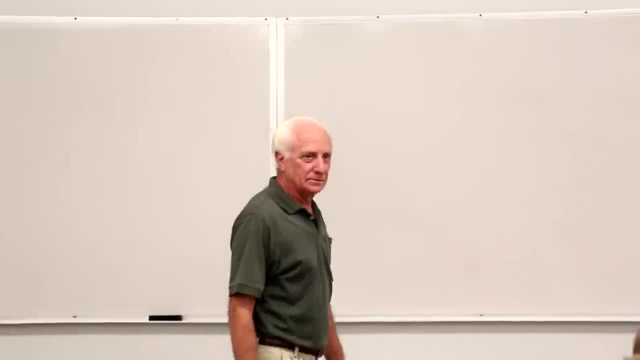 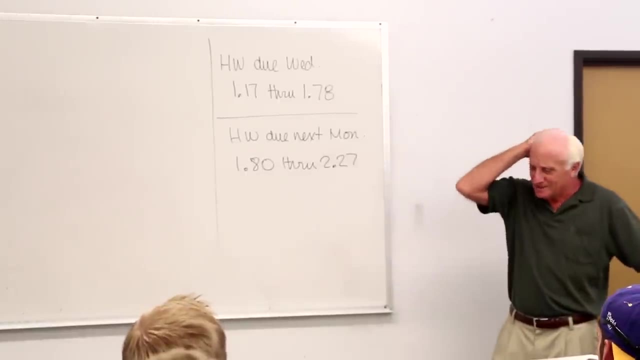 Well, I'll tell you How. about a thousand One times ten to the third, One times 10 to the third? So, oh yeah, I mean, don't you wish the whole world was SI? Of course we all do, but it's not. 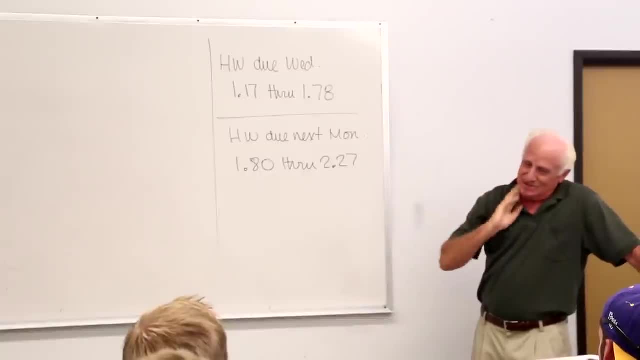 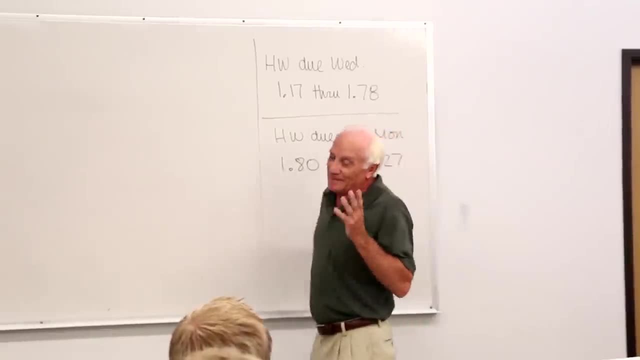 And you live in the country that's. you live in the worst country for it, The country that still has both unit systems. So you have to be really, really, really good in both of them. That's why. that's why my point is. 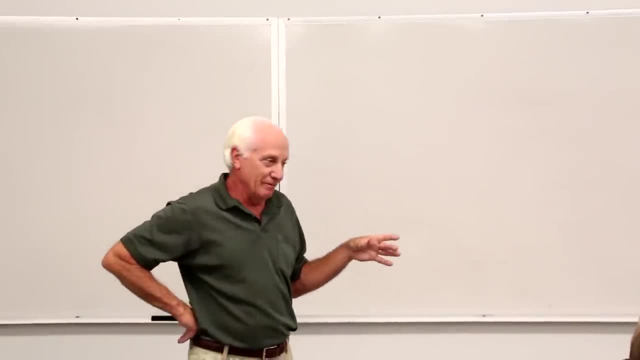 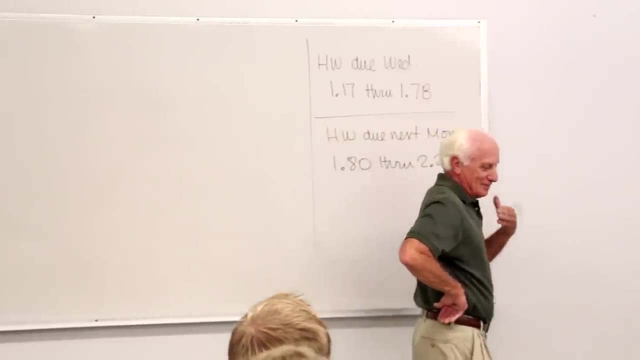 that's why, when we select a textbook, we make sure the textbook has, if we can find it, dual unit systems in it, Because we know the more you practice, the better you get. The problem is most people work problems in SI. 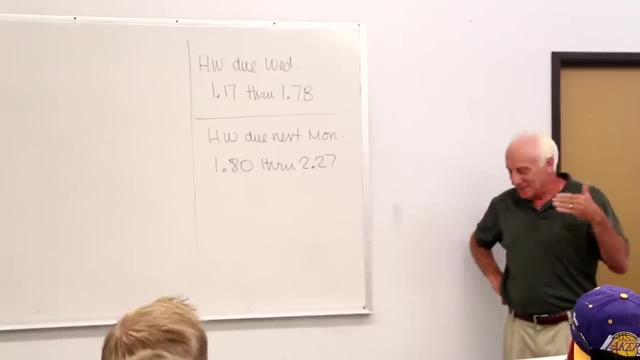 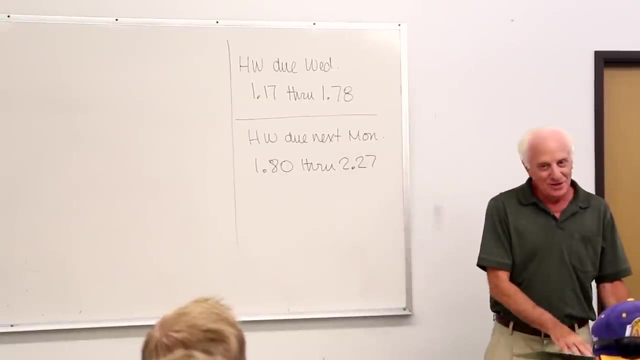 where they need to practice in English engineering. Okay, well, that's either here or there. There's problems here. There'll be problems on homework of both. There'll be problems on tests of both. You can use your. you can use your smartphone. 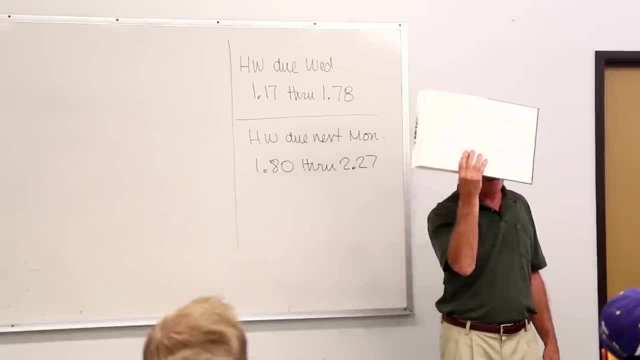 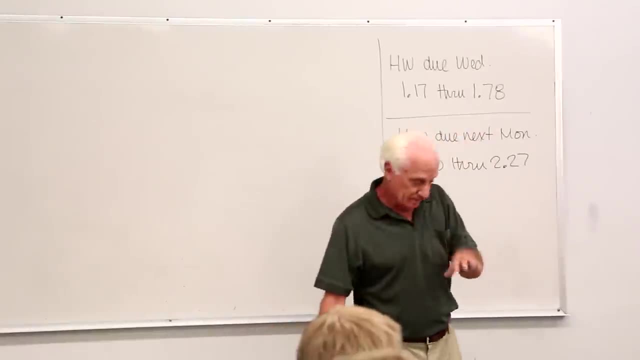 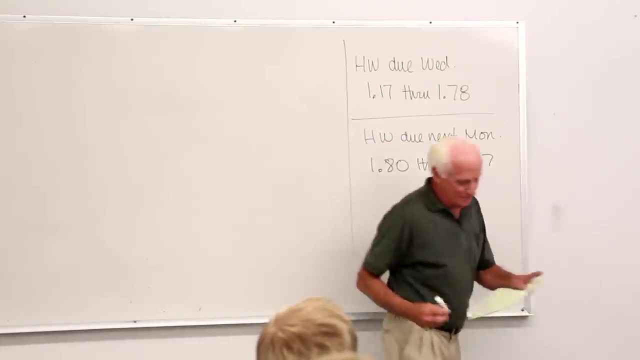 for conversions. There's conversions in the inside back cover too, SI to British gravitational. So good choice. but there will be both kind of problems for homework and exams. Okay, let's just briefly go over the two unit systems. Let's do SI first. 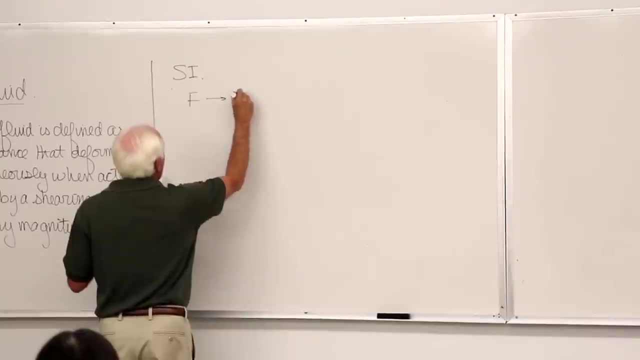 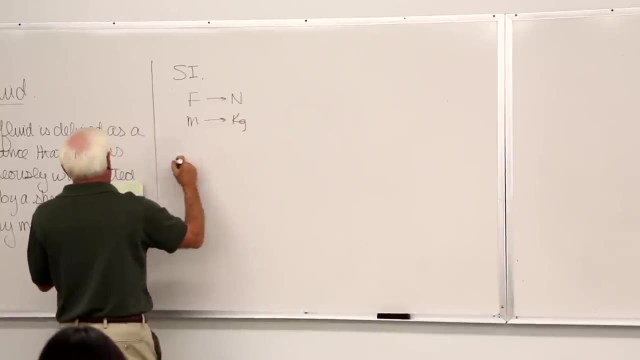 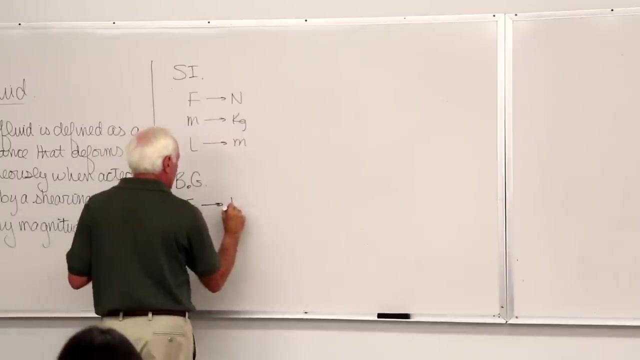 Okay, force is in newtons, Our mass is in kilograms And, of course, length is in meters. Let's do British. gravitational Force is in pounds, Mass is in slugs, Length is in feet And they both have seconds for time. 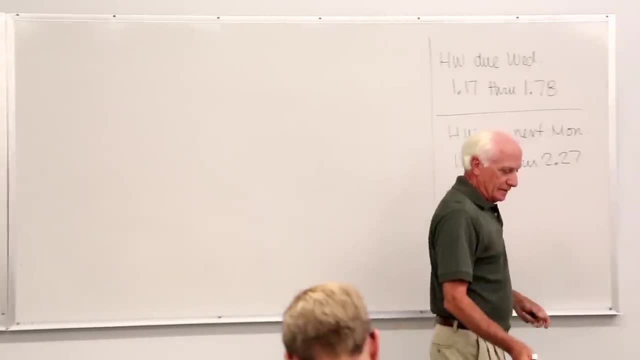 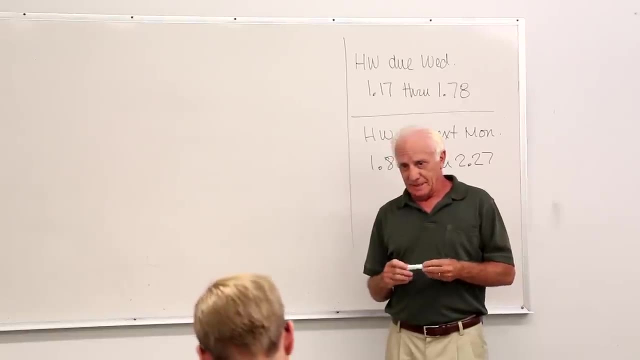 There's a third unit system that has force in pounds, force Mass in pounds mass. And then there's the second unit system, mass in pounds mass. But this is the British gravitational. You don't put a subscript on this guy because you know. 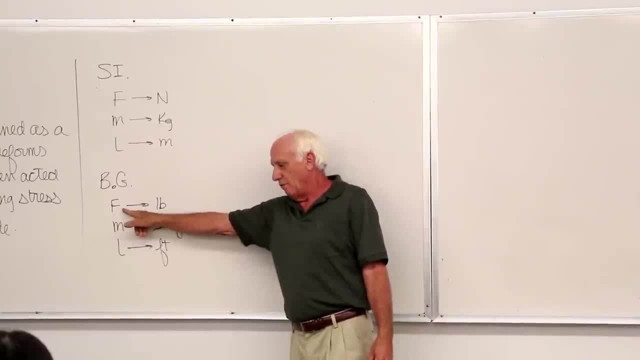 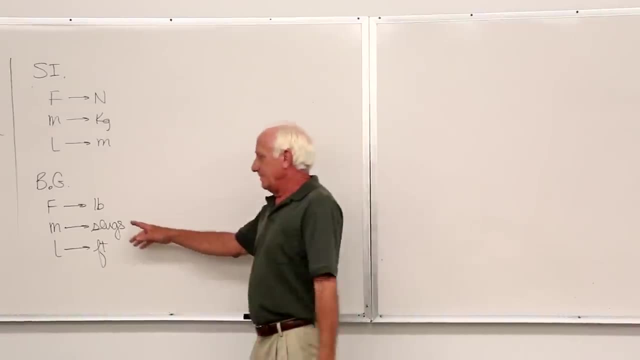 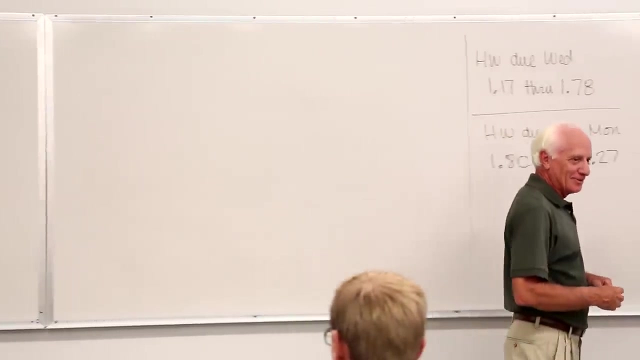 if it's in this system and it says pounds, it's got to be force, So you can skip putting the subscript F on pounds. Unfortunately, you don't deal with pounds under mass. You deal with slugs. These are not little creepy crawly, slimy things. 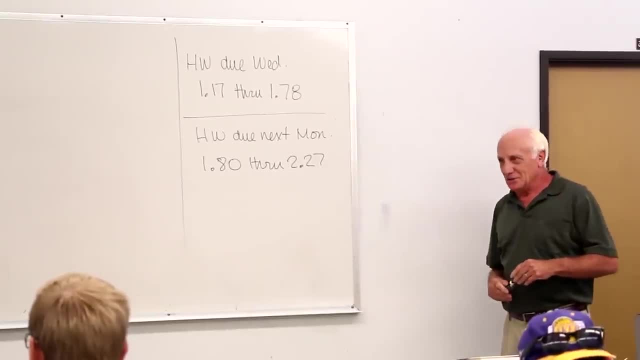 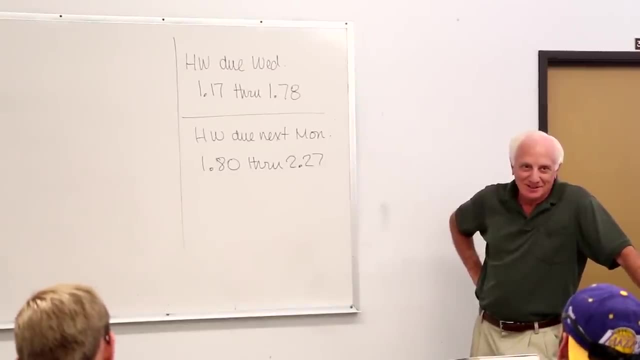 in the portal. okay, These aren't stale slugs. A slug is a unit of mass. How big is it? Anybody know how many pounds of mass are in a slug? That's a gravitational acceleration. in English, 32.2, right. There you go: 32.2 pounds mass in one slug. That means a slug is more massive than a pound mass. A slug is more massive. Okay, so those are the two unit systems. When you work problem for homework or exams. 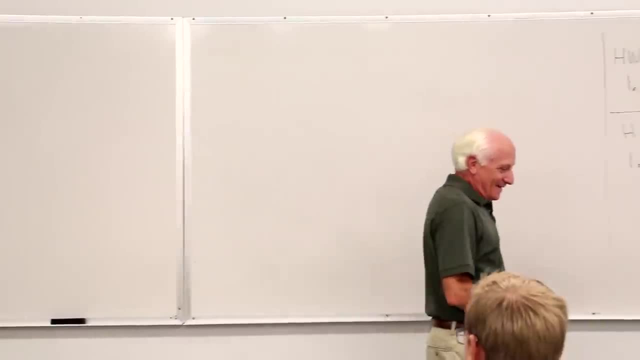 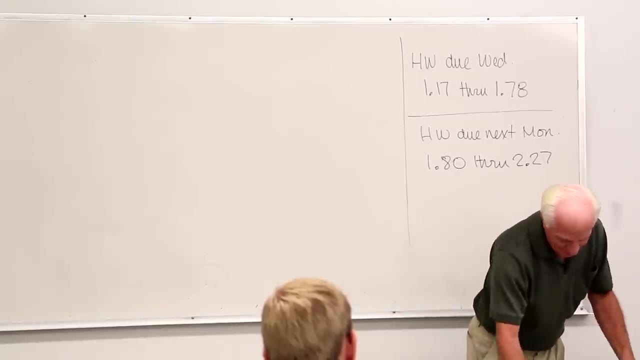 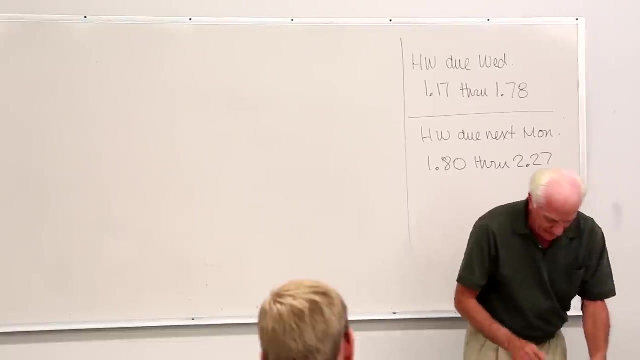 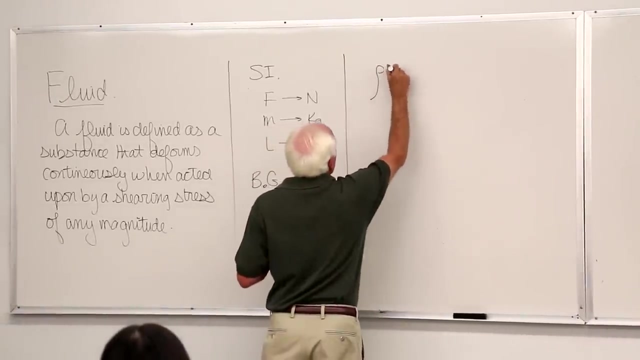 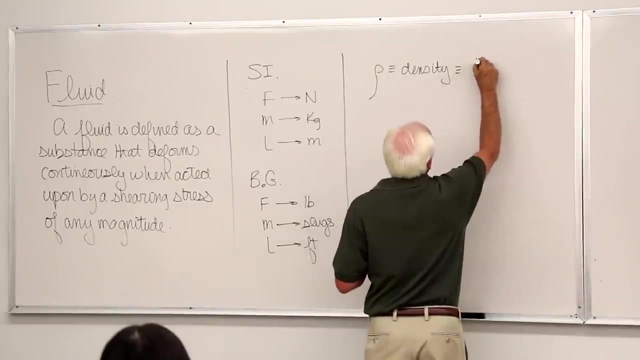 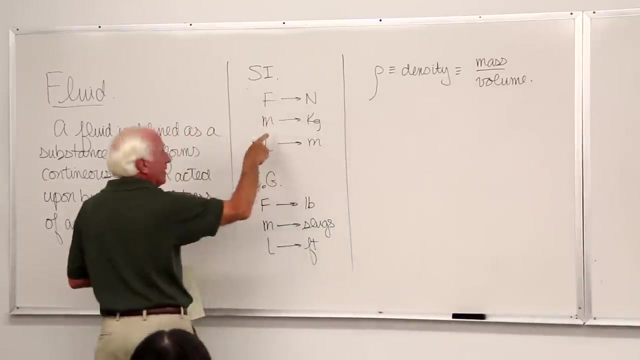 that's what you use there. Okay, Now let's take a look. Let's see pressure. let's look at some other. Oh yeah, Okay, If you've had physics or thermo rho density: density mass per volume, If it's in SI, kilograms per cubic meter, If it's in 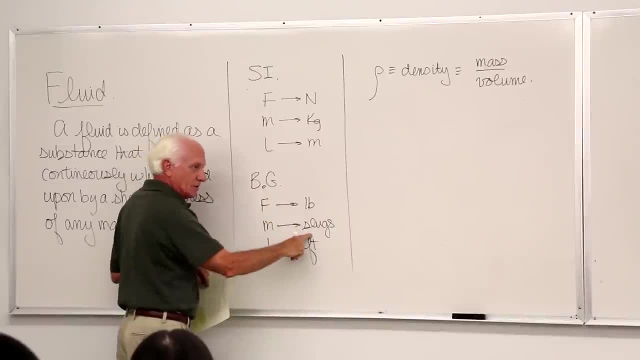 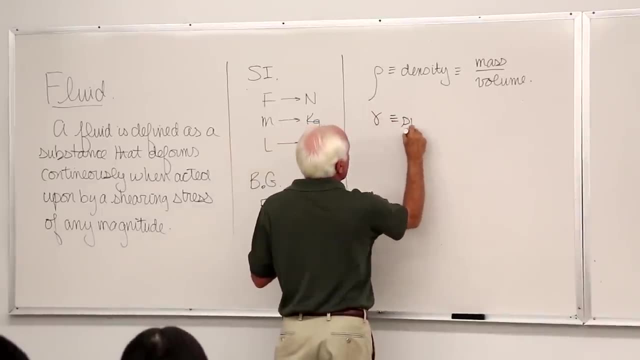 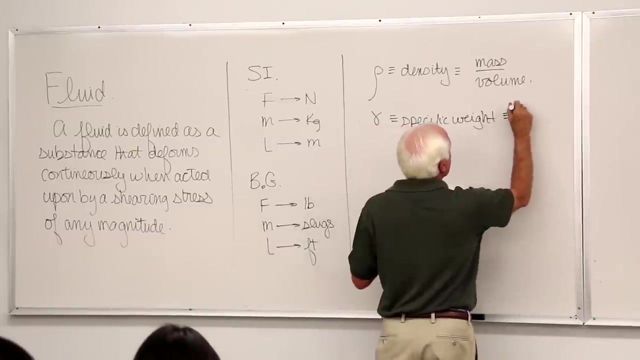 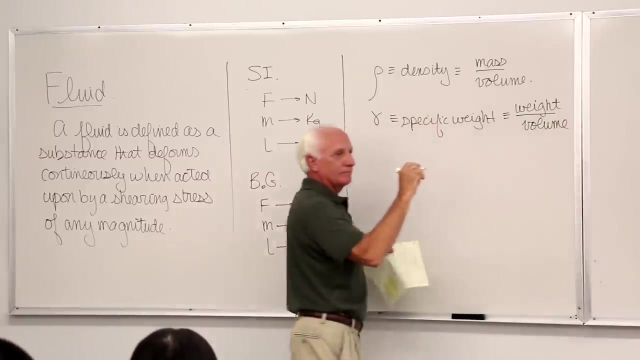 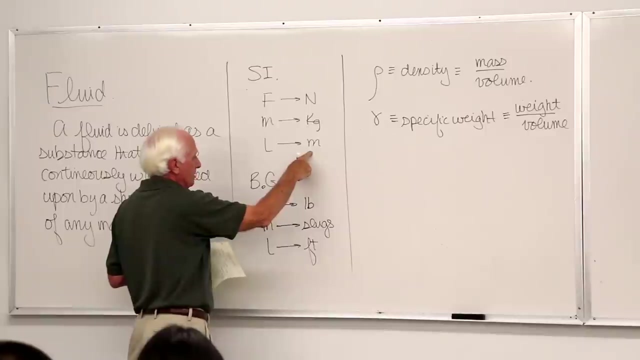 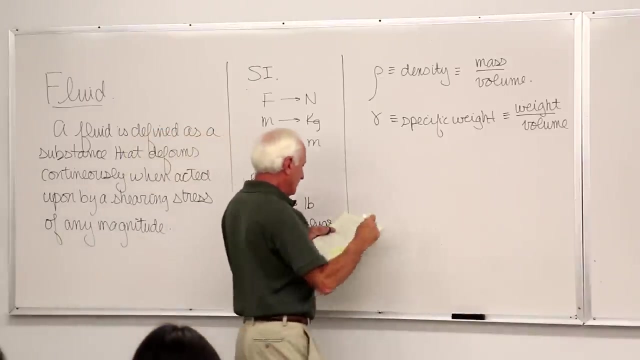 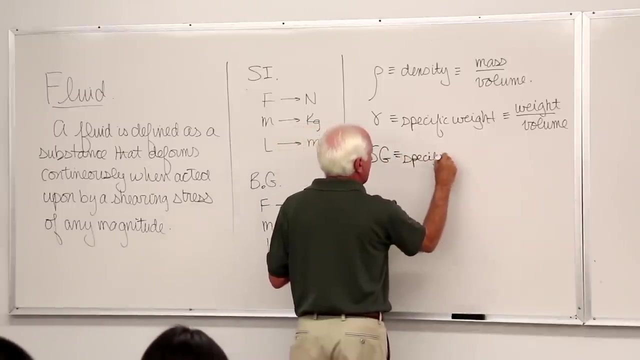 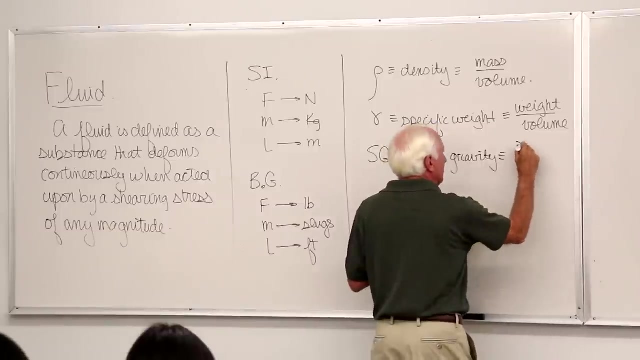 British gravitational mass: slugs per cubic foot. Specific weight gamma. Weight per volume: SI weight. weights of force: Newtons per cubic meter. British gravitational force: pounds per cubic foot. Specific gravity, Okay, gamma of the fluid in question under gamma of water at a certain temperature. 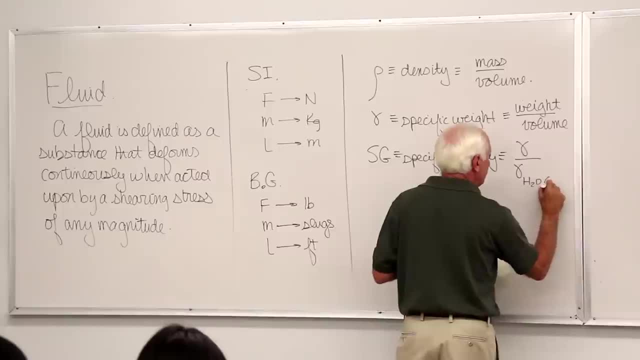 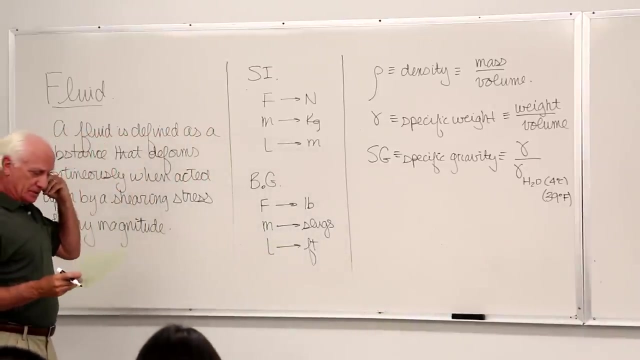 like I think it's 4 degrees, yeah, 4 degrees C, Or it's 39 degrees F, So it's a ratio. A ratio is dimensionless, So it's a dimensionless ratio. It's a dimensionless number. specific gravity Gamma is the specific weight of the fluid. 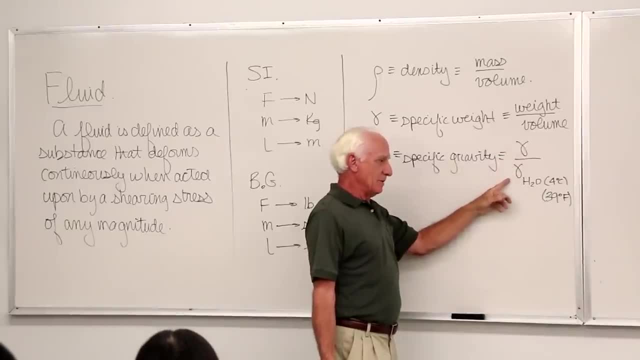 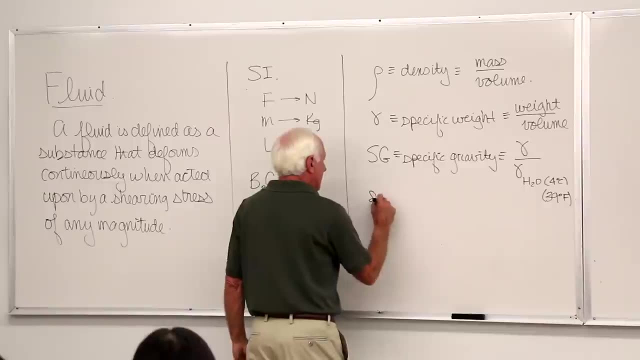 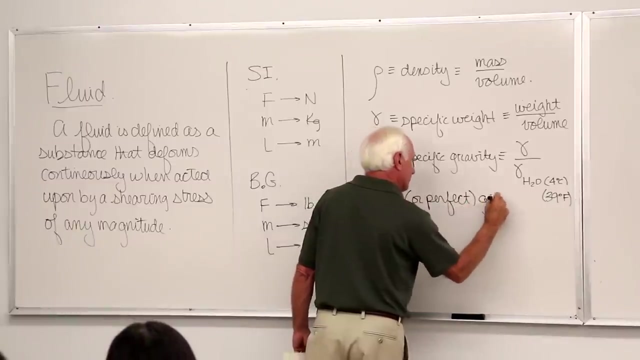 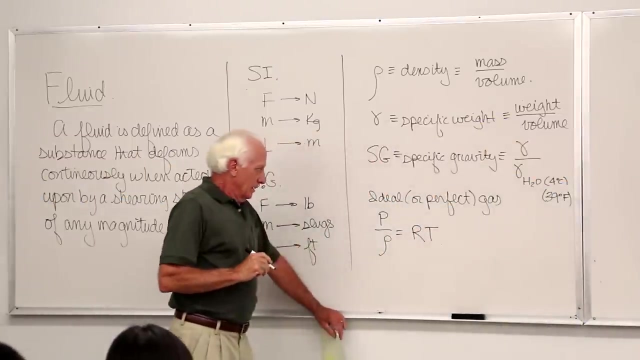 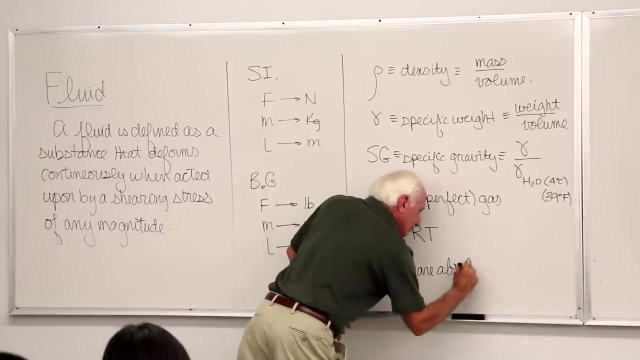 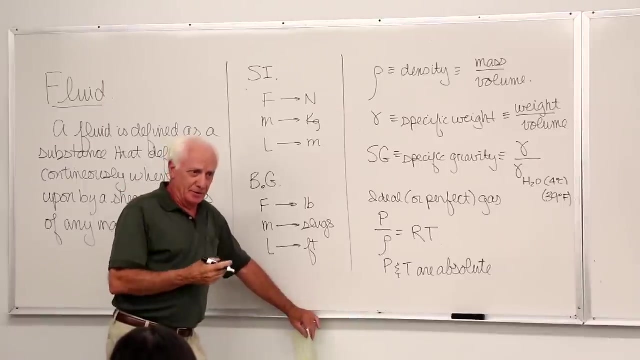 you're studying. divided by gamma of water at a certain temperature, An ideal gas or perfect gas- law P over rho equals R times T. P and T are absolute values, Absolute pressure, absolute temperature: We'll mention absolute pressure in just a little bit. You know absolute temperature. 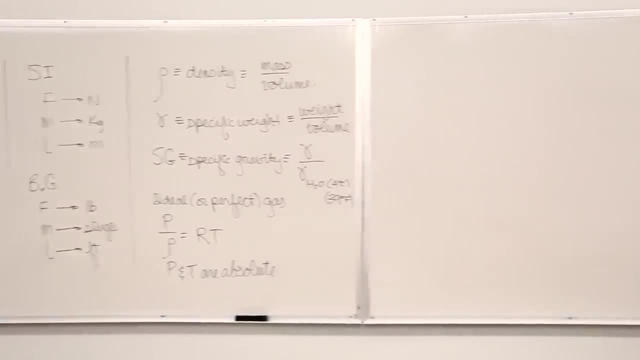 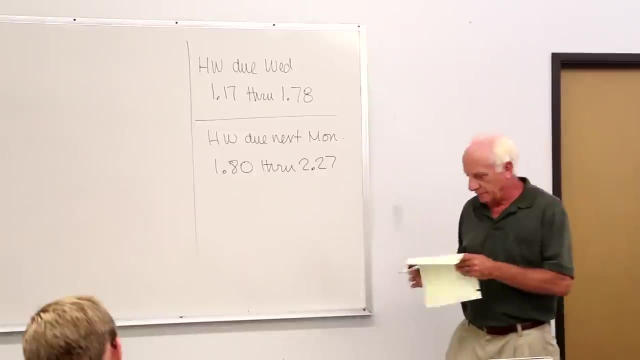 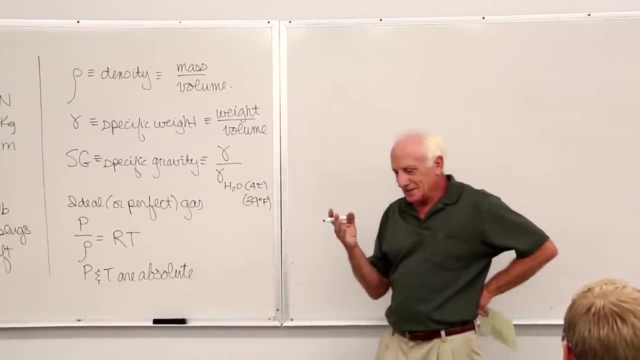 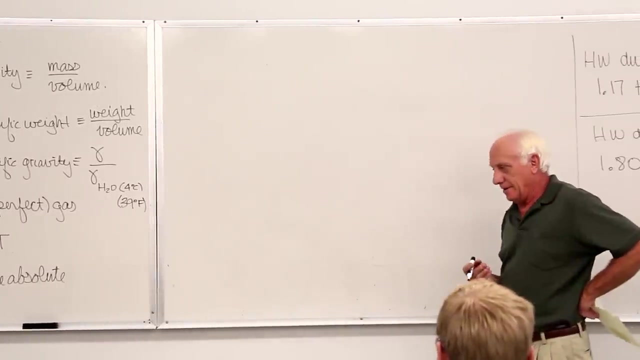 at 273 degrees C, degrees K, Add 460 degrees F to get degrees R. It's in the book. This is for gases. So the good news is, when we're studying this class, pretty much all the gases behave like that As long as you're around ambient conditions: air, hydrogen. 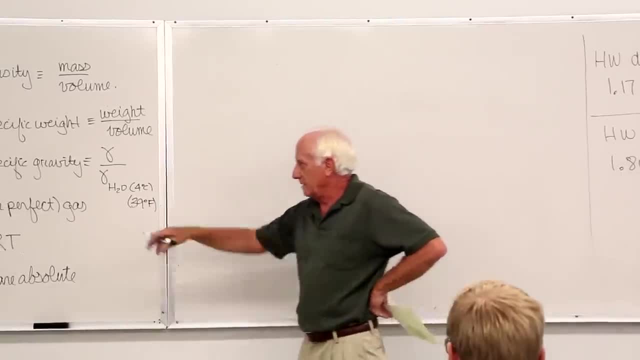 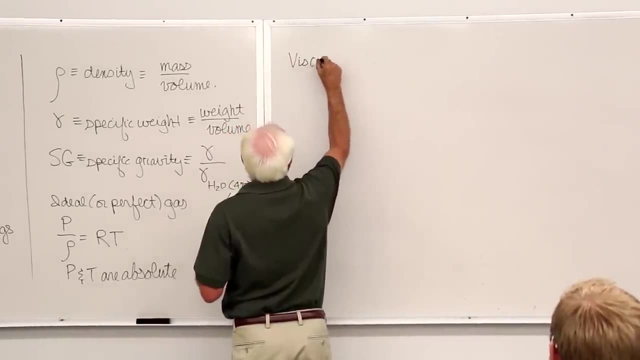 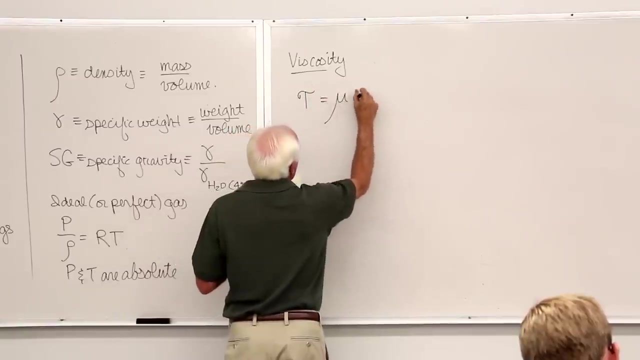 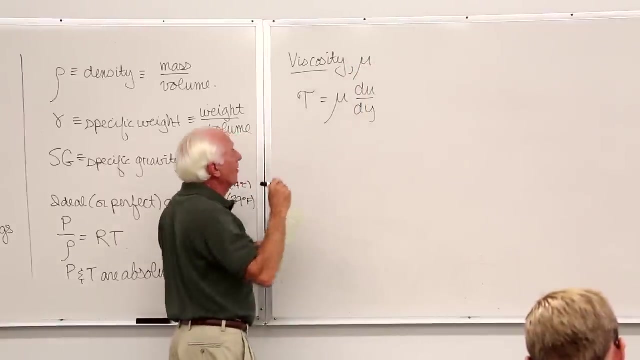 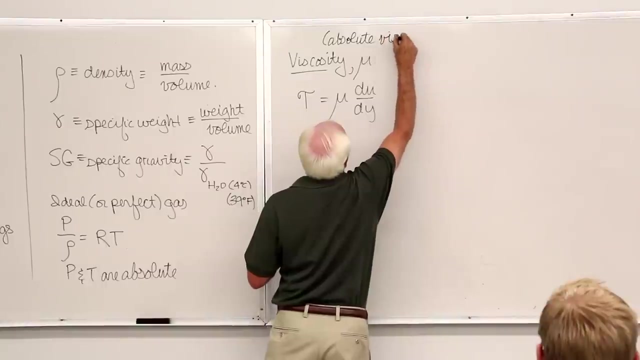 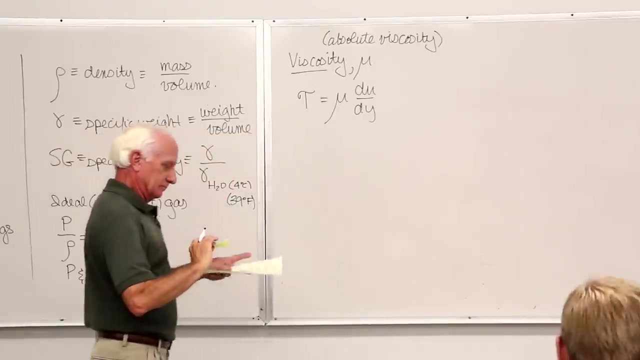 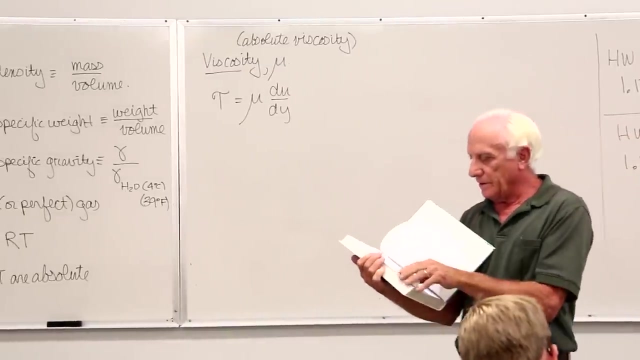 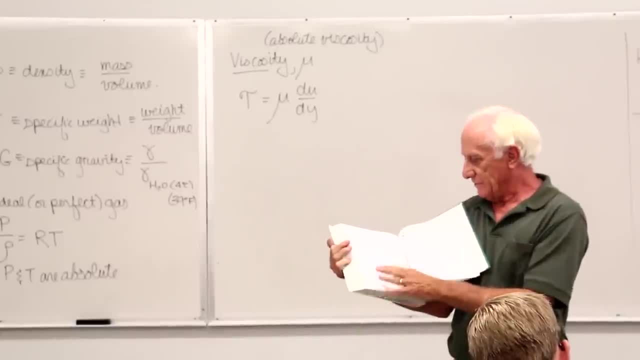 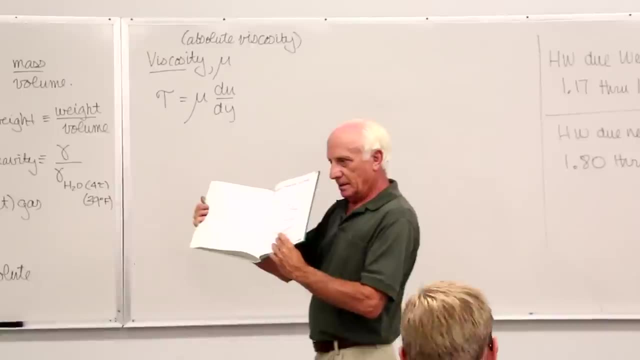 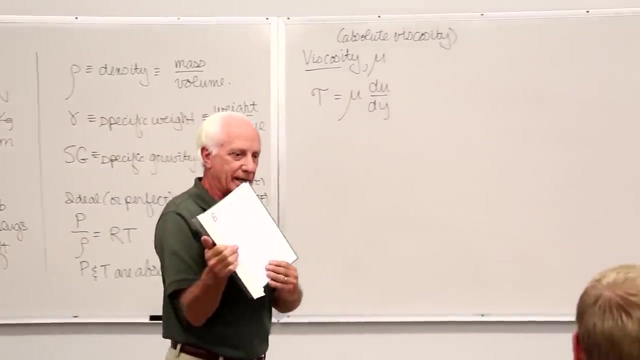 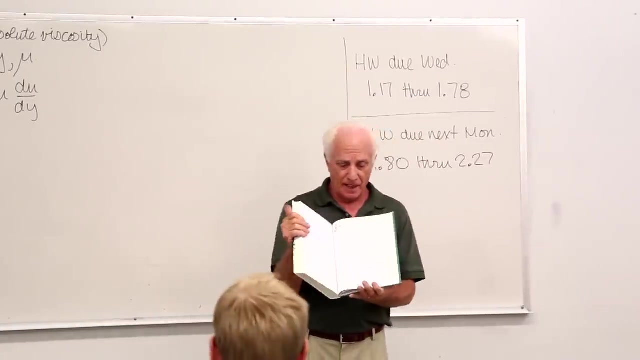 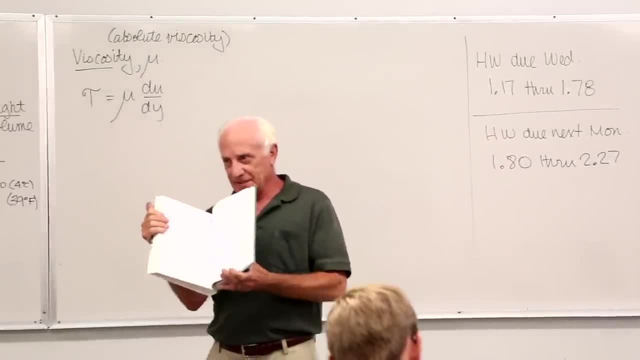 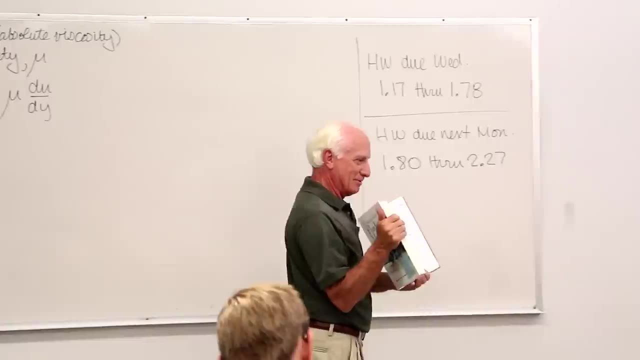 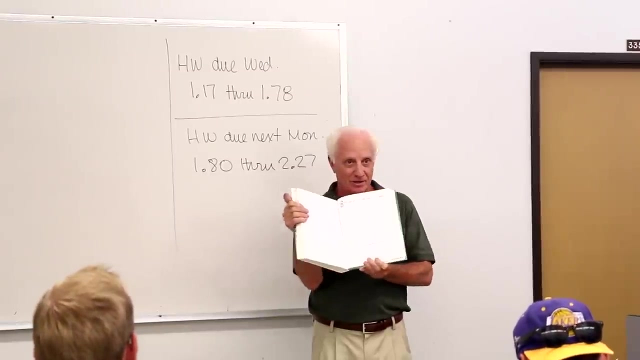 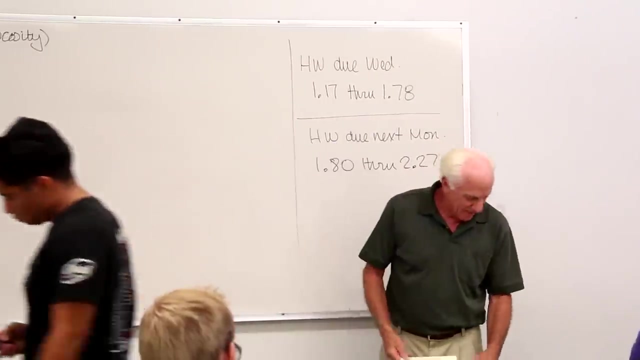 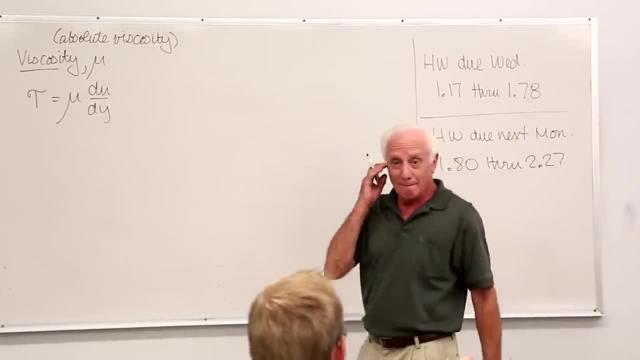 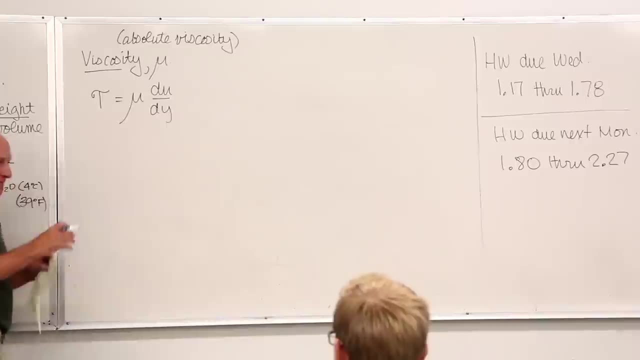 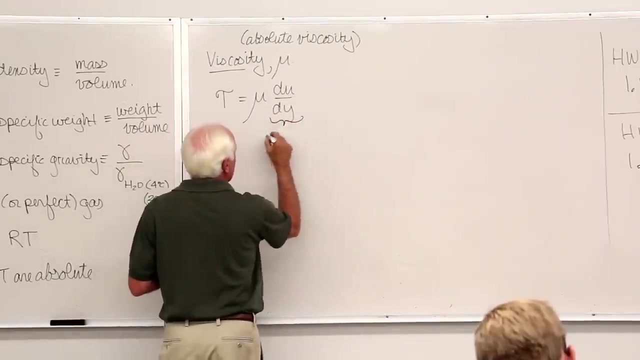 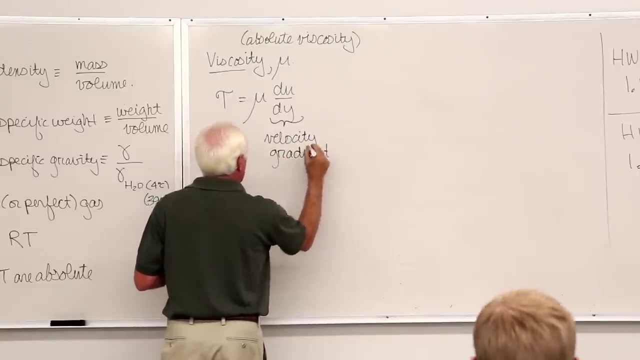 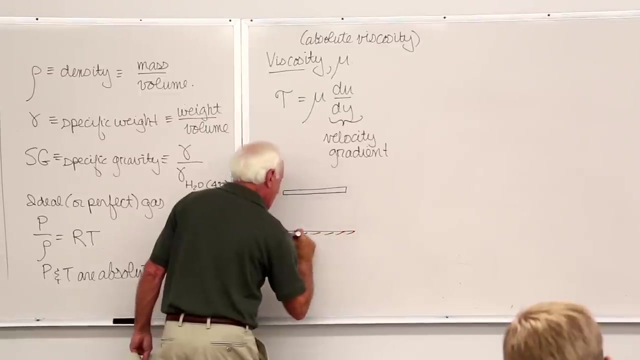 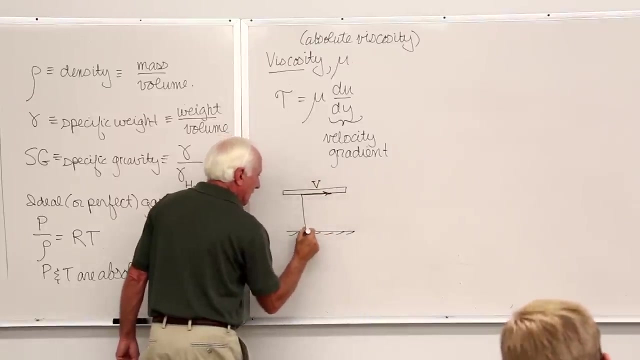 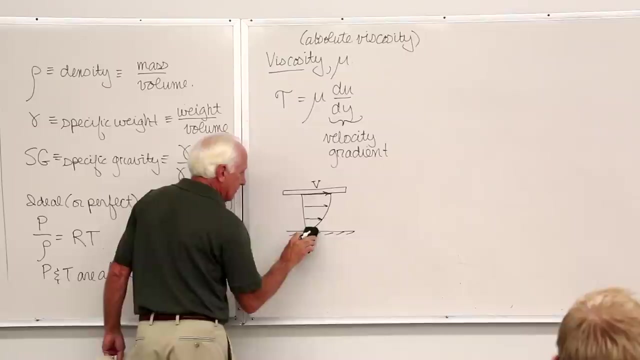 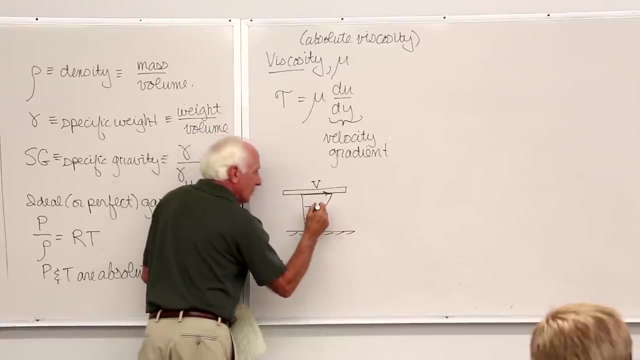 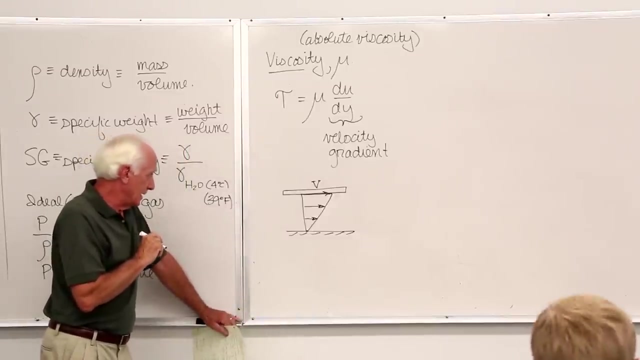 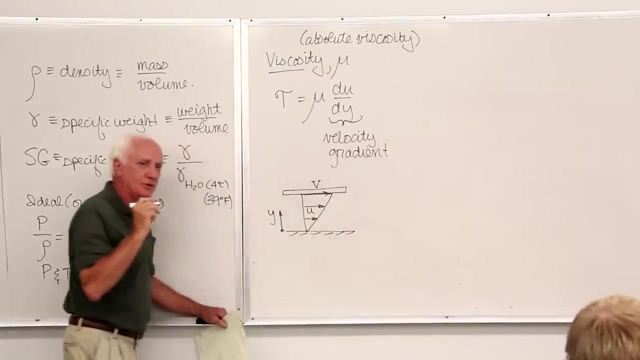 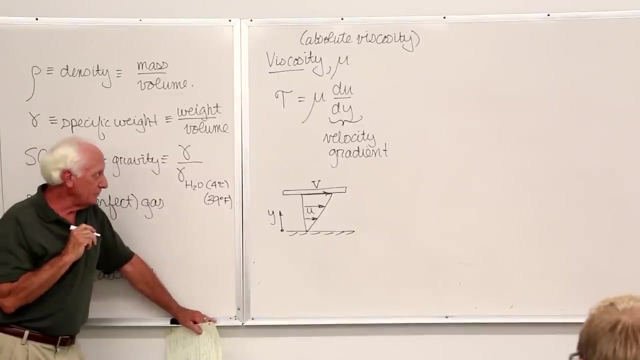 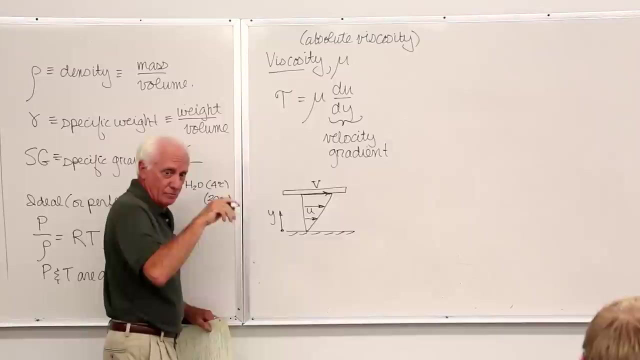 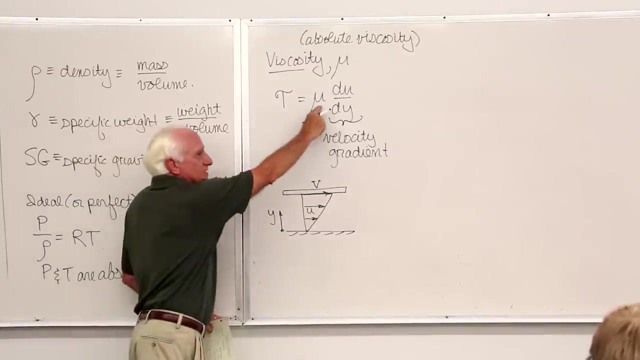 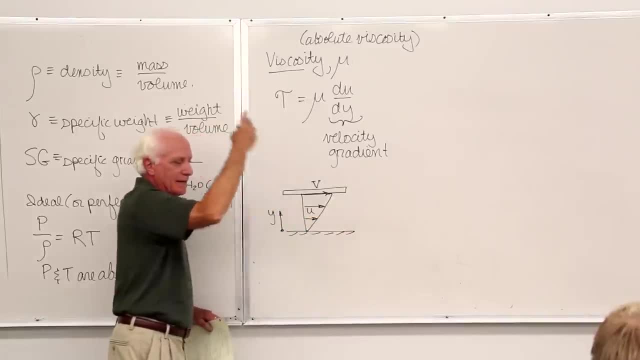 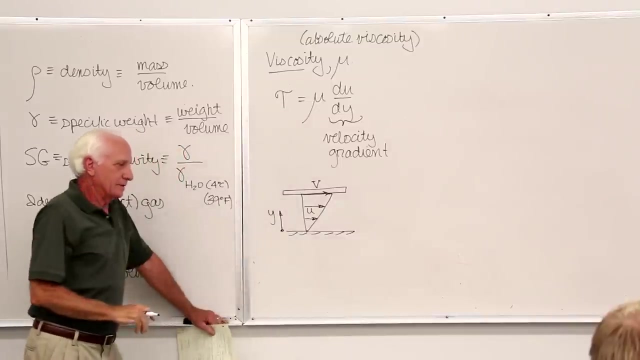 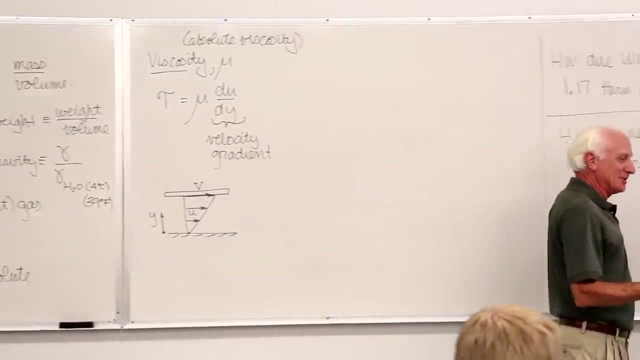 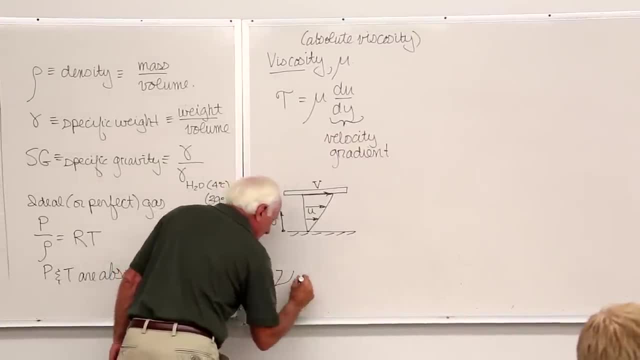 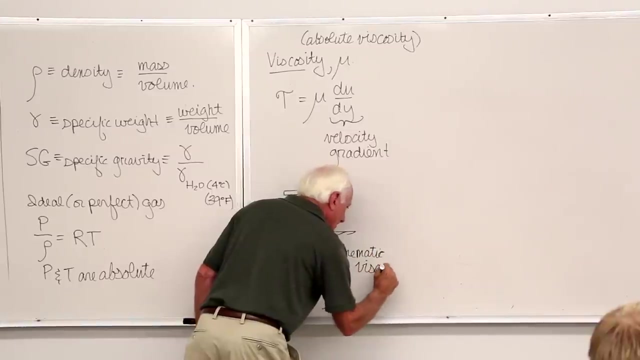 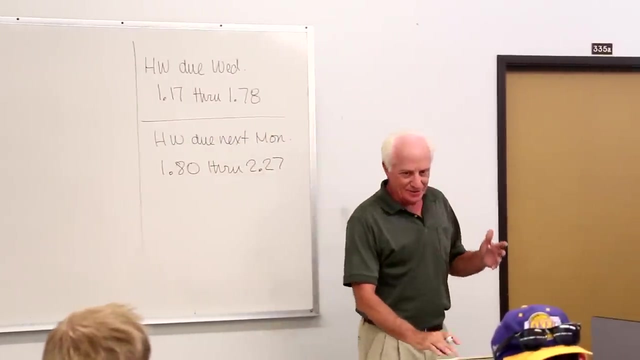 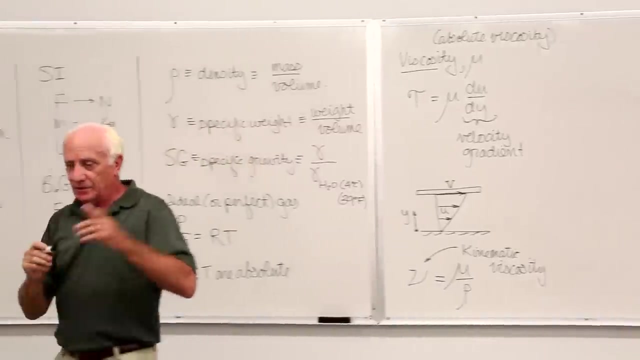 property which is mu over rho. This is called kinematic viscosity. So there are two possible viscosities. One is a real thing. The real thing is this up here. This is really the viscosity. If someone just says viscosity to you, then you 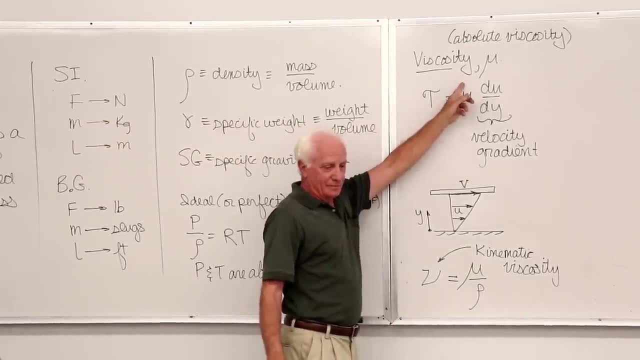 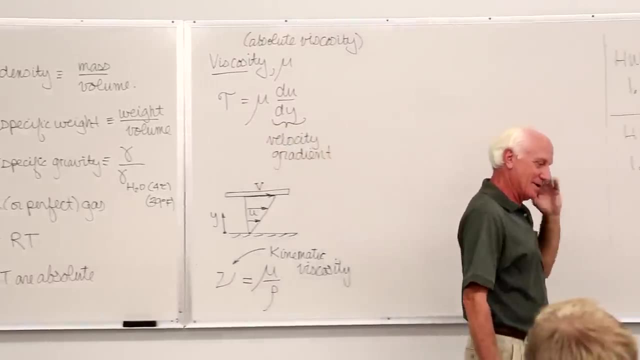 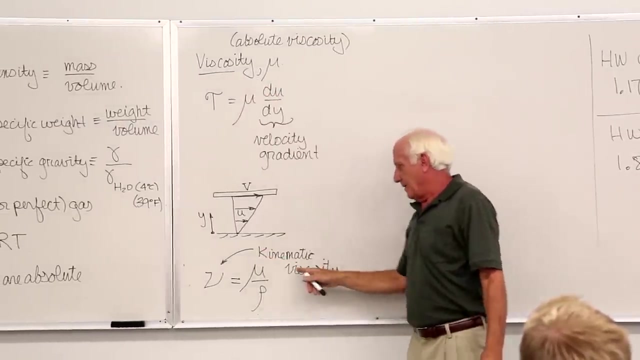 assume they mean this one, But that's why they're also called absolute and kinematic, just to be certain that someone knows what you're giving them. If you say viscosity, though, the default definition is here: Kinematic viscosity is this value divided by the density growth. This thing comes in handy. we'll see. 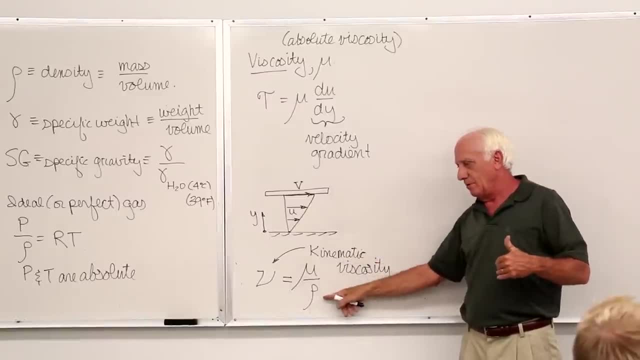 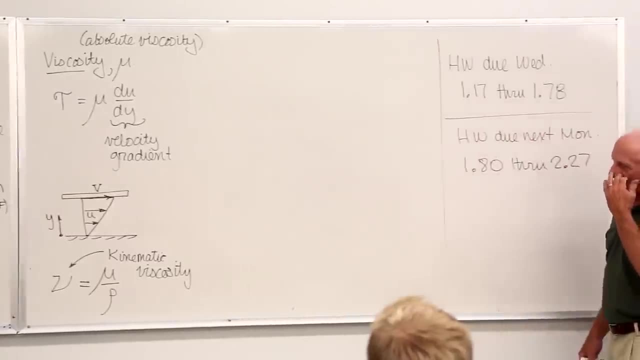 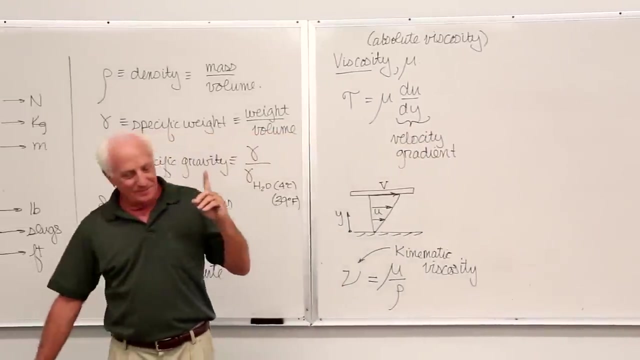 later on in some equations, When it appears the ratio mu divided by rho appears in some equations, So it's given a special name called the kinematic viscosity. Okay, the units, Oh the units. Okay, if you don't memorize those things, and I hate to if you don't- 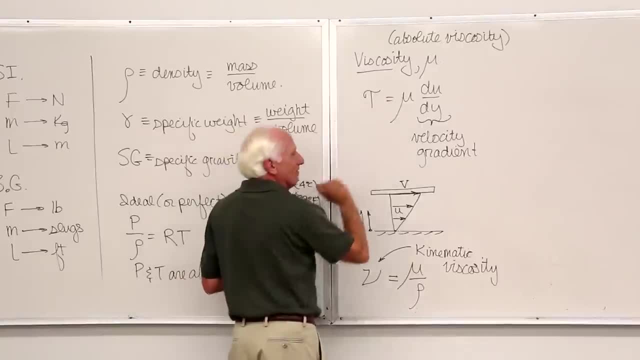 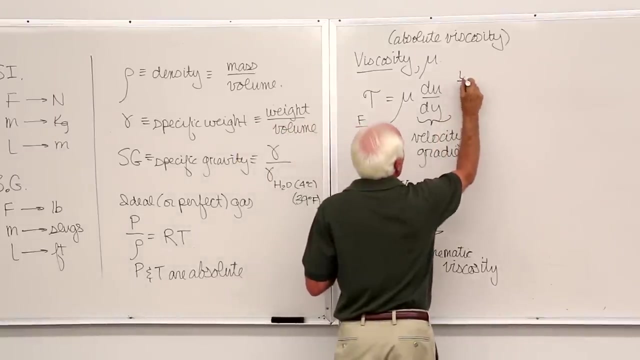 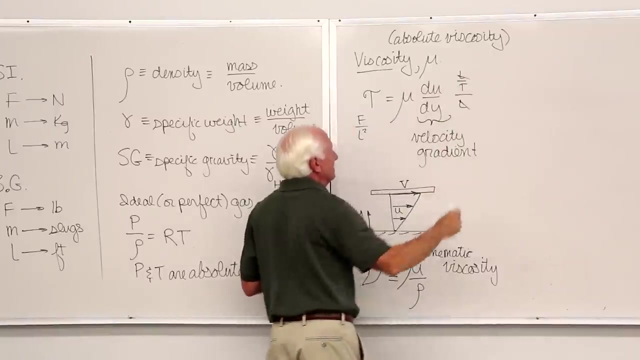 memorize them, then figure out what they are. What is this guy? Force divided by area: Okay, so force divided by area, The area, Let's just say length, squared. What's this guy? Velocity, Length over time: What's this guy? Length, Okay, Cancel, cancel. So figure out that mu is F. 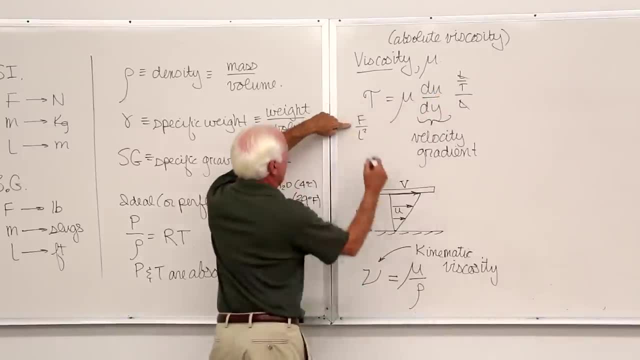 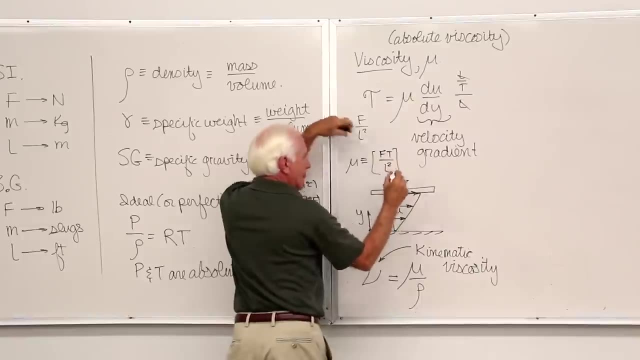 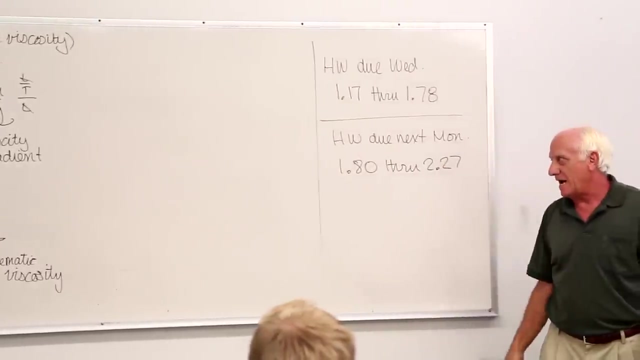 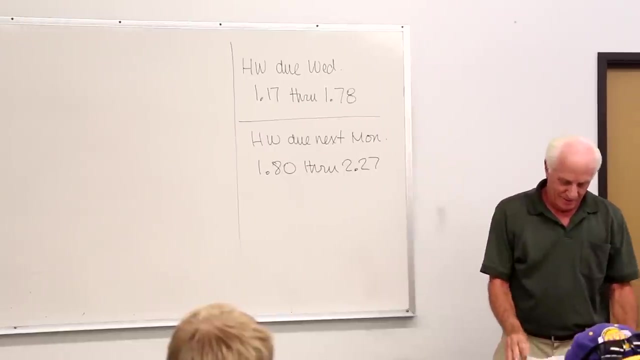 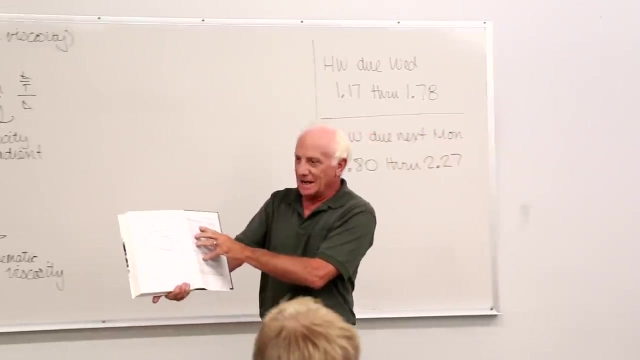 This guy's a denominator. This guy's a denominator. Put him up here, FT over L squared. If it's nu kinematic viscosity, divide that guy by mass divided by length: cubed. Density Mass divided by length, cubed. We go back here. Viscosity, English units. 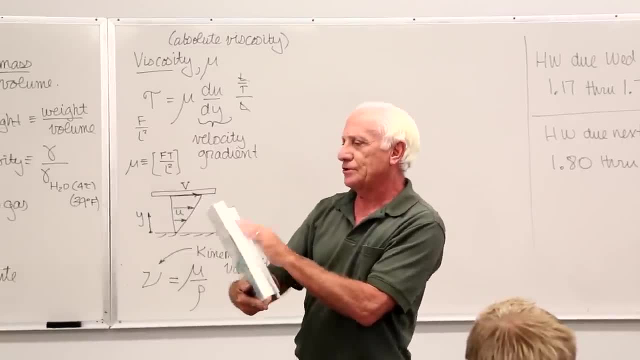 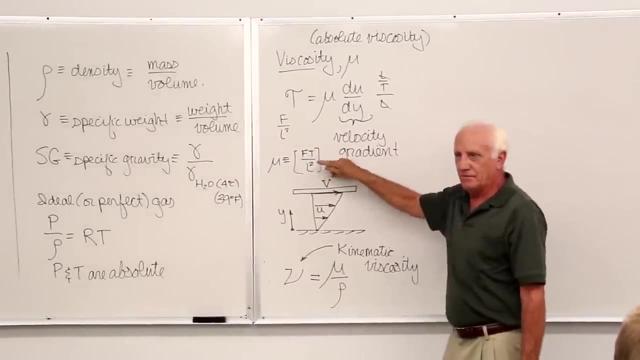 What are they? Pound second per foot, squared. Look at it. Pound second per foot, squared. Pound Over there. Pound second per foot, squared. Yeah, I don't memorize that stuff. I derive when I have to, When I have to. So there's no. 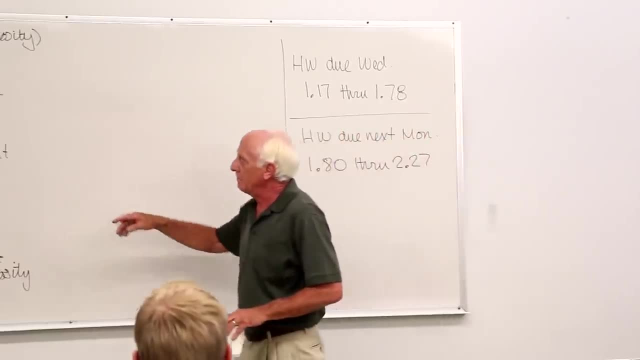 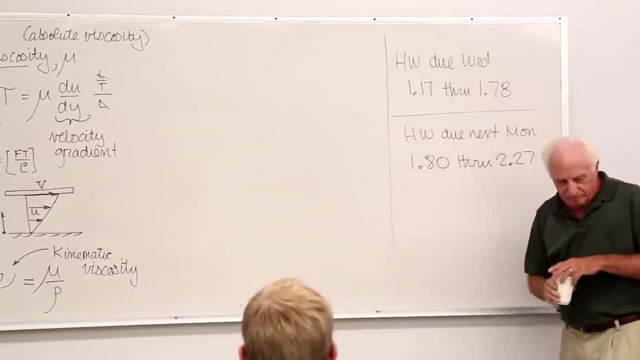 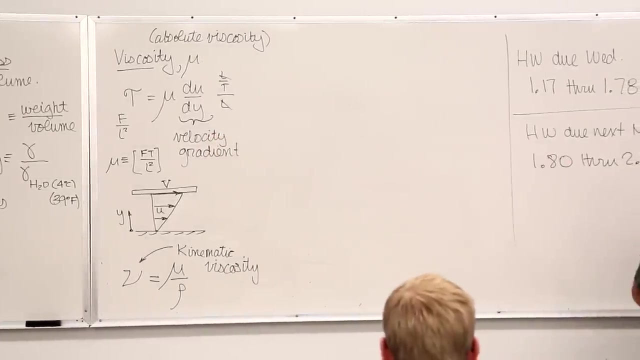 reason to memorize it? because you know you can derive it. Where does it come from? The basic governing equation? right there. Okay, Now let's go on to our next two properties, The next one, By the way, before we forget. let's just go. 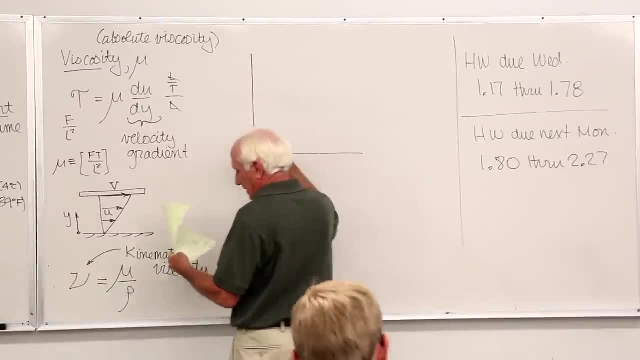 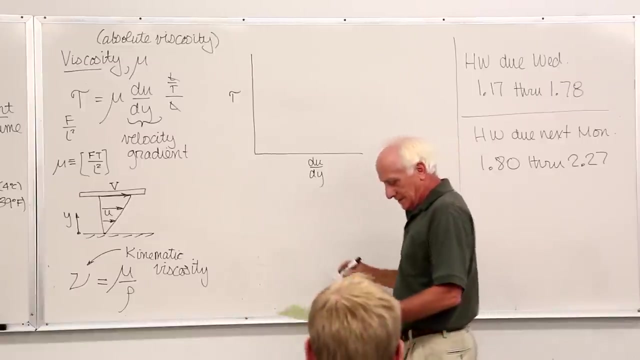 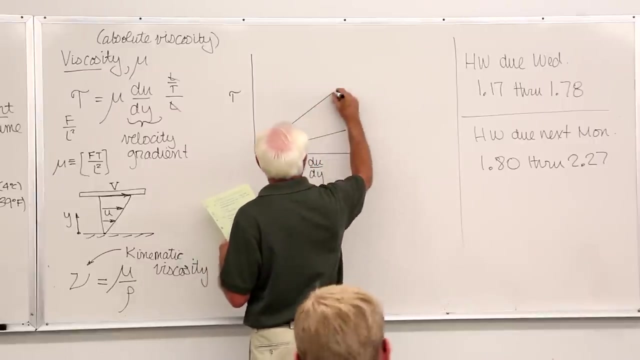 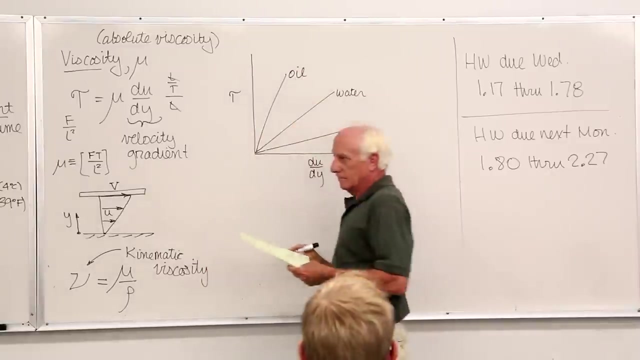 ahead and put this graph up here. This is Shearing stress. tau there. This is g and dy velocity gradient, Sometimes called the rate of Shearing strain. but the velocity gradient is sufficient. If this is air, this is water, this is oil. Oh yeah, We know, Intuitively, we know. 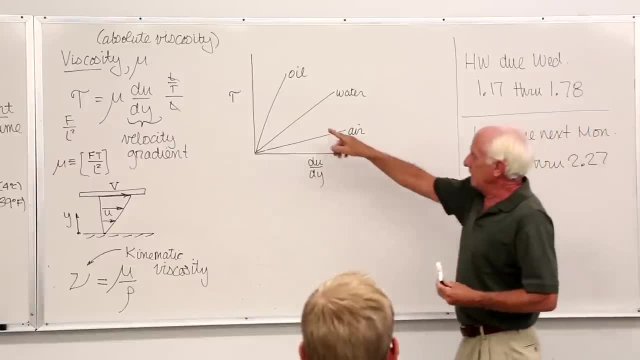 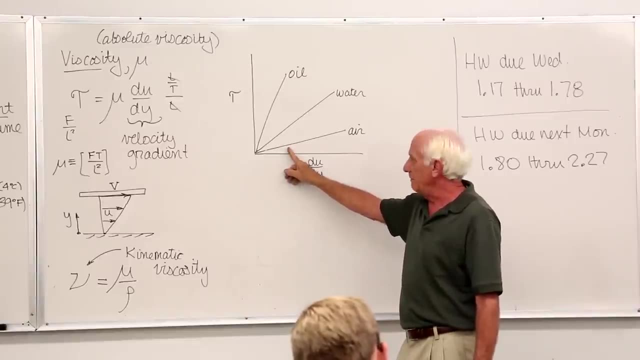 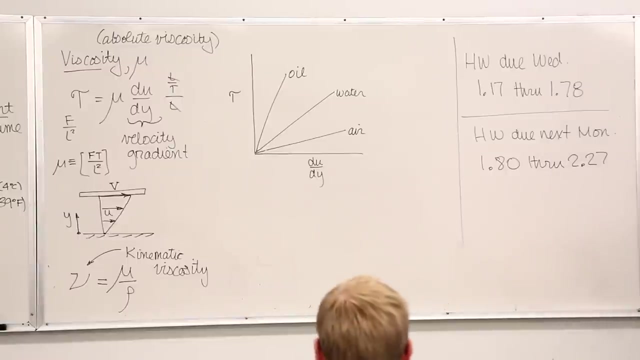 oil is very viscous, It will give you very high Shearing stress for a certain value, du dy. Given a value of du dy, air is not very viscous. Water is in the middle of the road. Oils are very viscous, Notice. they're linear too, which is very important. 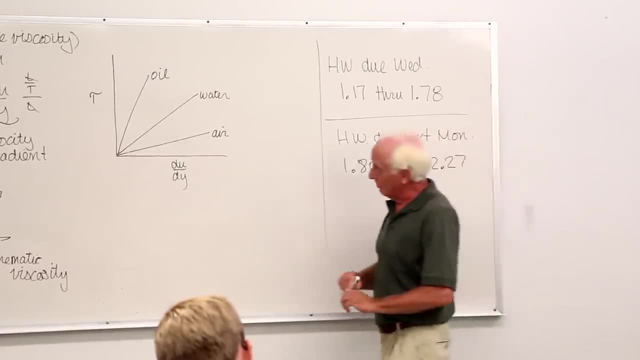 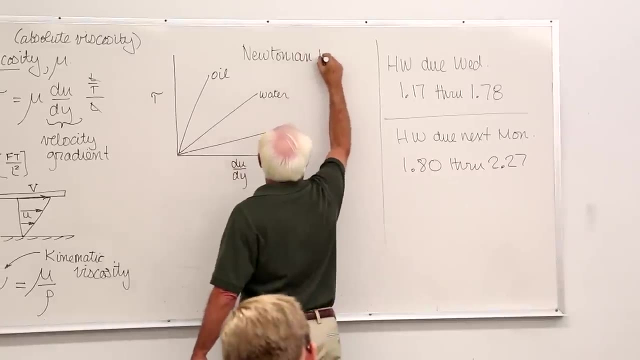 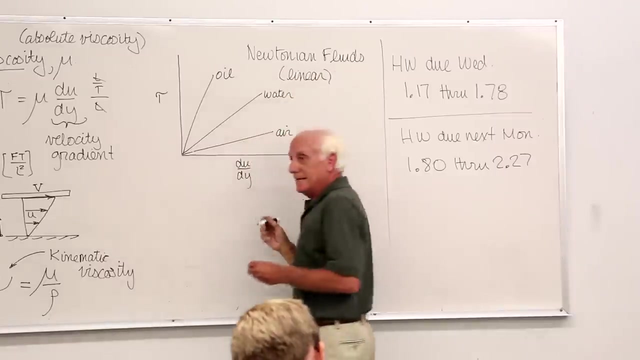 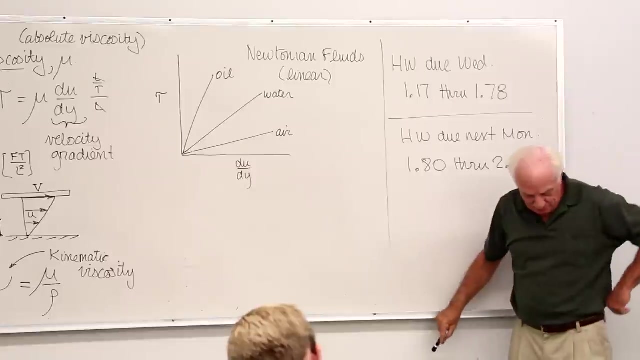 They're linear. Those, those tools are called Newtonian. There are many which are not linear, which we know. Think of a common study in ME 311, examples: Toothpaste- no, it's not Newtonian. Latex paint. 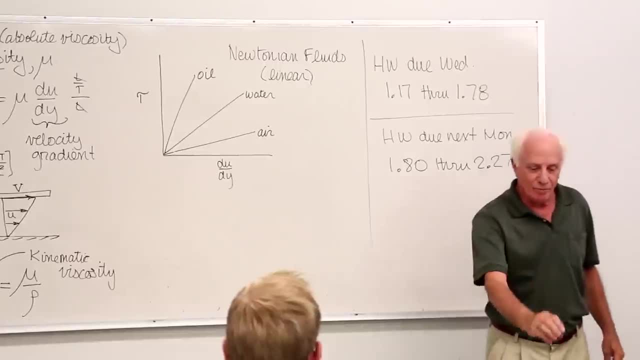 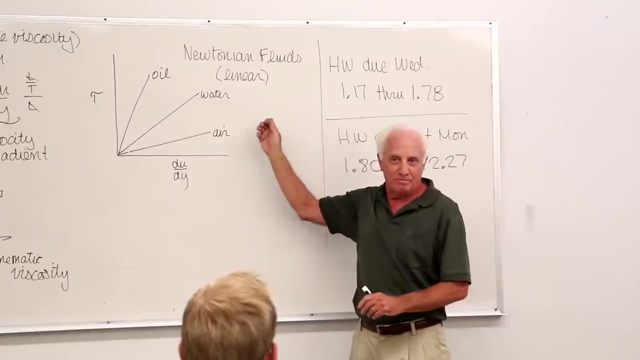 no, it's not. When you put that paint on a brush, put that brush in water, pull it out of there. all of the water just runs off. You'd be running to the wall to get up on the wall before it ran off your paint brush. No, no. 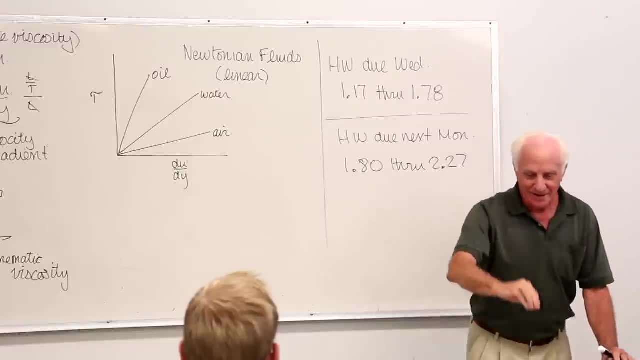 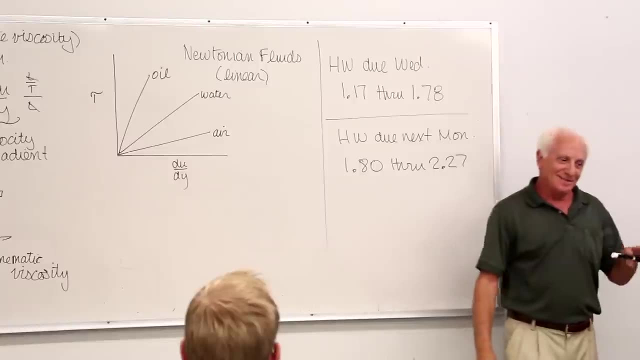 You put that in there in latex paint, take it out of there, kind of turn the brush. it stays fibers until you get to the wall. Then you either roll it on or you paint it on. Yeah, it's different, It's not linear. It's not linear. The graphs are in the book, by the way. 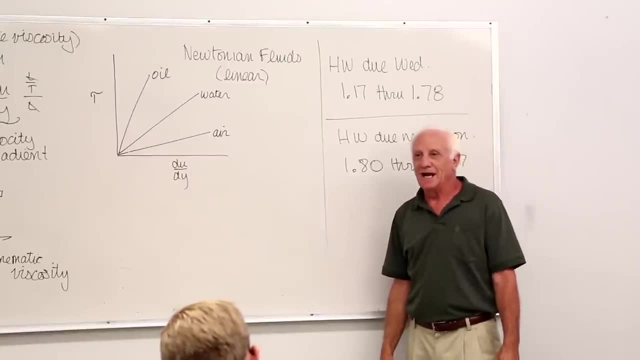 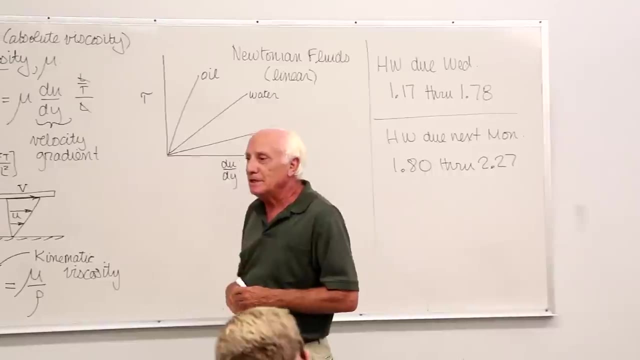 Crick sand, not linear. No, no, no, Crick sand. The more you try and get out, the harder it is for you. You've got to go really, really slowly. Don't try and pull your foot out, because you're. 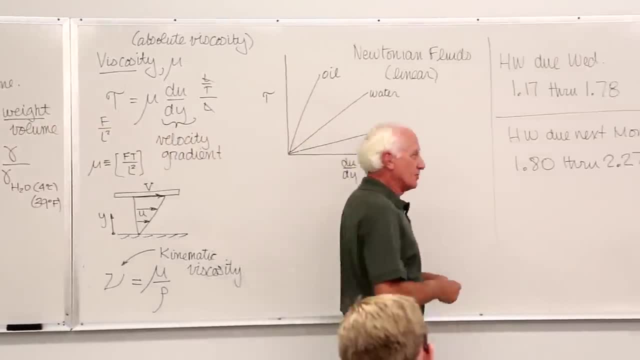 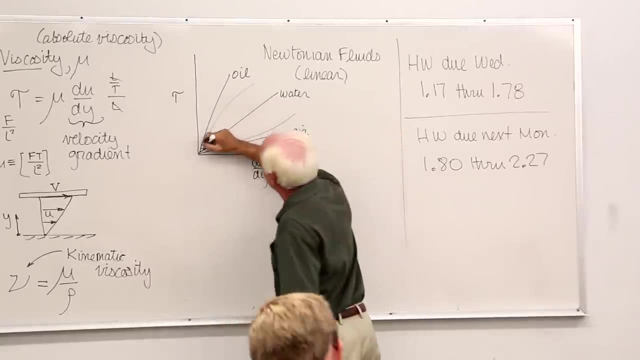 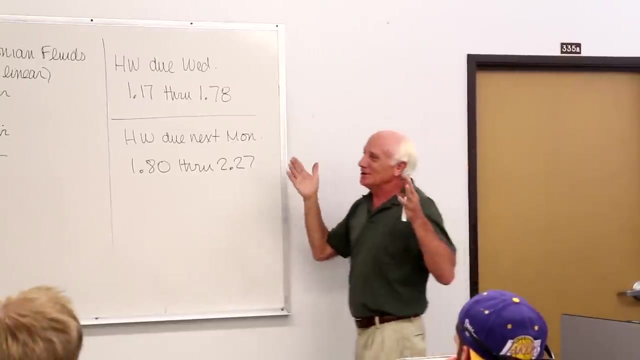 going deeper. It's all. this graph tells the whole story. I'll just show you a couple. Some go like this, Some go like that. Here's crick sand, Here's latex paint, There's toothpaste, Maybe stuff like that. That's just for your own sidelight, right now, What you're worried about. 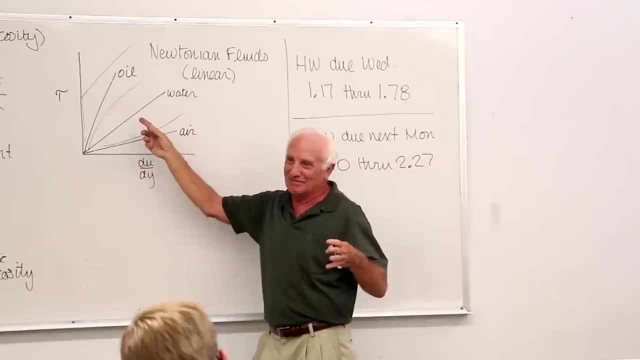 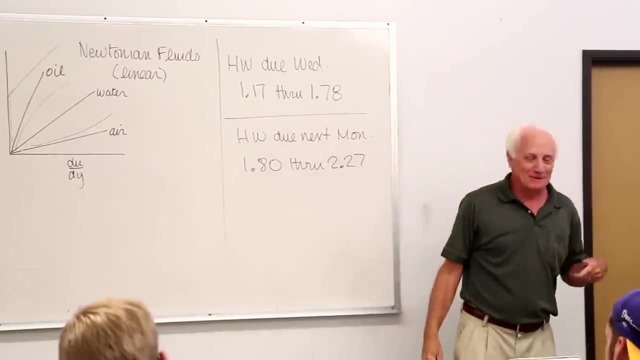 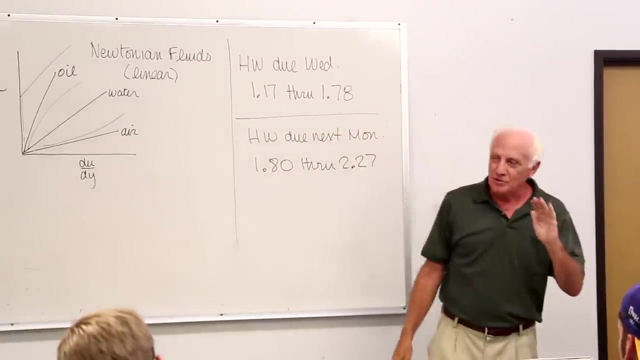 are the three things us MEs and CEs look at most in life: Arrows and MEs, arrows and CEs mostly MEs, engines and things like that. We're not going to worry about those other exotic ones, We're going to worry about things like these three right here. They're all going to be Newtonian. 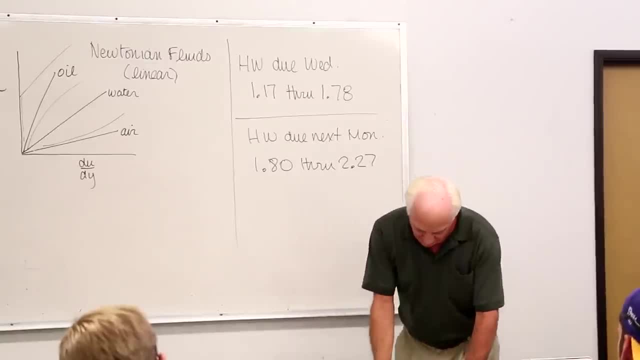 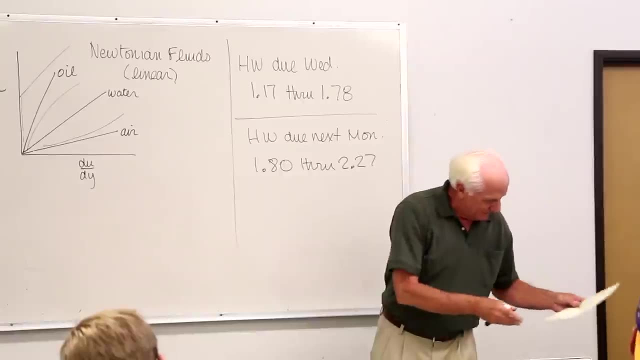 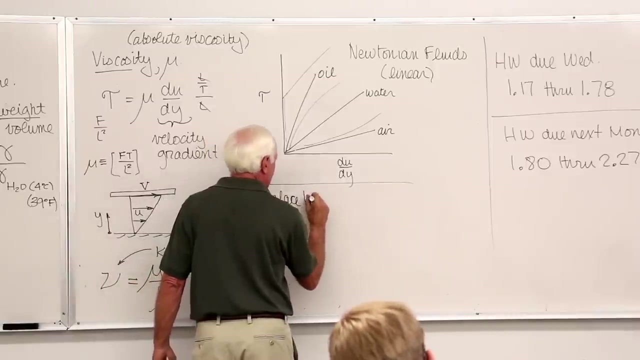 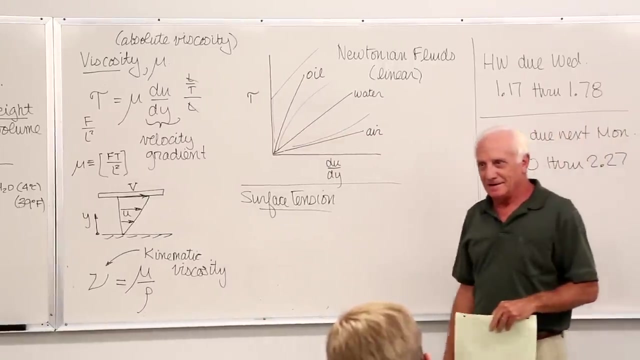 Newtonian fluids in ME 311.. Okay, Let's go to one more. Let's see, Here we go: Surface tension. Before I forget, of course we're being videotaped by our friend here, Matt, Matt, you're an. 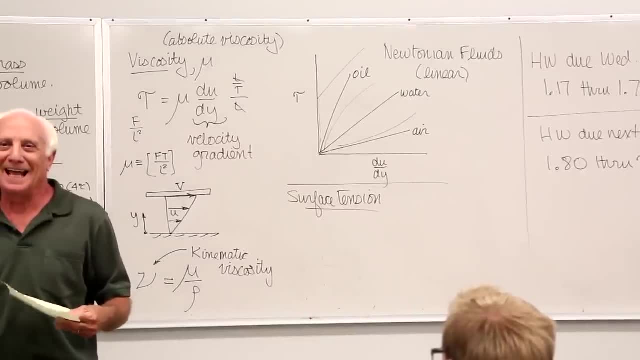 ME student. right, What year are you in? A lot, Did you start here? Did you start here? Yeah, I started here, Oh, did you? Okay, Okay, But you're taking senior classes now, right? Yes, 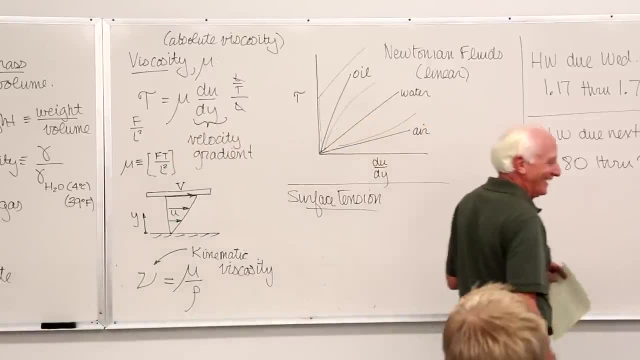 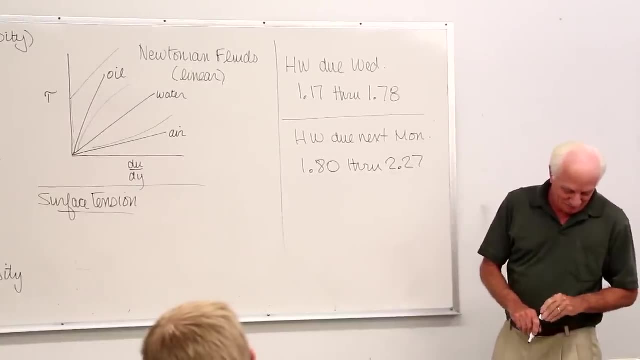 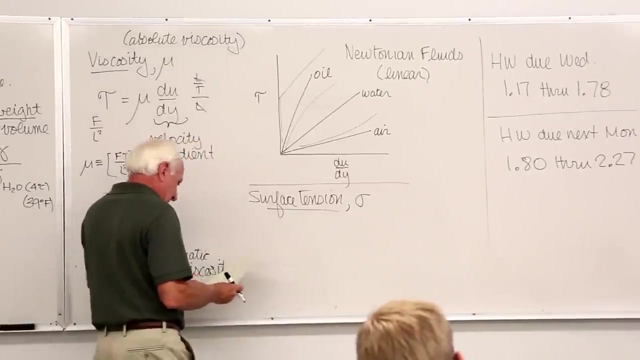 Oh, good for you. So it's close. Yeah, very close. It should be my last quarter. Okay, good, So he'll be at every class meeting videotaping the lectures here. Okay, surface tension. The symbol for that is sigma. Sigma is. 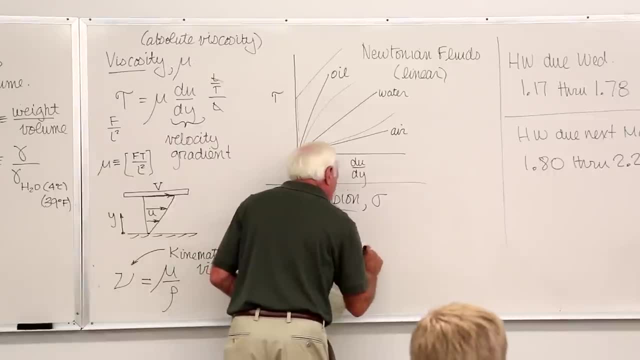 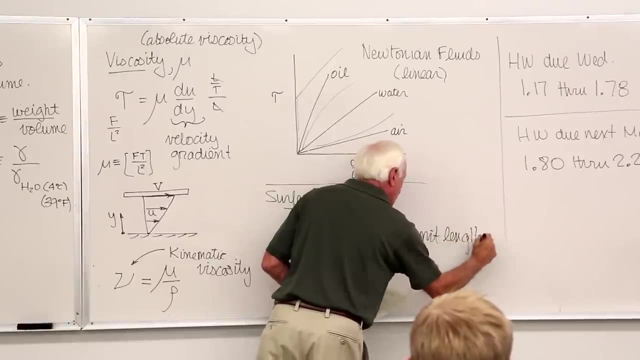 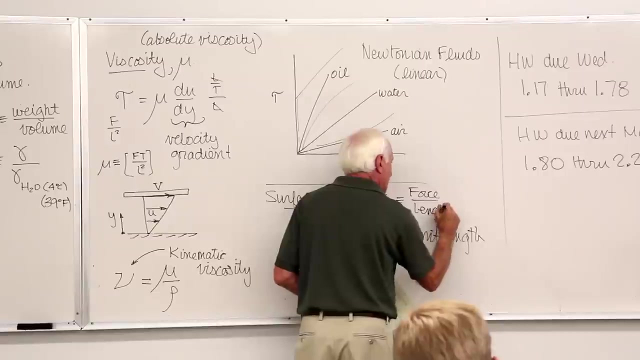 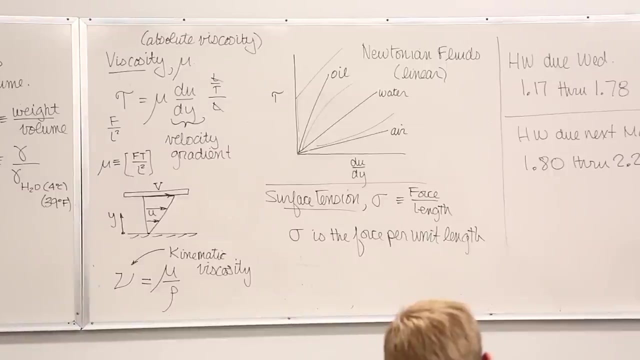 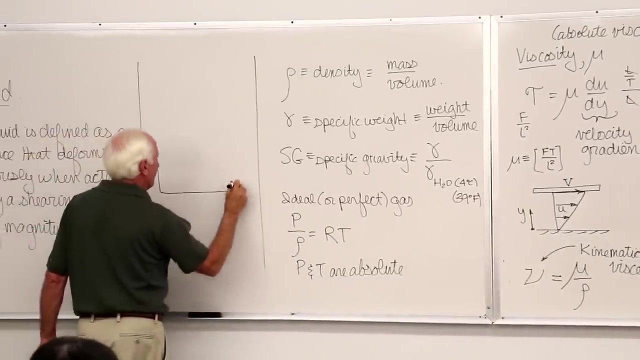 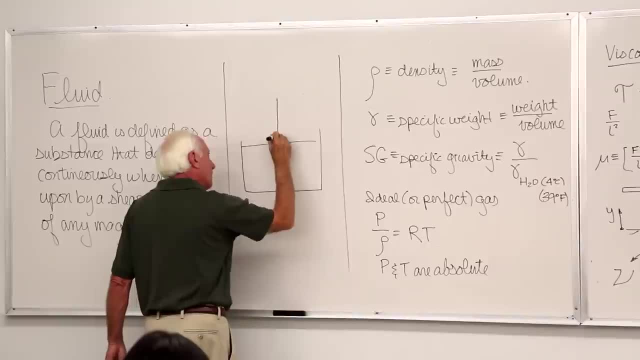 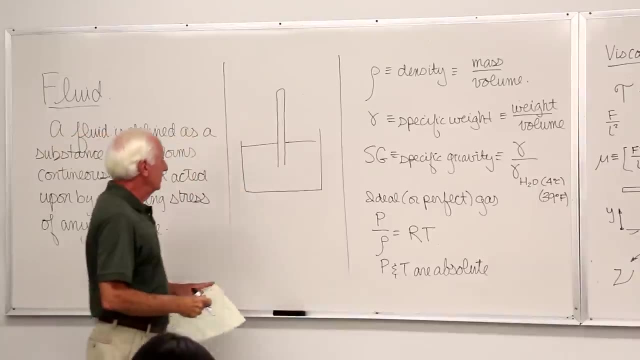 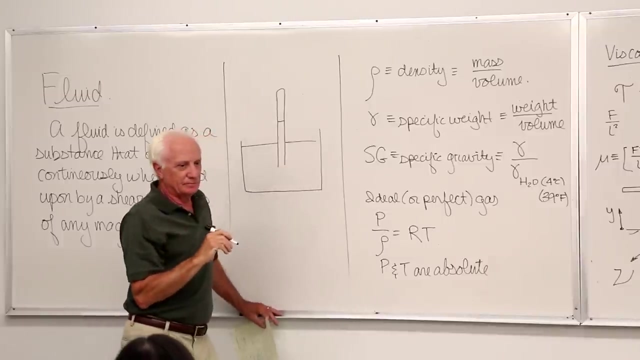 Okay, Okay, Okay. Here's a reservoir. I put this tube in there, invert it. The liquid will rise up in that reservoir. something like this: You might have seen a Mercury barometer on the wall And the Mercury rises up that glass tube to read off what the Mercury level is. 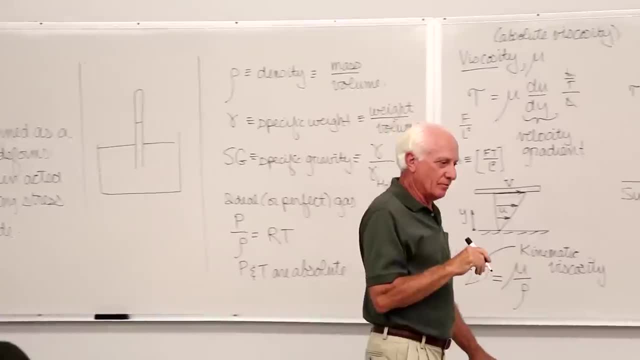 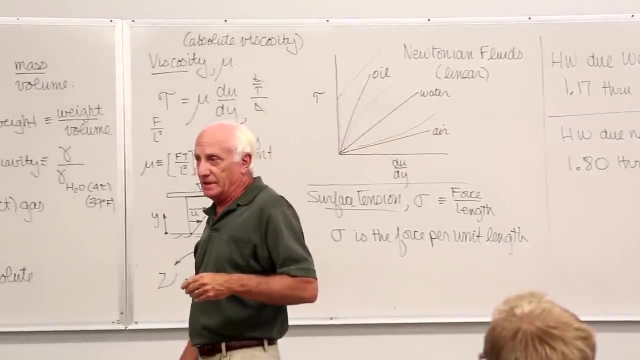 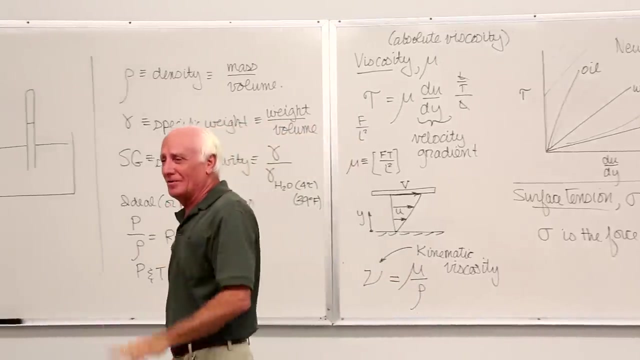 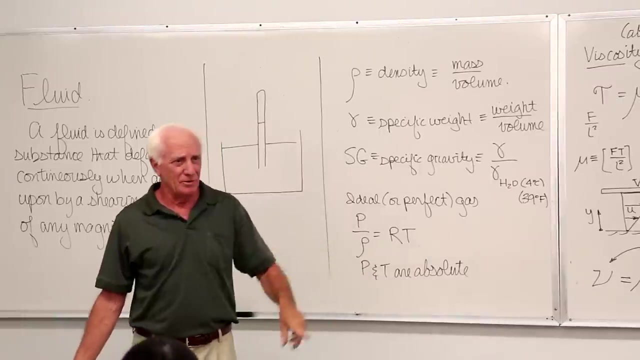 The guy at night in the news says: okay, the weather forecast, a cold front's coming on from Canada and the barometer's dropping, and it's right now 30.05 inches of mercury. You say, what do you mean? there's mercury dropping out of the sky on people's heads. No, no. now ask any of your friends at night, say to them what does he mean when he says the pressure is 30 inches of mercury? 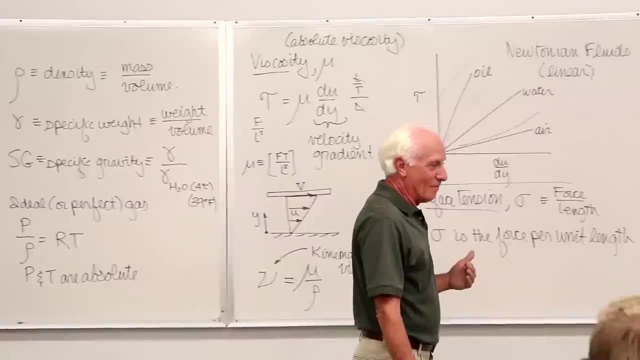 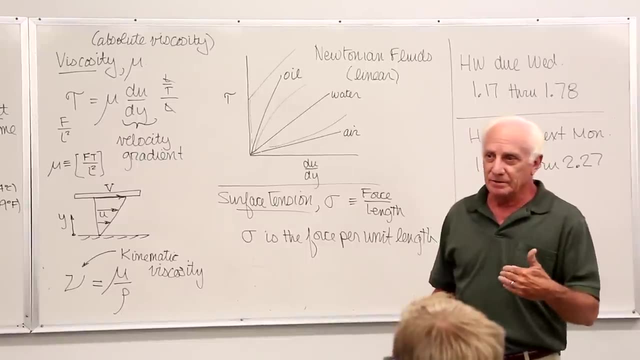 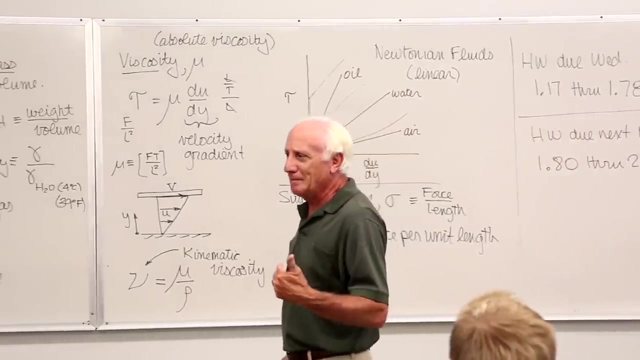 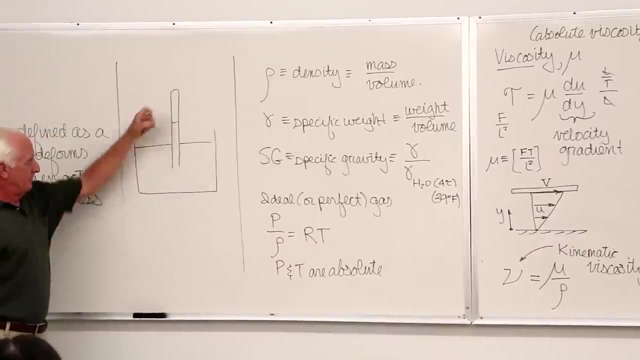 Most folks don't have the slightest, of course. They don't ask them their tire pressure. don't tell you 32 pounds in my tires. Do they really mean 32 pounds of air into your tire? No, no, they're taking shortcuts. They mean to say 32 psi in my tire. Well, if you put mercury in here, fill the tube with mercury, invert it, come off. there the mercury rises up. 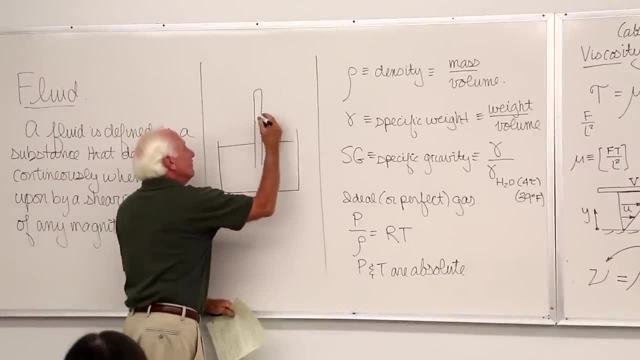 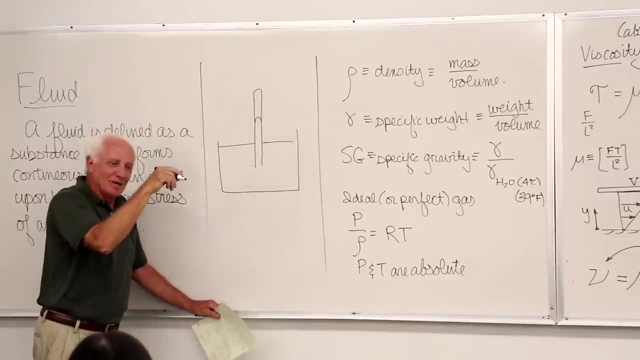 At this point, right here, you're going to see the temperature rise up. At this point, right here, you're going to see the temperature rise up. At this point, right here. mercury does this Around the glass perimeter. where the glass and mercury are in contact, the mercury's being pulled down. 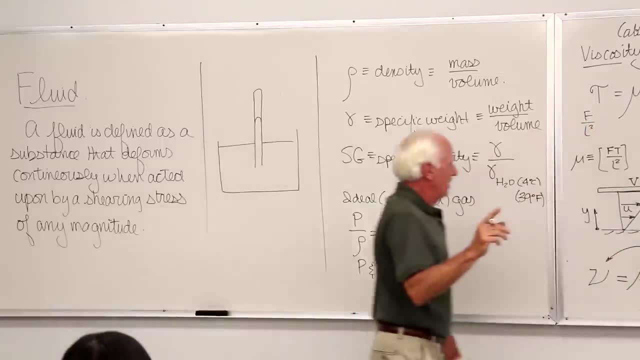 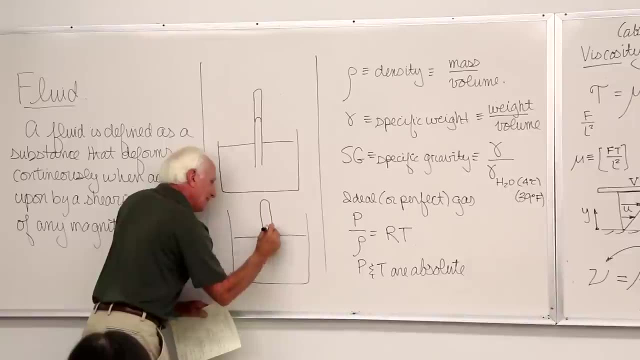 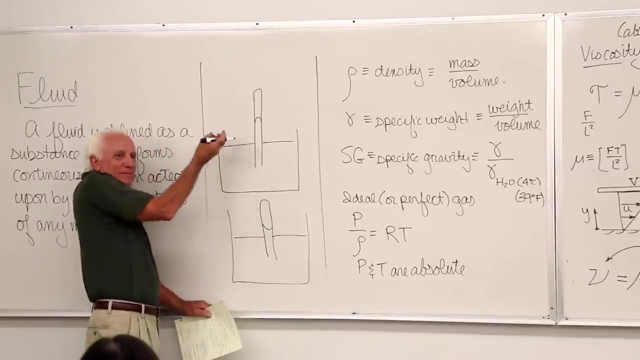 That's surface tension. That's surface tension. Take water. Here's a tube of water. Do the same thing. Doesn't work quite as well, but looks like that Water is being pulled up by the glass. it seems like So. it's a property. It's a property of the fluid and the temperature. 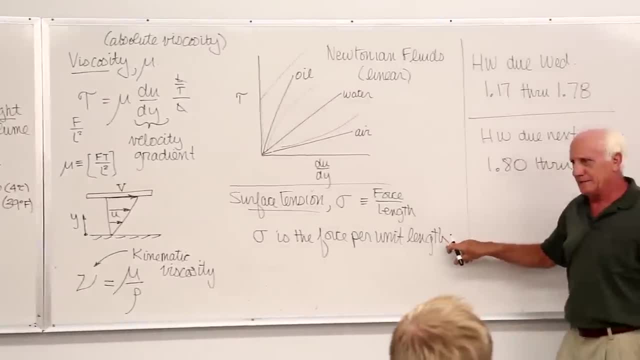 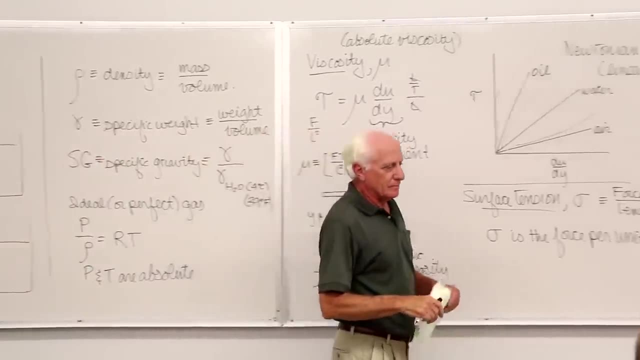 So that's why it's fourth per unit length. What length is this length? It's the perimeter of the glass tube, the perimeter pi times d. So that's a phenomenon that occurs quite often in fluids that you should be aware of. 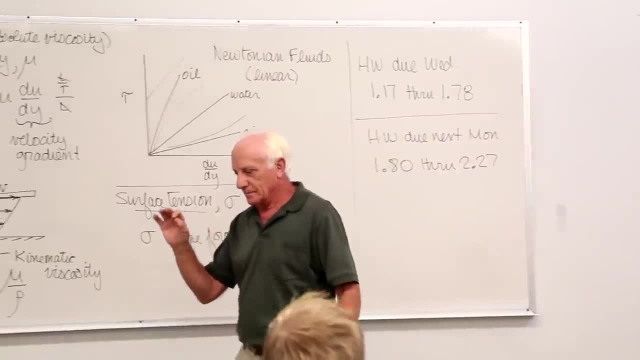 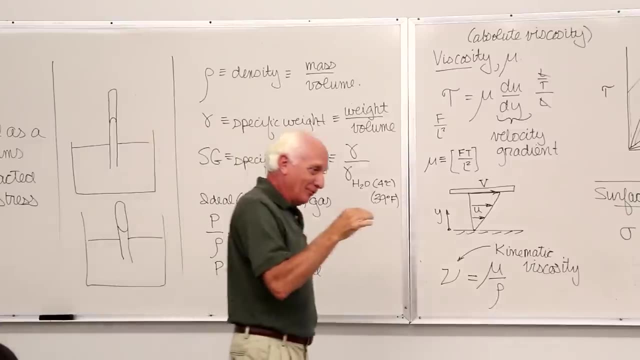 What's this thing called surface tension? Try and put- If you do it real carefully- a dime on water. If you're really really, really careful, you can float it on water. It won't sink. It won't sink. 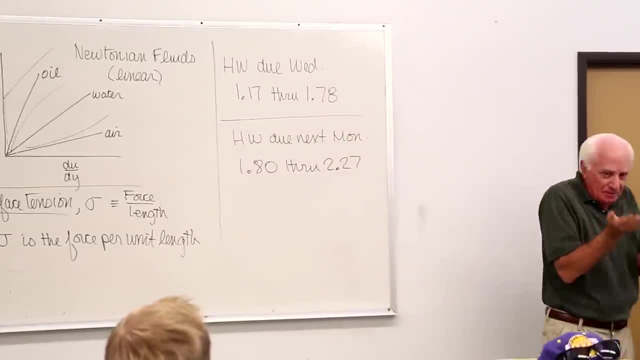 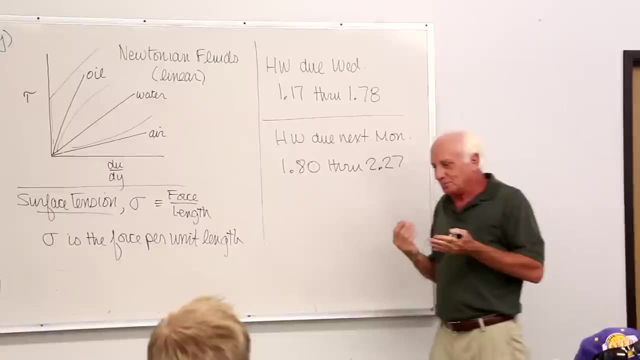 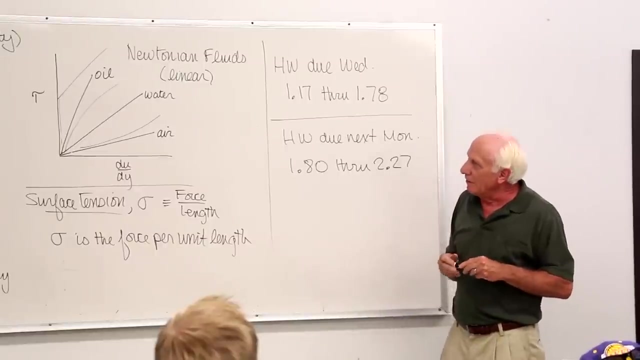 Something's pulling it up around the perimeter, Something's pulling it up, And that's the water doing that, And that's the surface tension in the water. So those are all part of the concept of surface tension. Okay, I think that pretty much covers all of our important properties. 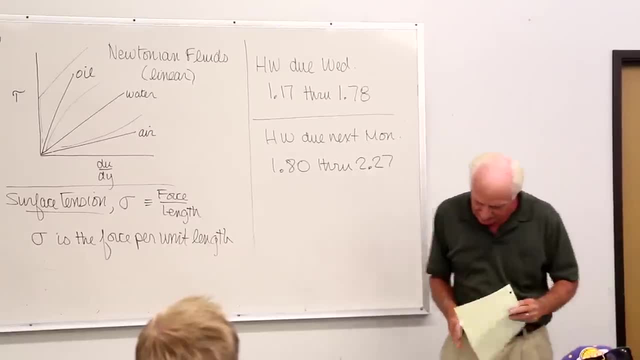 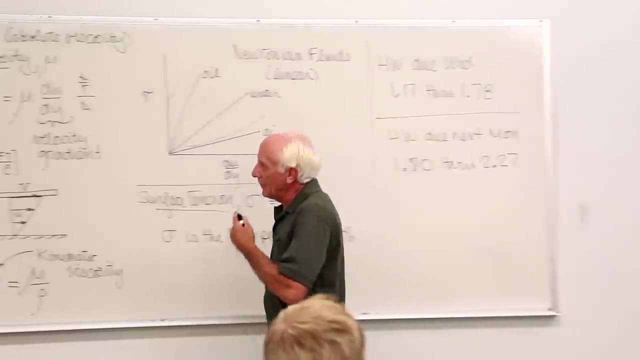 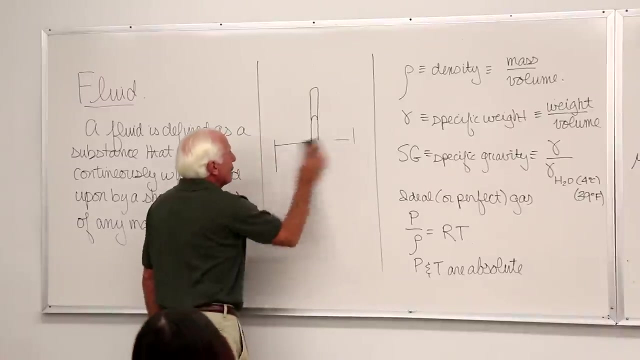 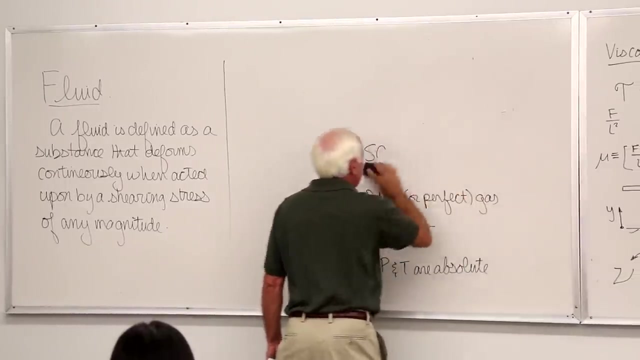 in there. So let's take a look then at pressure. All right, Now let's go back over here. Let's talk about pressure. It's one of the big concepts in our first fluids course. What do you call pressure in? 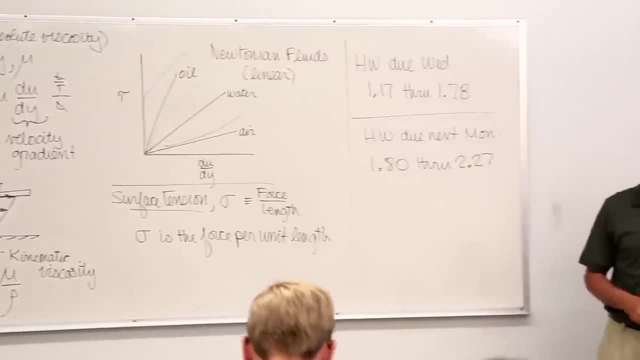 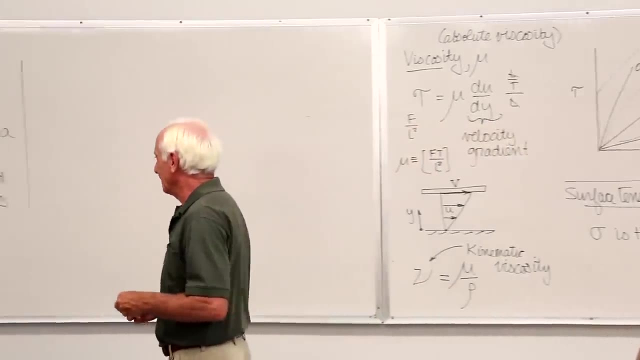 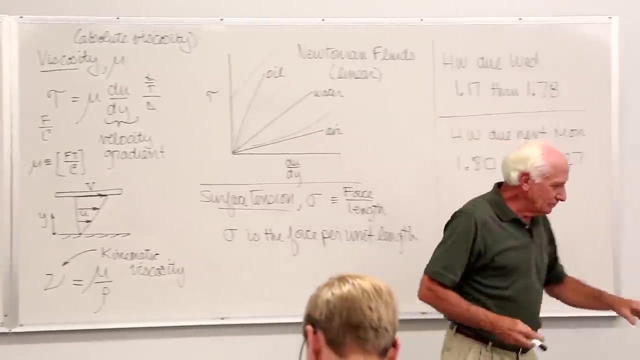 218: strength. What's stress Force per unit area? What's pressure Force per unit area? Right right, Different, but just different. Those guys are solids, These guys are liquids. Okay, Let's start off by absolute pressure. 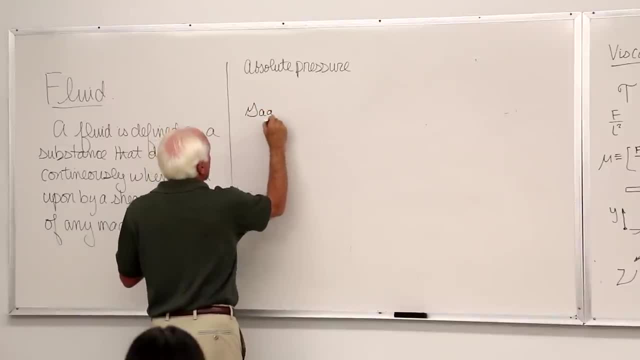 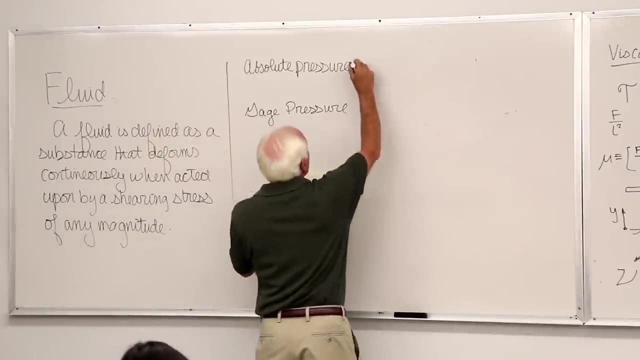 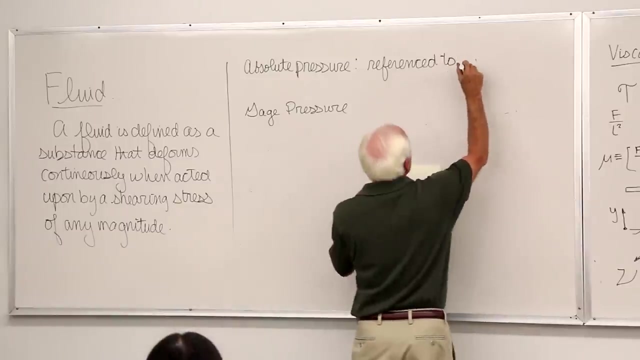 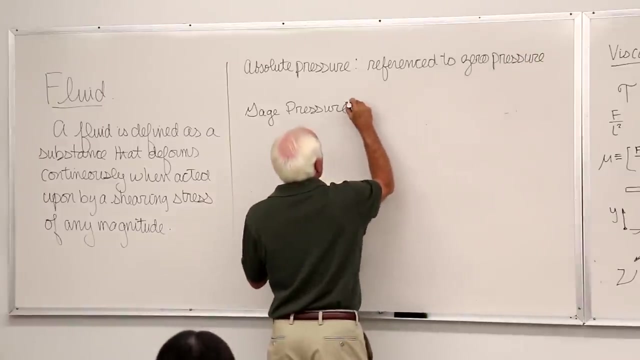 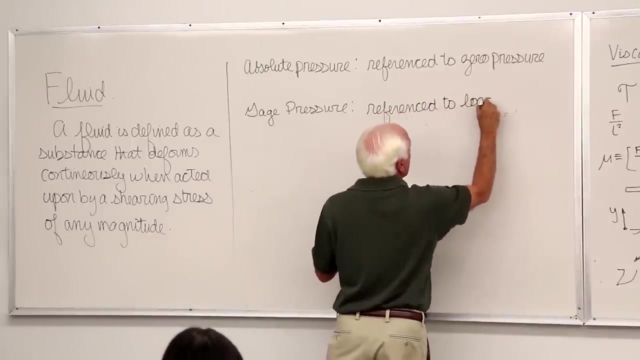 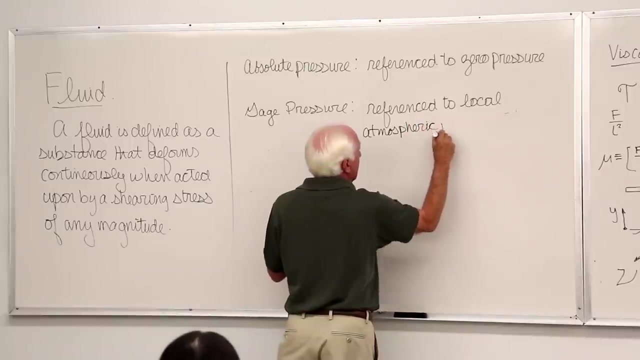 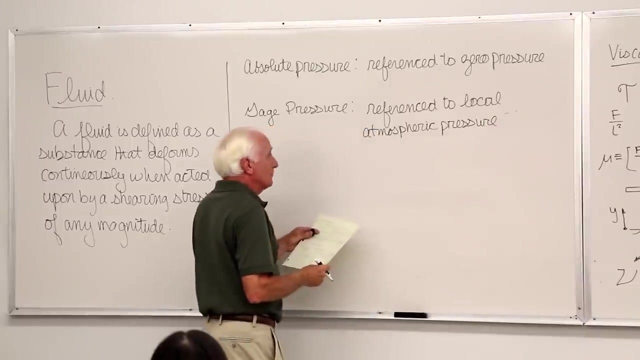 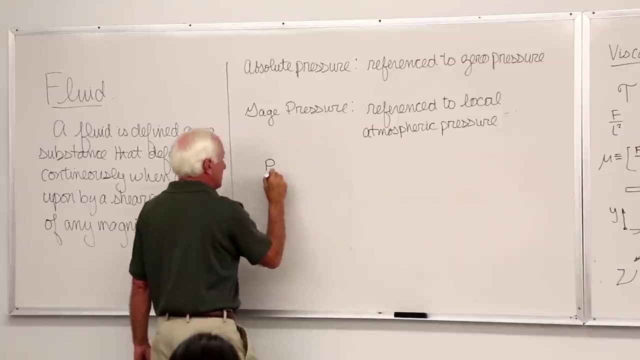 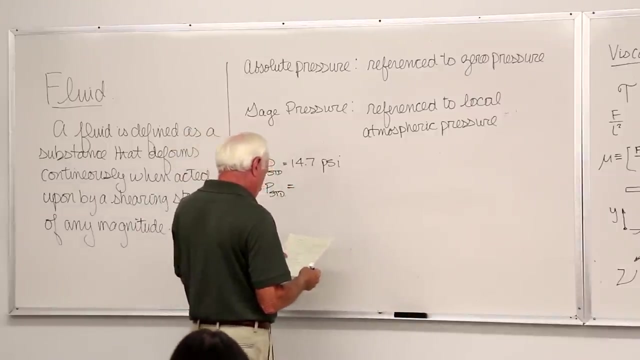 We'll put them all down. Gauge pressure: Okay, absolute Reference to zero pressure. Reference To local atmospheric pressure, We'll use our standard pressure, 14.7. BSI, And I think for our We'll just use 101 kPa. 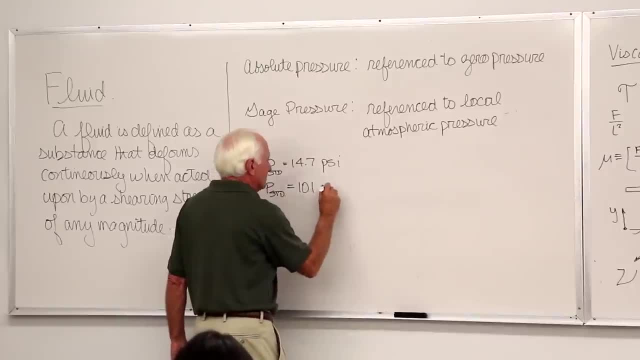 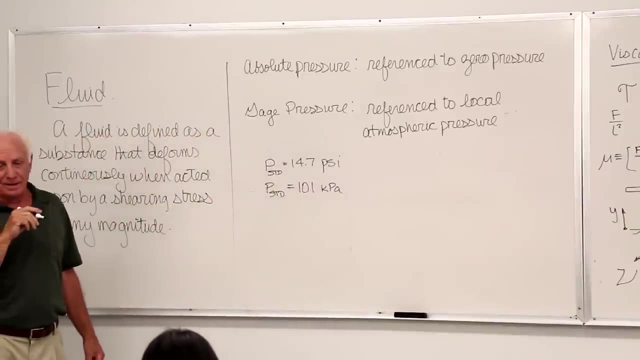 It's like 101.3-something-something-something, 101 kPa. So these are the standard pressure values. We're not going to use the value of pneumonia, which is, I don't know, air above sea level. 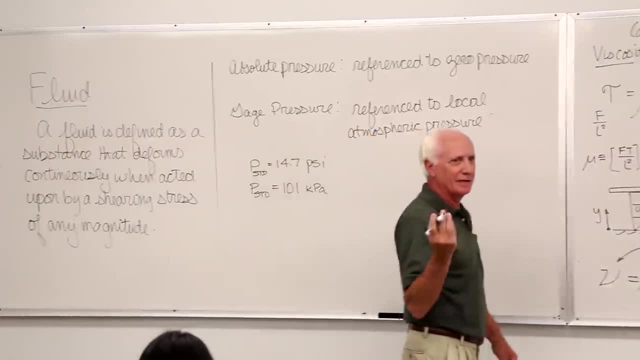 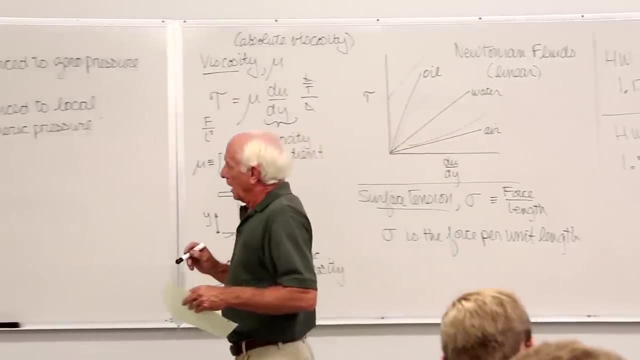 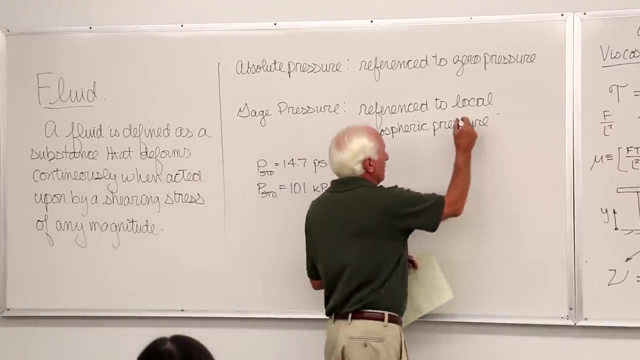 These guys are at sea level and I don't know. 34 degrees latitude or something like that. Standard values: We'll use those, Okay. Gauge pressure: Reference to local atmospheric pressure. The word local means where you are when you make the measurement. 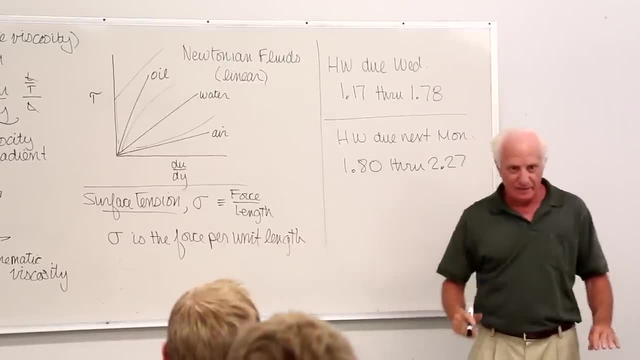 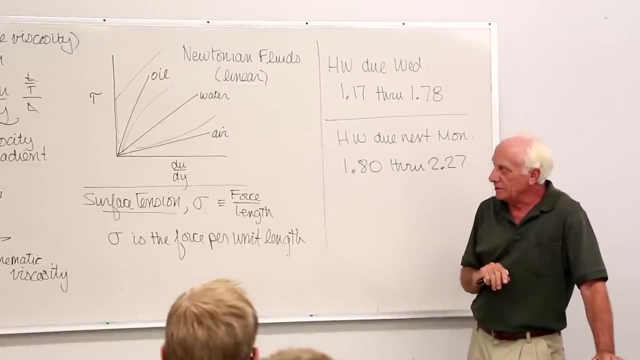 Local means where you are when you make the measurement. If you're in Pomona, California, Pomona, it's the pressure here. That's the local atmospheric pressure. If you're in Denver, Colorado, it's the pressure in Denver, Colorado. 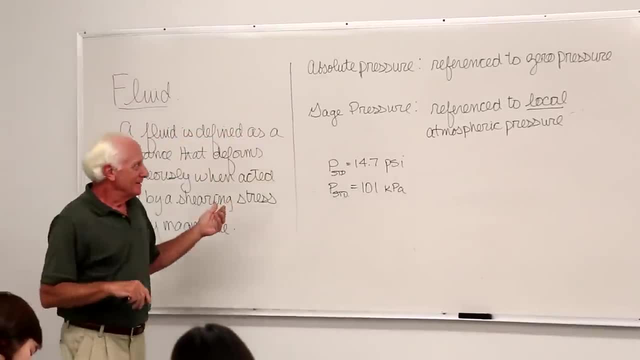 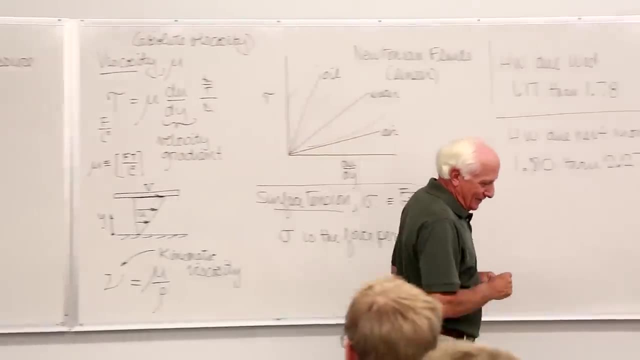 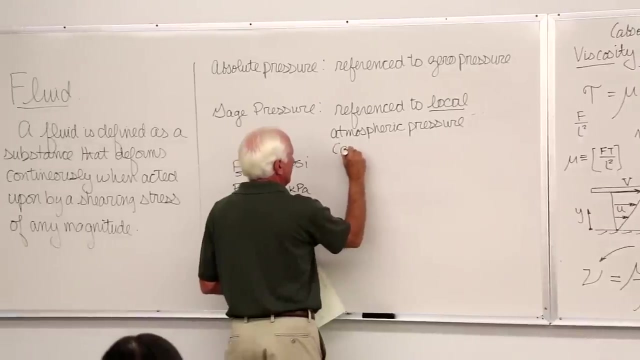 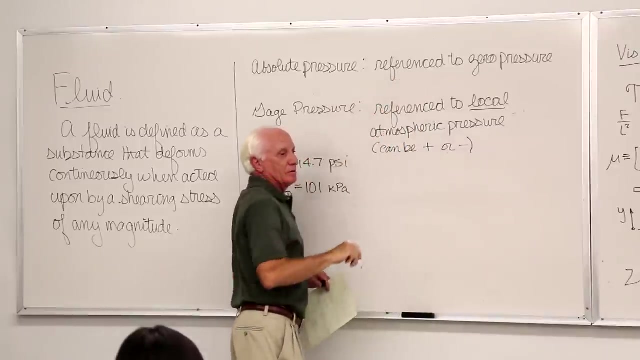 at that time of day, that day of the year. So that's reference to where you are. Okay, Now let's talk about these guys. Gauge pressure can be positive or negative. These guys are always positive because they're referenced to zero. 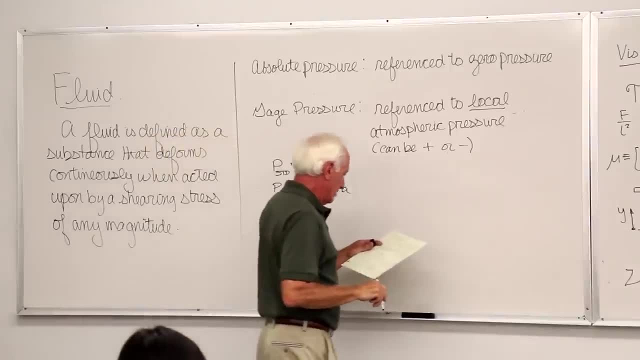 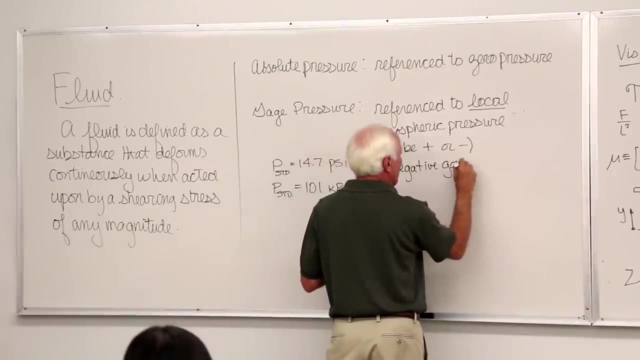 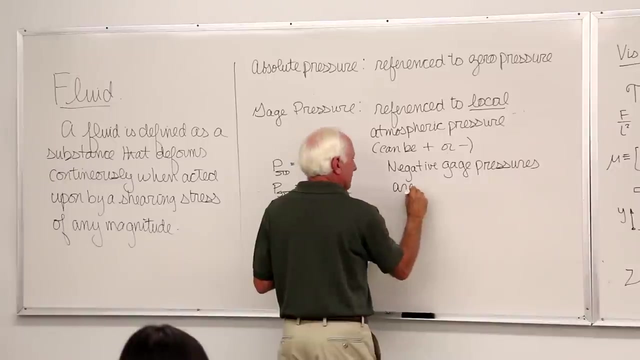 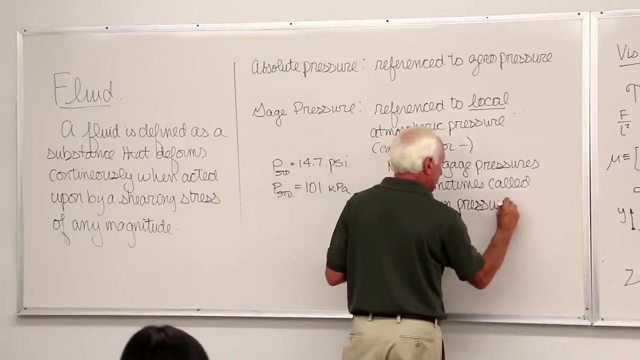 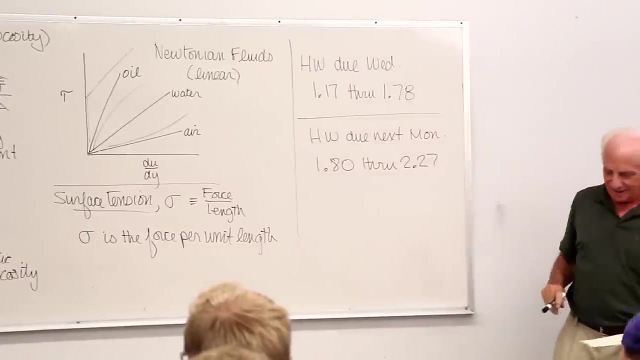 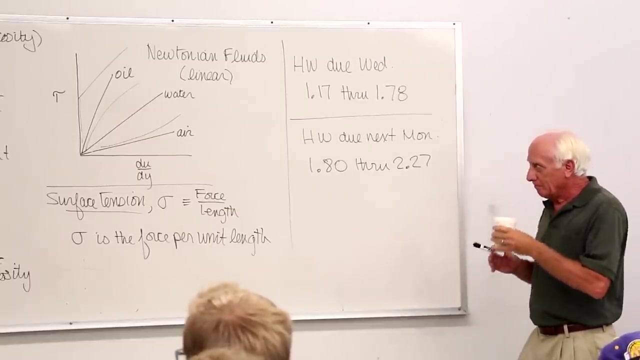 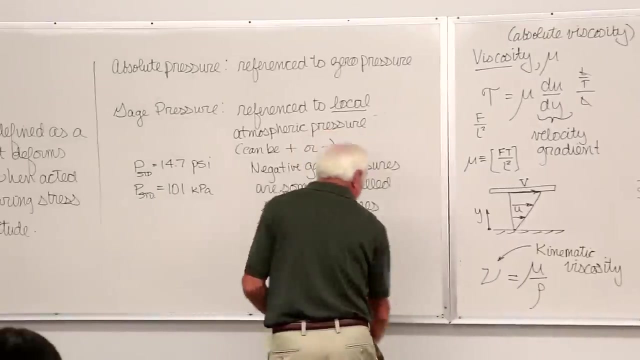 No such thing as a negative absolute pressure. Negative gauge pressures are sometimes called vacuum pressures. So here the word vacuum pressure, and some gauges will show you positive pressures and vacuum pressures. That's what they mean by that, Okay, So let's draw a little picture here that shows these pressures. 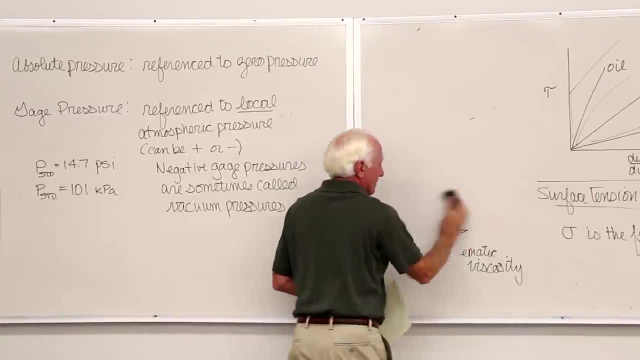 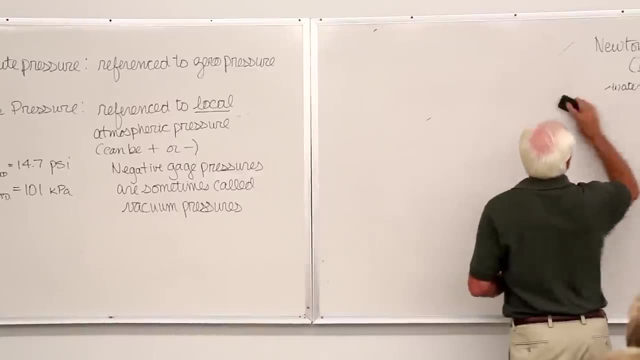 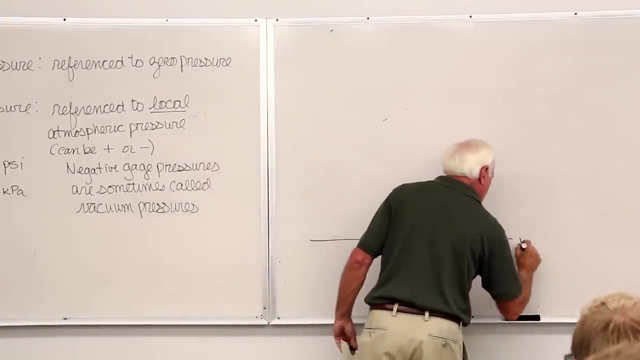 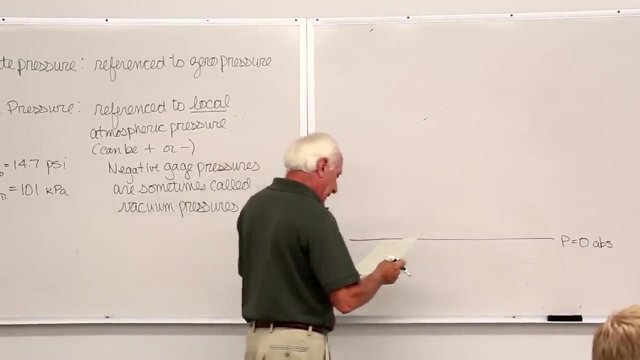 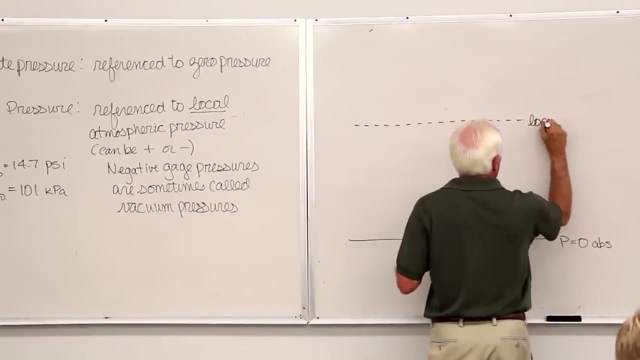 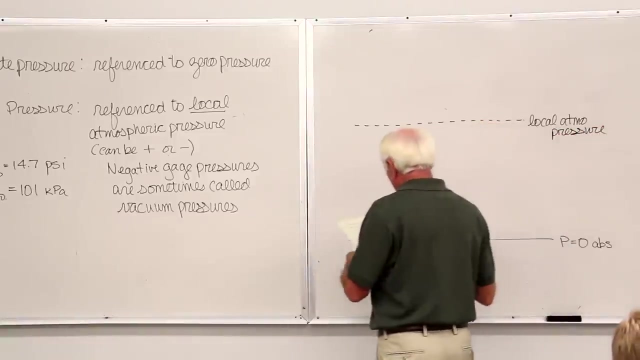 Pressures. I'll put on the board the values of some conversion factors too for you. Let's start off with zero pressure down here, Zero absolute, And let's say that this is the local atmospheric pressure, And let's call that 101 kPa. 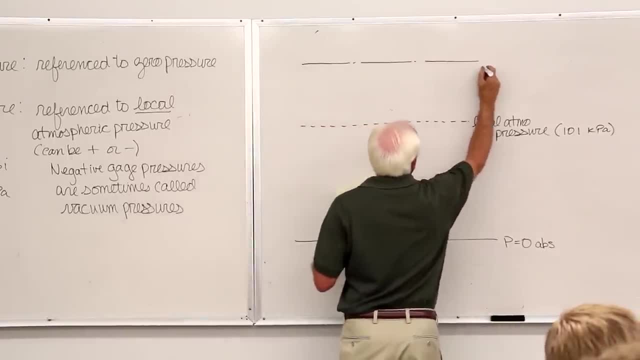 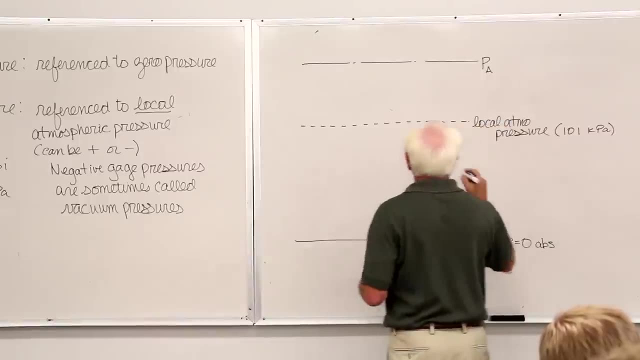 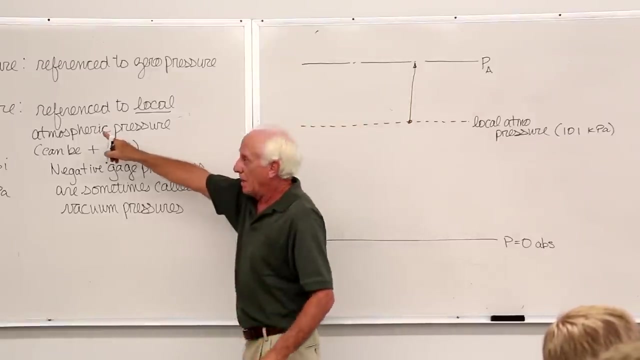 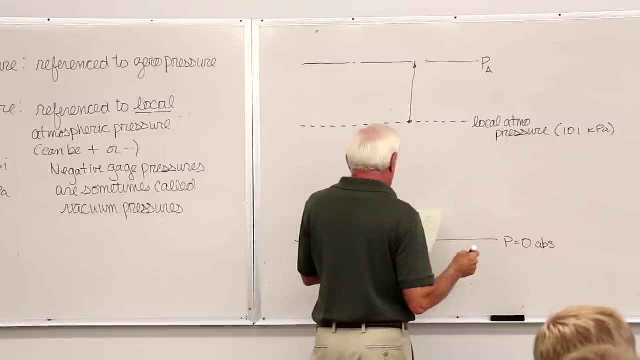 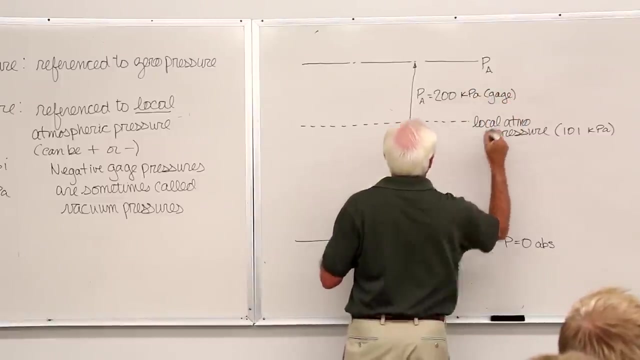 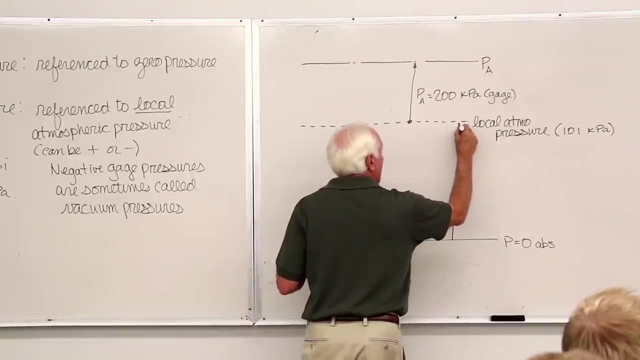 And let's call the pressure up here Pa. If I measure Pa from the local atmospheric pressure, reference to local atmospheric pressure, that's this line right here, And Pa is going to be this- is given 200 kPa Gauge. 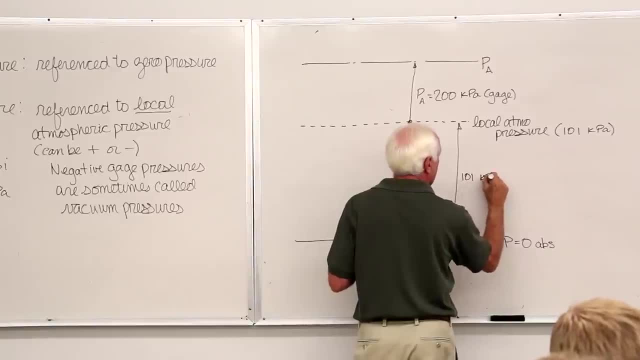 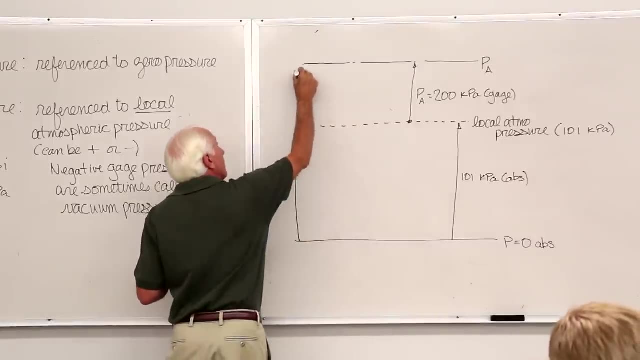 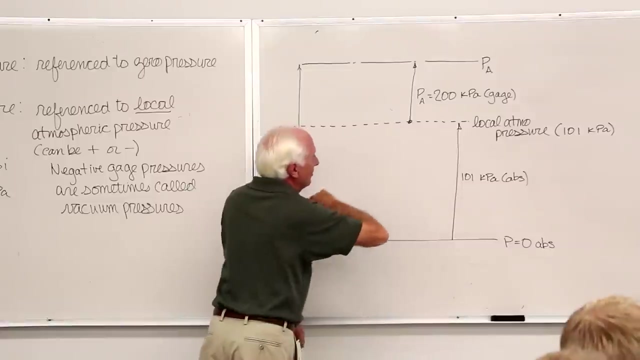 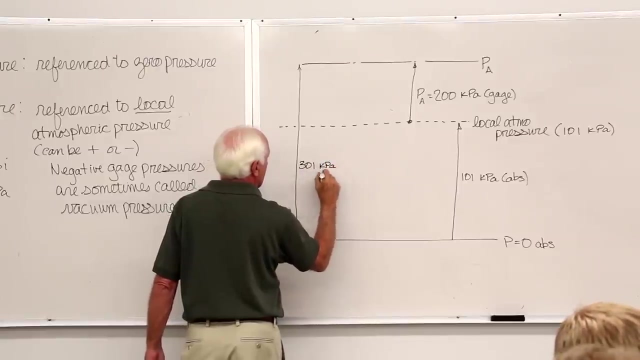 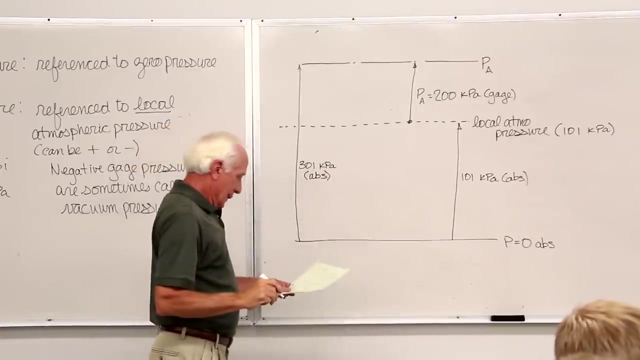 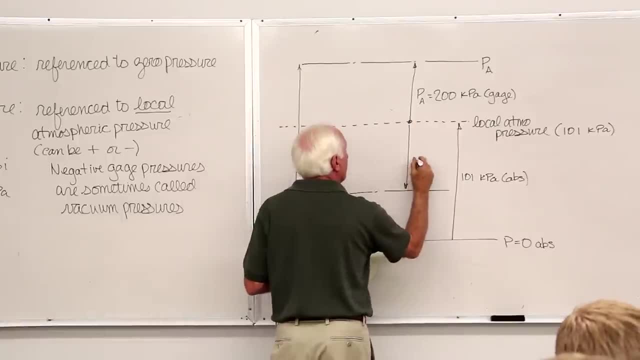 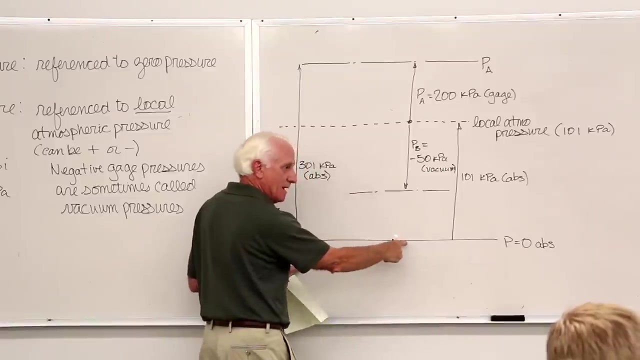 and let's say that it's minus 50 kPa gauge vacuum, then the absolute pressure always is measured. then the absolute pressure always is measured from the bottom down up to here. from the bottom down up to here, 101 minus 50, 51.. 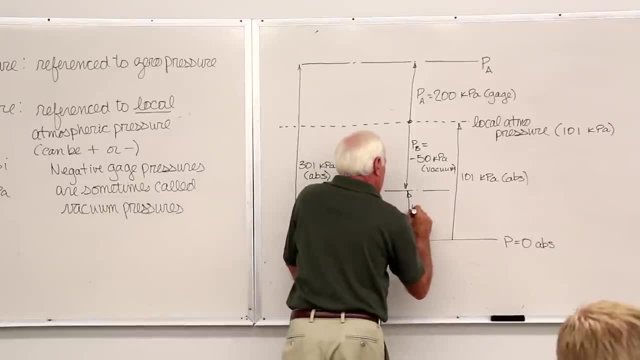 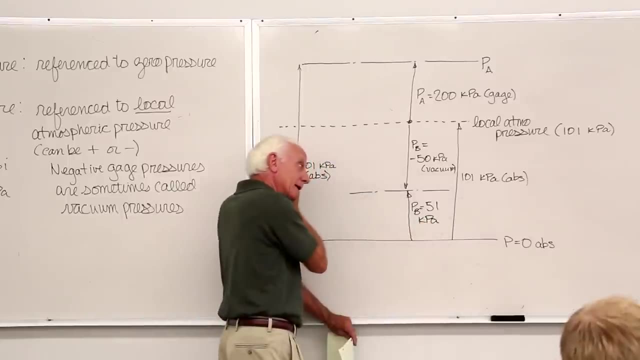 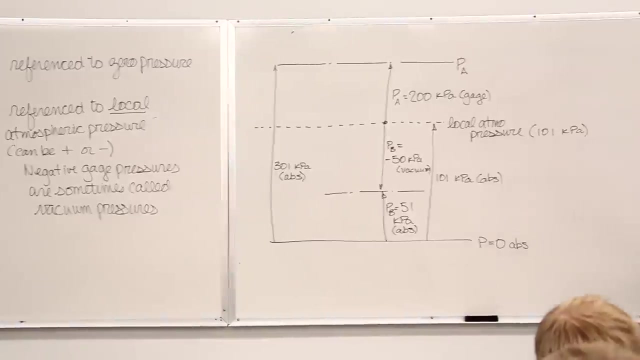 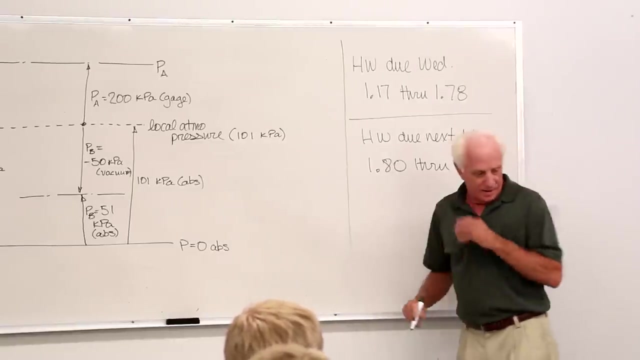 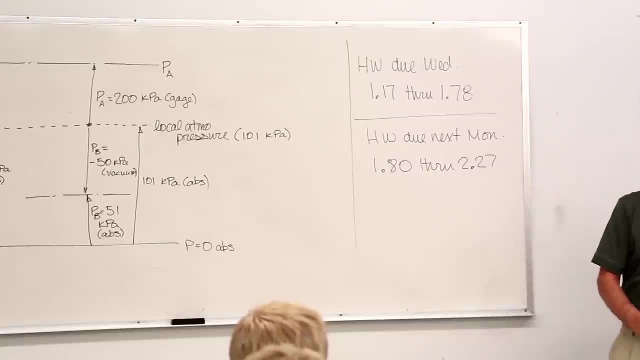 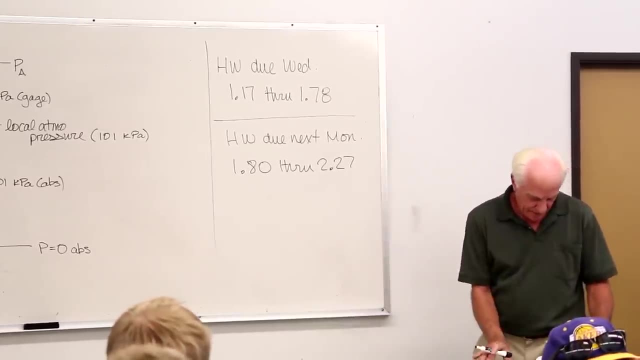 In the textbook. In the textbook, I think he gives us a big hint. I think he gives us a big hint. Let's see what pressures are here. This picture is in the book too, by the way. Yeah, it's on page 50.. 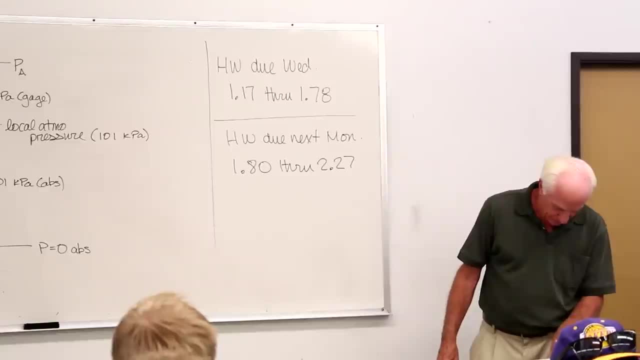 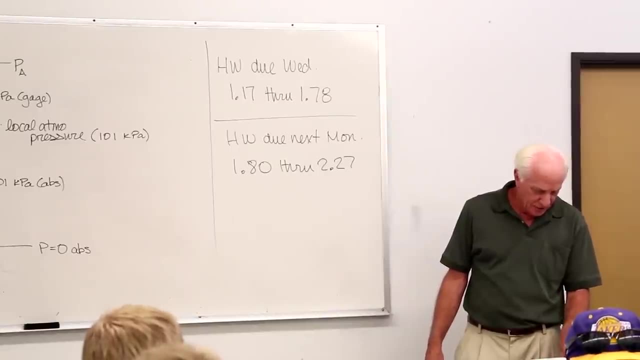 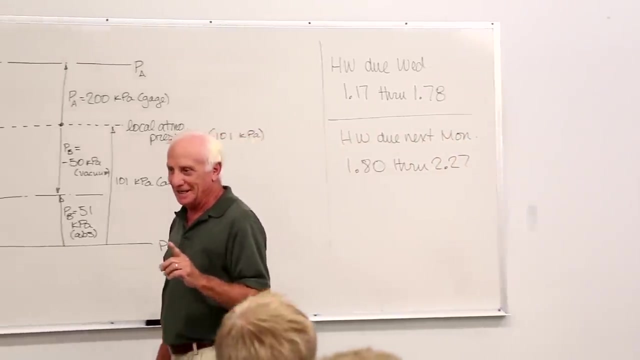 Okay, Here's what he says in italics In this textbook: pressures will be assumed to be gauge pressures unless they're specifically designated as absolute In this book for homework. in an exam for a problem, the pressures are assumed to be gauge unless it specifically 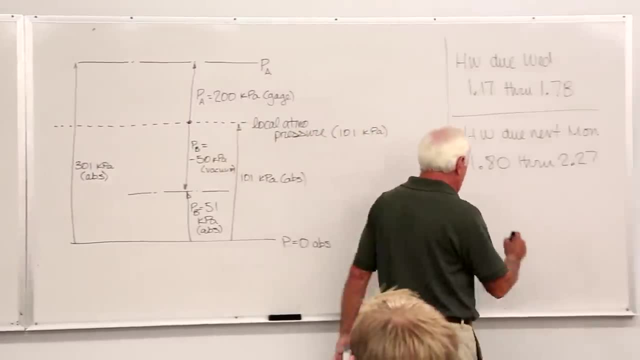 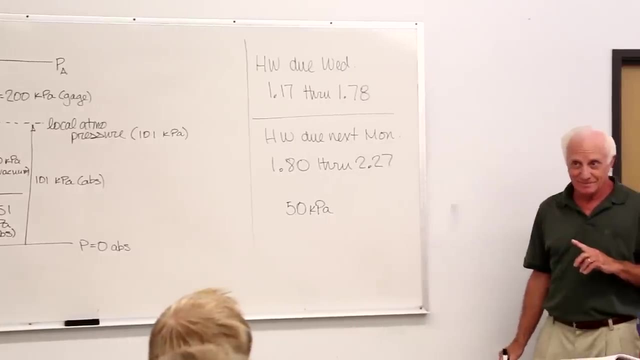 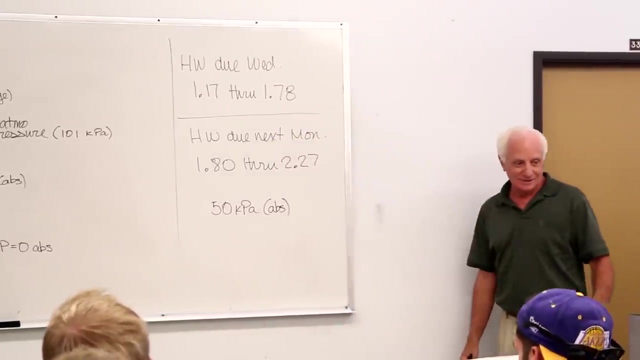 says absolute. So if I give you a problem on an exam and it says the pressure is 50 kPa, that means you assume that's gauge. Unless I put that, then it's absolute. So that's the default rule. The default rule is: 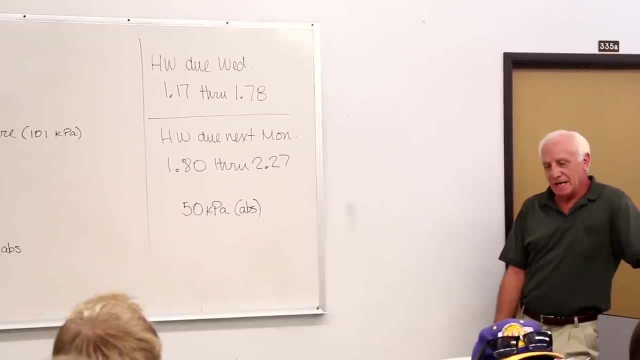 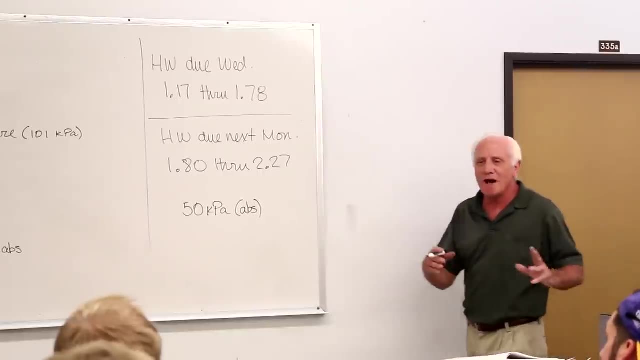 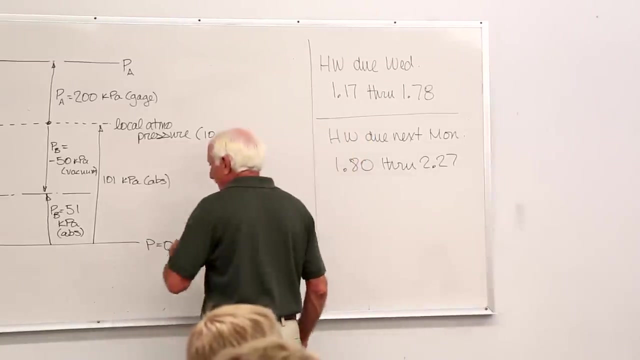 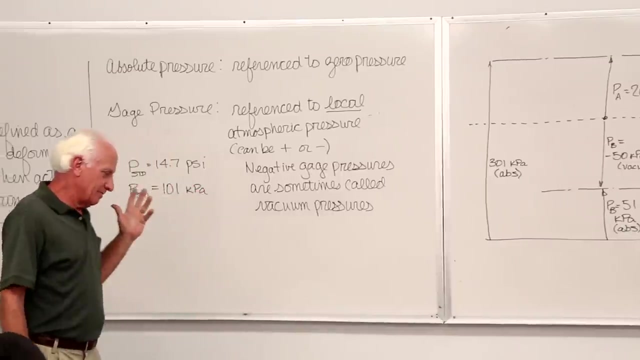 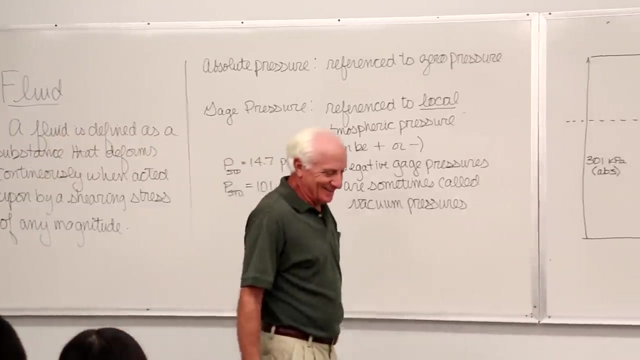 pressures that just are in kPa, assume that they're gauge, unless they're absolute. There will be a corrent abs after it Or the problem will say: the absolute pressure is 50 kPa. Okay, In English engineering or British gravitational, if someone tells you the pressure. 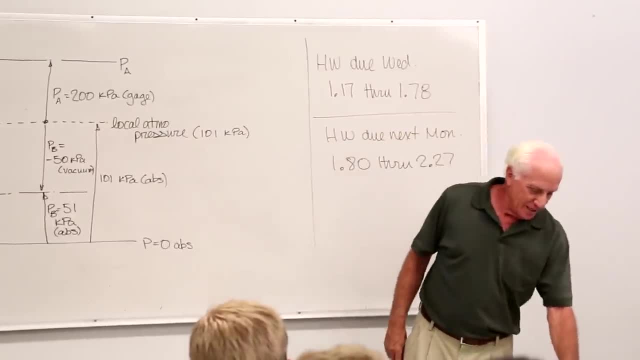 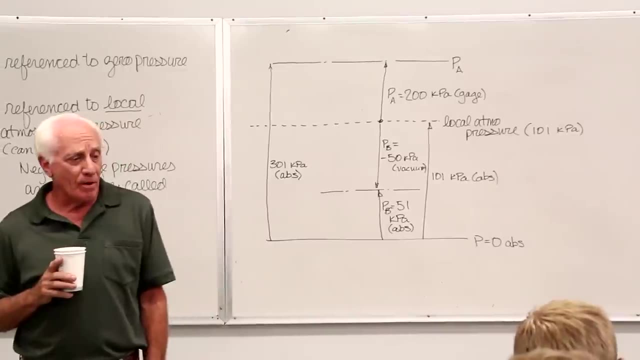 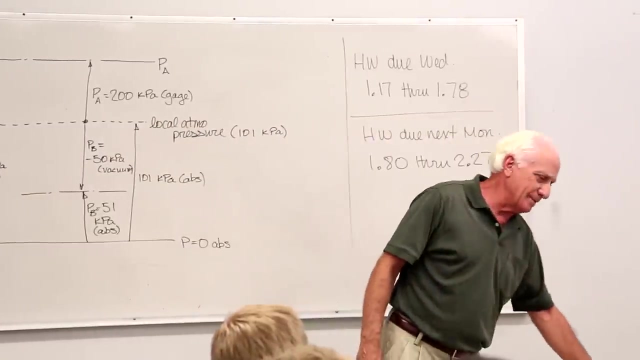 of the air in your tire- make it easy- is 30 psi. How do they measure? Oh, probably a tire pressure gauge. I would suspect a tire pressure gauge. How does a tire pressure gauge work? Oh, a typical example. There's a. 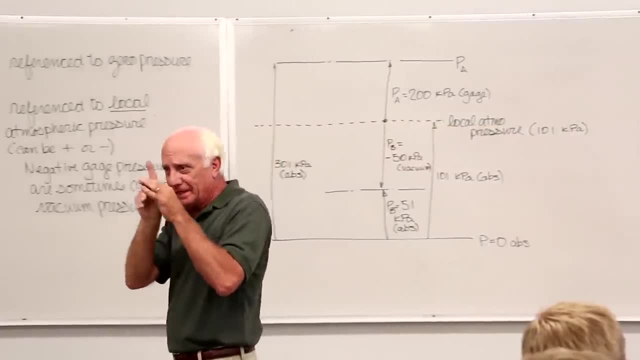 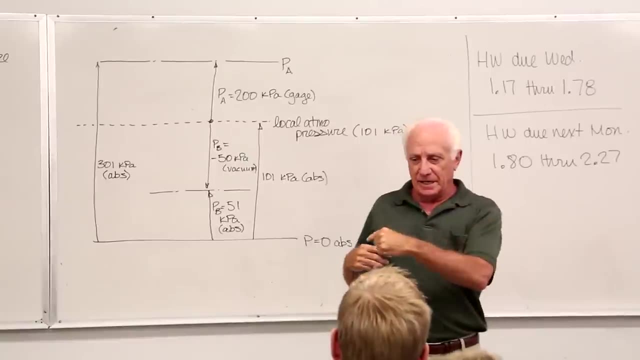 spring in this thing and the stem pops up and you read it. Or there's a circular gauge you put on your tire and you read it. Take the spring gauge for one. What's the pressure in your tire doing to that thing? Oh, it's. 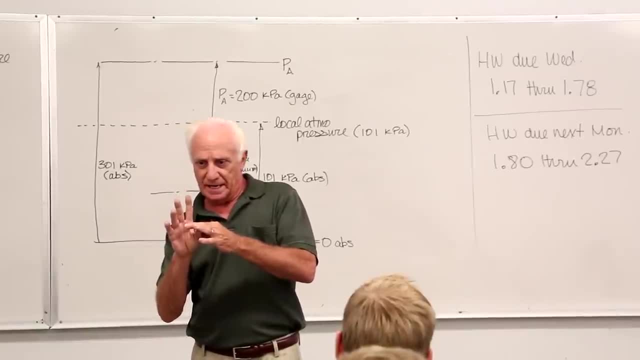 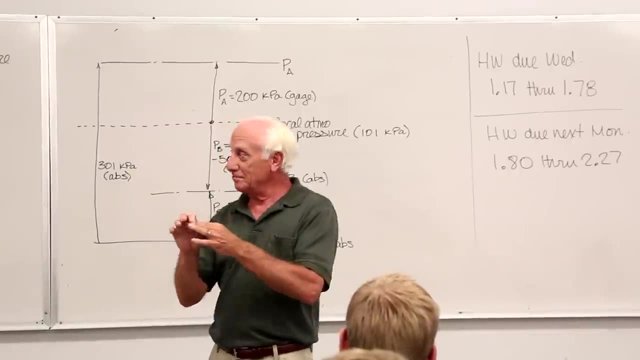 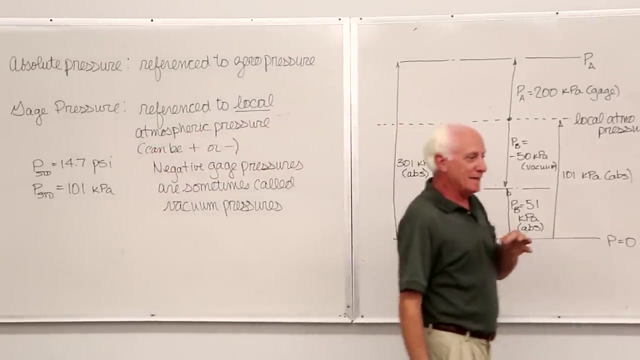 compressing the spring as it pushes it up. What's it working against? What's outside that pencil-like device? So what's it? measuring the pressure with respect to 30 psi means that's 30 psi gauge. And we don't say nobody says. 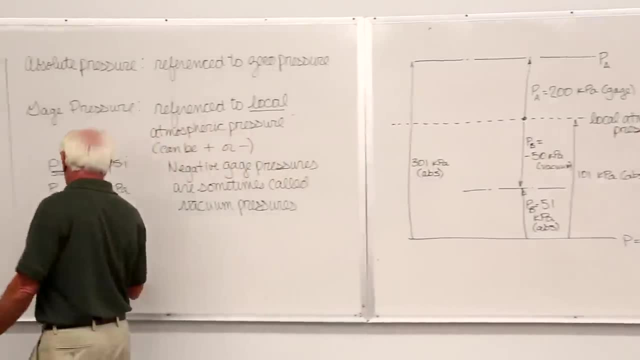 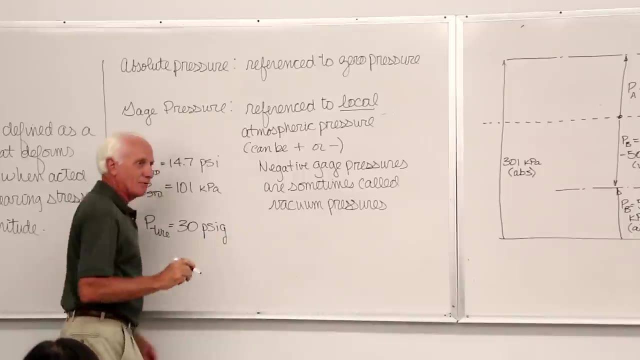 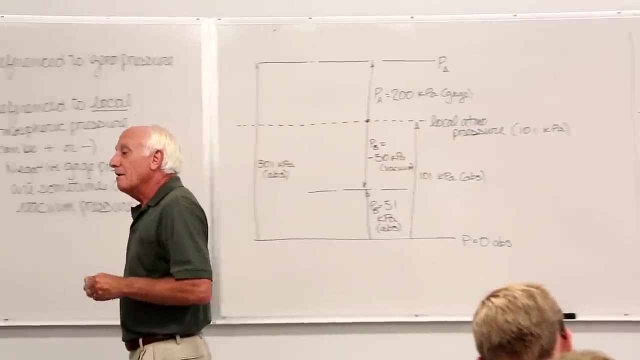 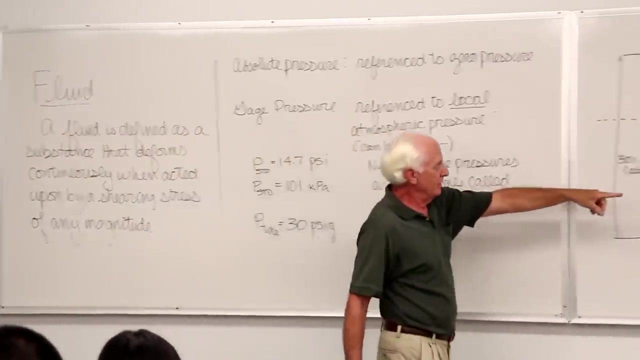 30 psi gauge. We say my tire pressure 30 psi g. That's standard practice. psi g means gauge. If somebody says: well then what's the absolute pressure of the air in my tires, Here it is. You're up here now at 30.. 30.. Above local atmosphere: 30.. Local atmosphere. I think I erased it. Yeah, there it is: 14.7.. 30 plus 14.7.. 44.7 P-S-I-A means absolute. That's just the way most engineers work. 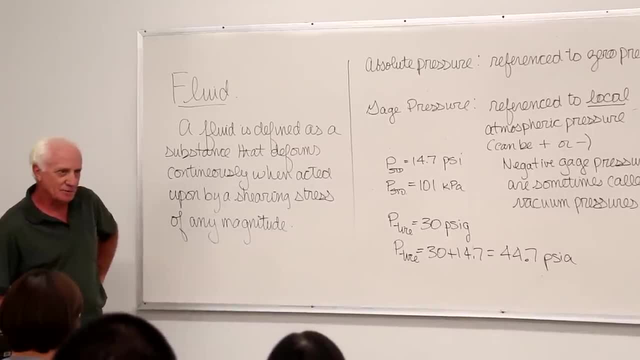 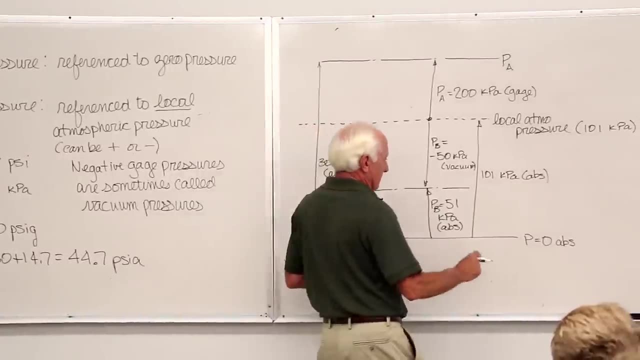 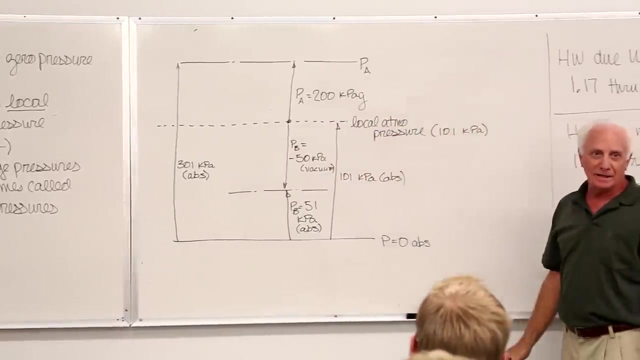 They use P-S-I-G for gauge pressure, P-S-I-A for absolute pressure, But in the world of SI, in the world of SI, you don't say, you don't say this- There's no such thing as a K-Pag. There's no K-Pag in the world. 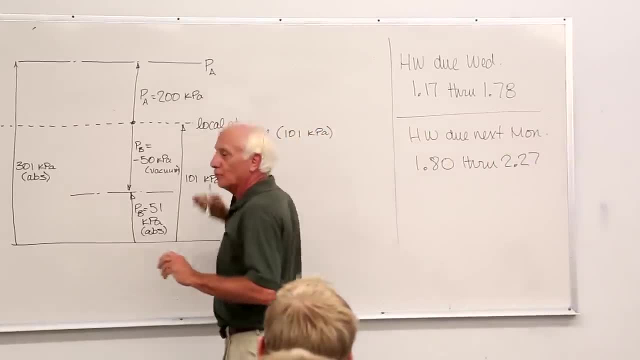 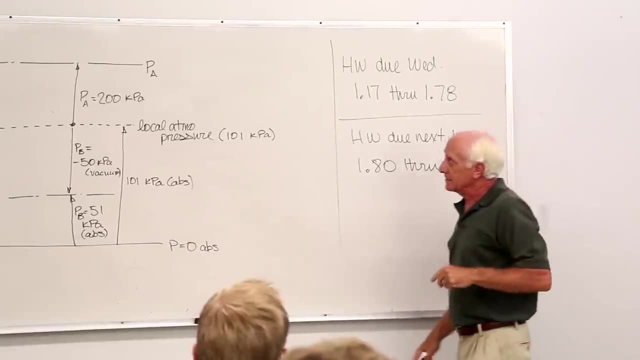 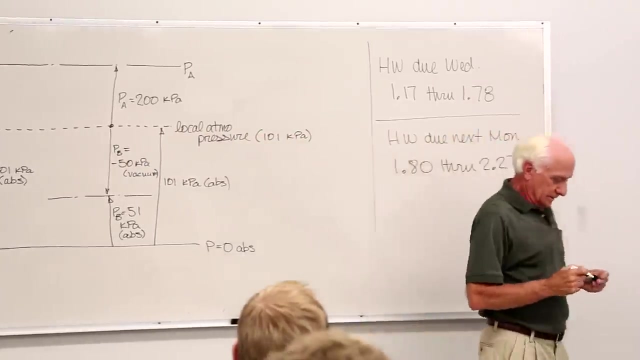 So what do you do? You have a rule. Textbook rule says: if I don't put anything after K-Pag, you assume that it's a gauge. If it's absolute, I'll put A-B-S after it, Just so on the exam you'll say: 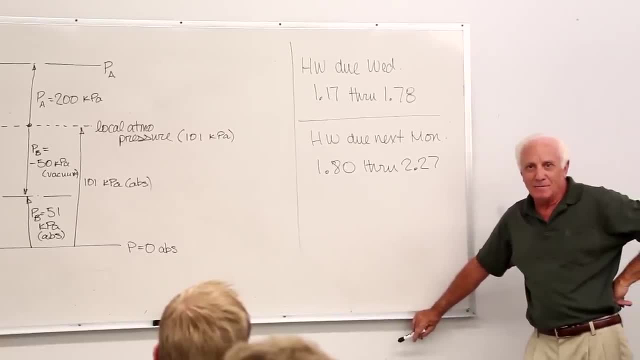 Professor Bill, what do you mean by that K-Pag? I'll say: go back to the default. what it would say: You don't want to get confused on an exam, A timed exam. It makes life miserable. Okay, so that's the pressure now. And the guy that says: 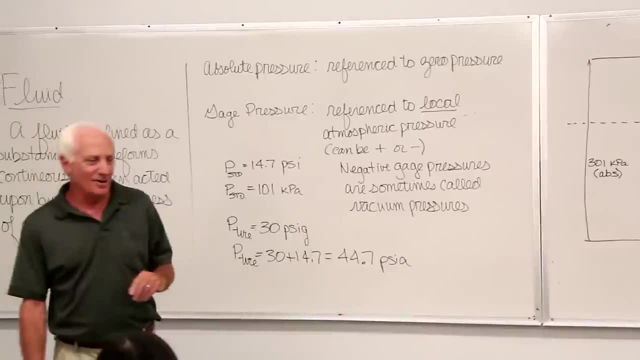 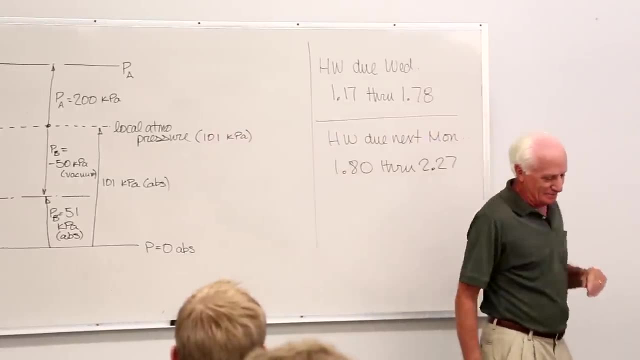 what do you want? your tires at 35 pounds? Say no, I want 35 P-S-I, Because they take a shortcut. They just say pounds, They really mean P-S-I, of course. Okay, now let's take a look at. 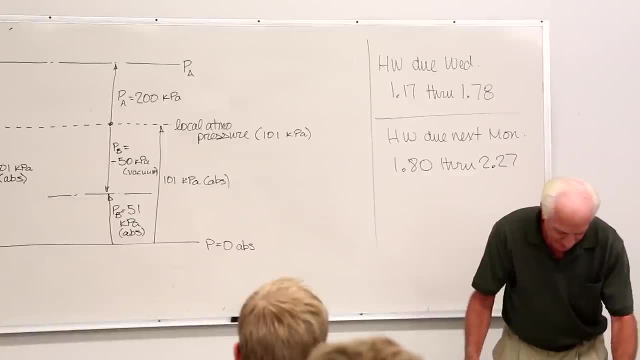 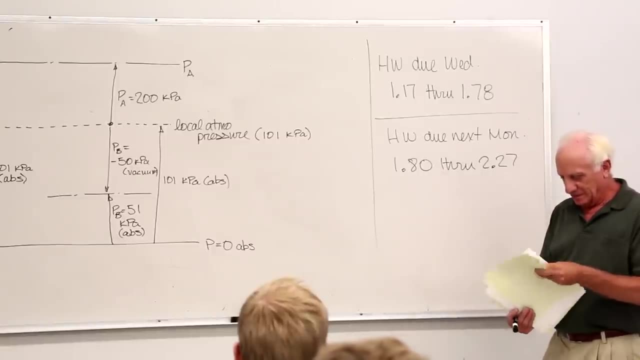 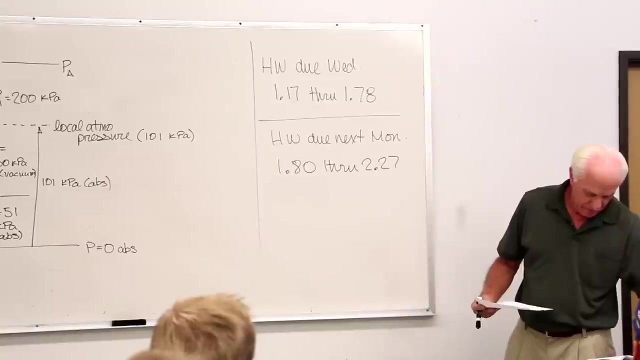 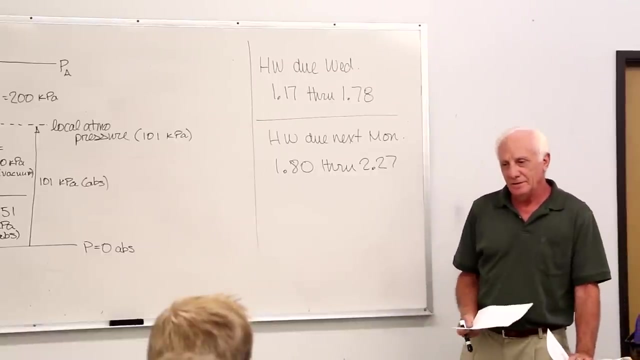 some problems similar to homework. Let's see which one I've got here. I'll take this one first, because it's a 177.. 177. This book, by the way, why do we use a textbook? It is the most popular Lumen Connect textbook in the United States. 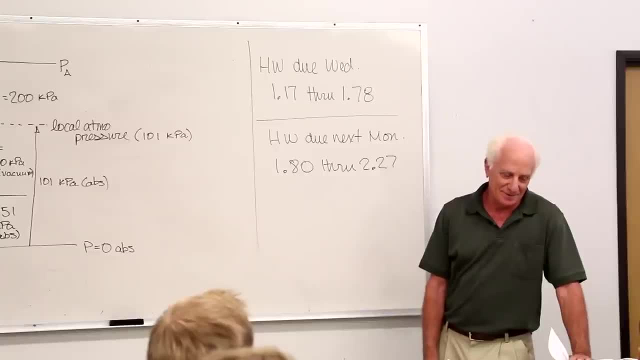 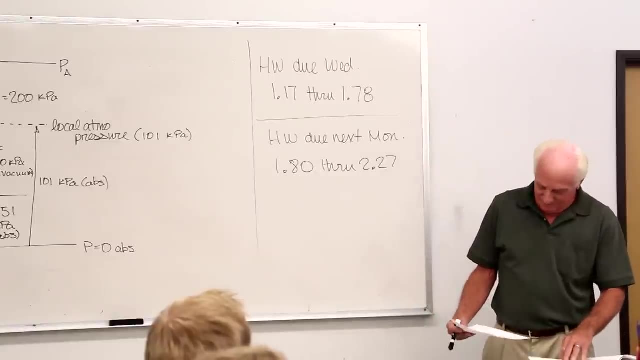 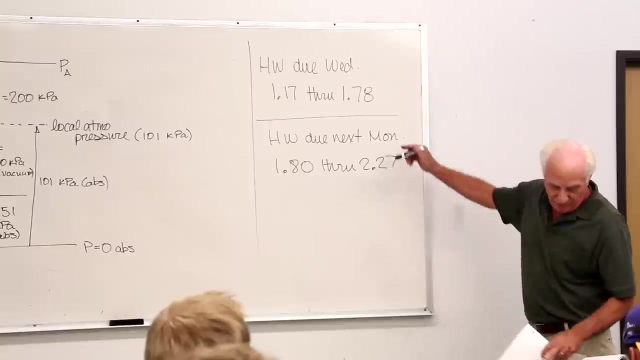 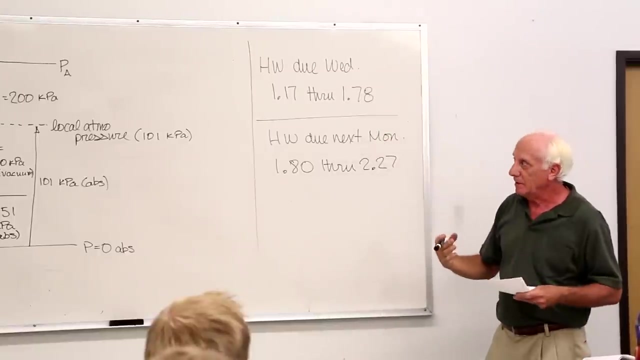 It's the most popular English textbook in the United States. That's why And the reason why it's very well written. Okay, 177.. You have 178 and 180.. They're all the same kind of problem. They're viscosity problems. 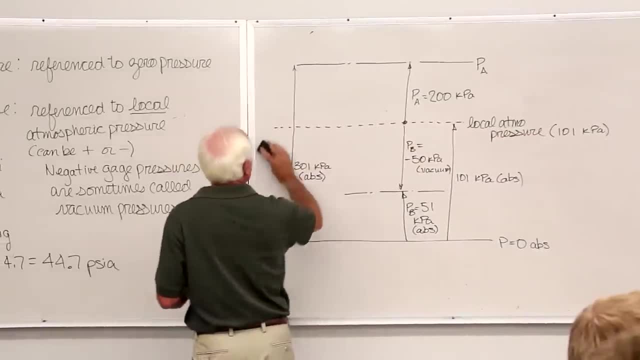 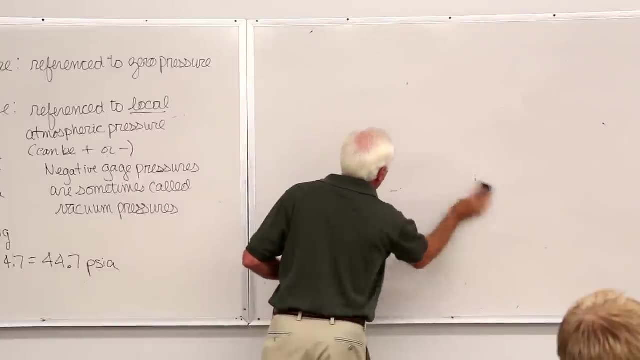 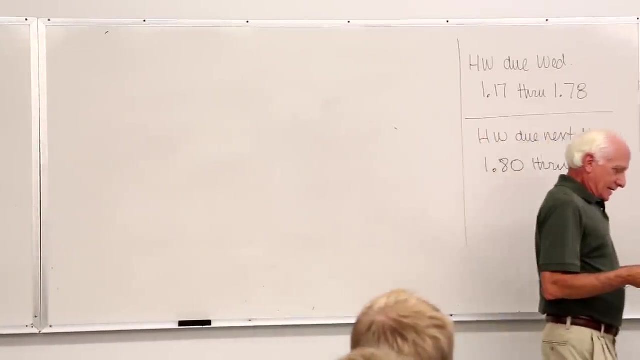 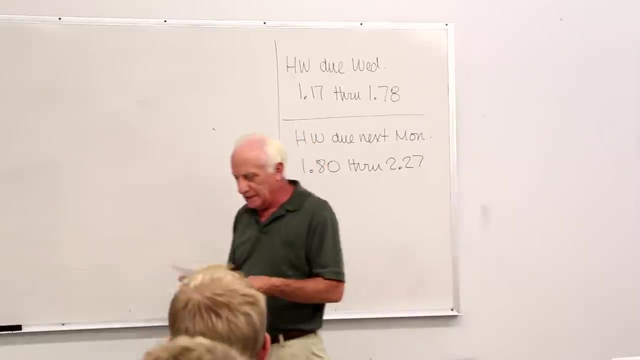 So we don't need this. Okay, I'll read it for you. It's a snow sled. The sled shown in the picture slides along a thin horizontal layer of water between the ice and the runners. So here's the sled From 177.. 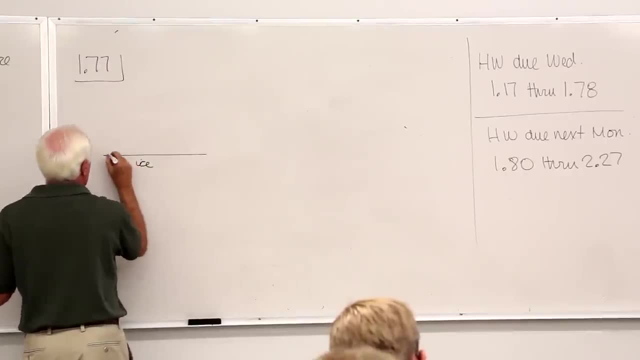 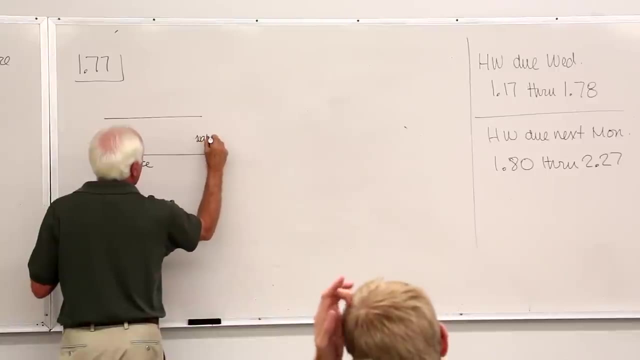 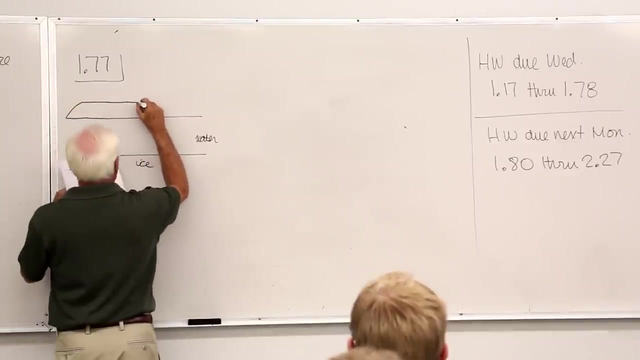 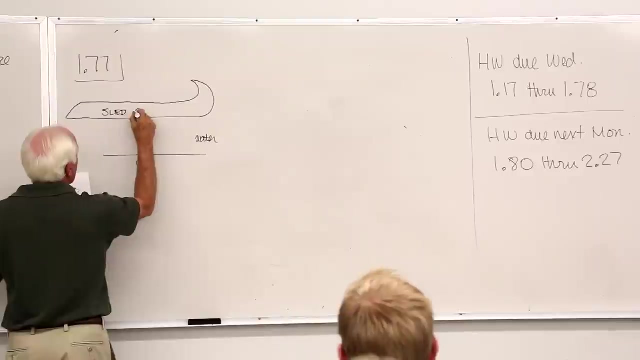 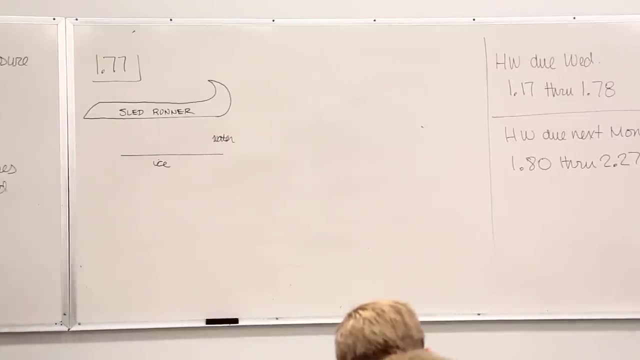 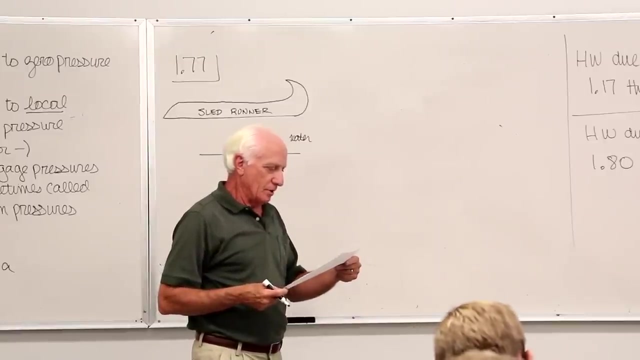 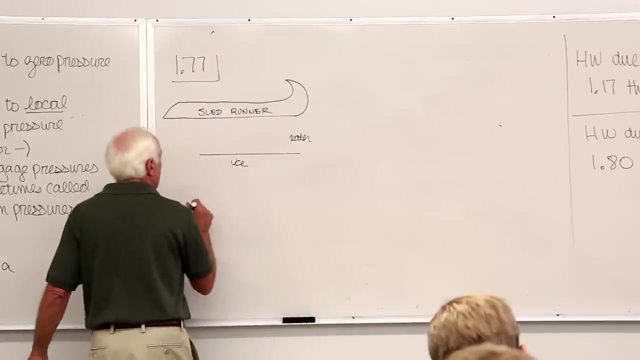 Here's ice. I'm going to expand it up. Here's water. Here's the runner on the sled: A blade, That's a skate blade. The horizontal force that the water puts on the runners is equal to 1.2 pounds. 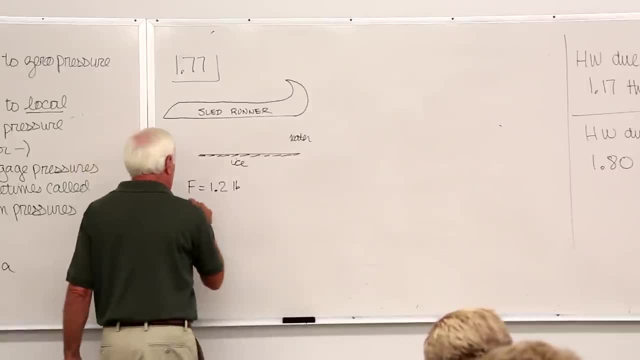 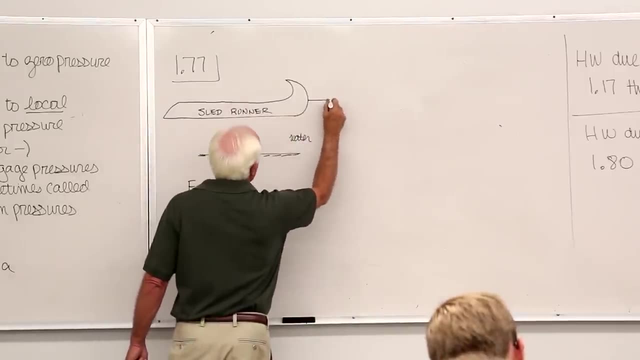 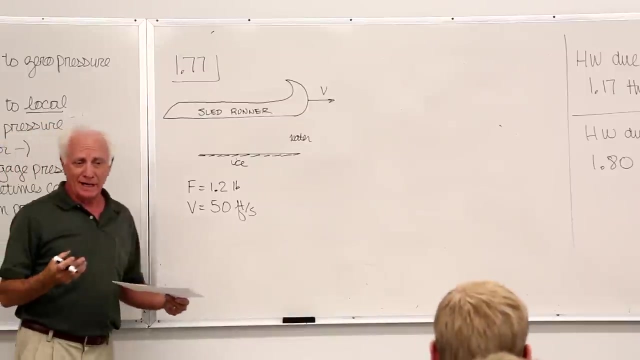 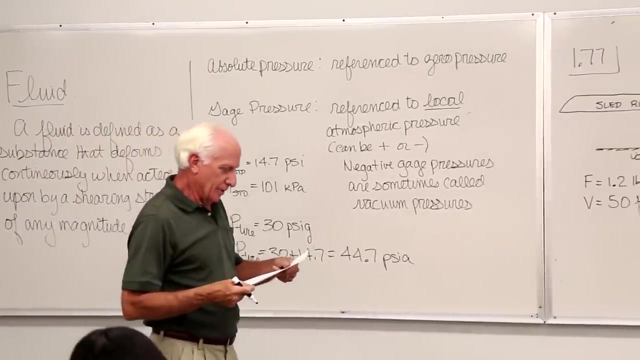 The sled's speed is 50 feet per second. Hmm, The sled's speed is 50 feet per second. The sled, the runner, the blade, runs on water, not ice Water. The total area of both the runners in contact with the water is 0.08 square feet. 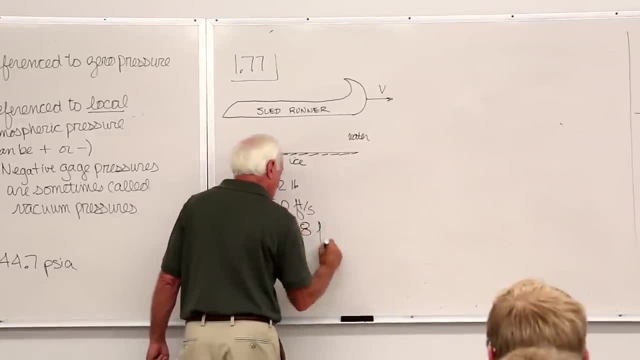 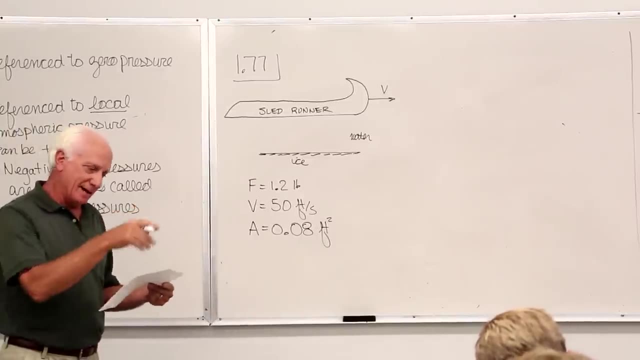 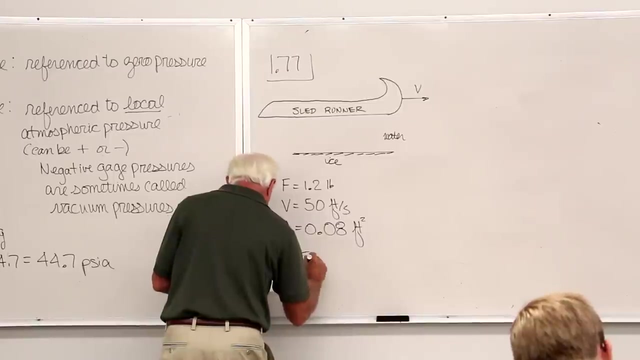 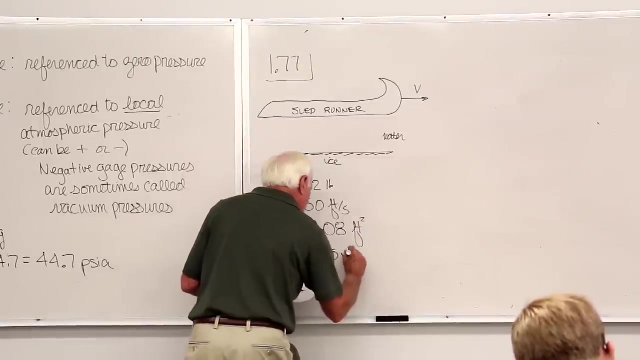 0.08 square feet. the viscosity of water: if they didn't give it to you is to the fact that they gave it to you. viscosity of water: 3.5. so this is new. they didn't say kinematic, they just said viscosity. assume it's absolute: 3.5 times 10 to the minus 5. 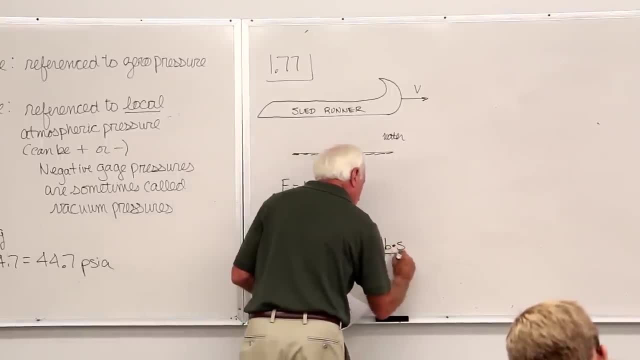 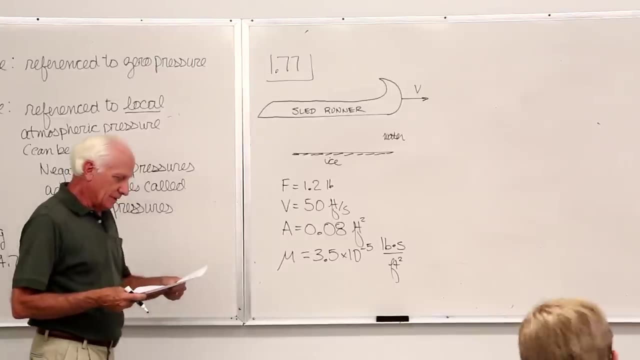 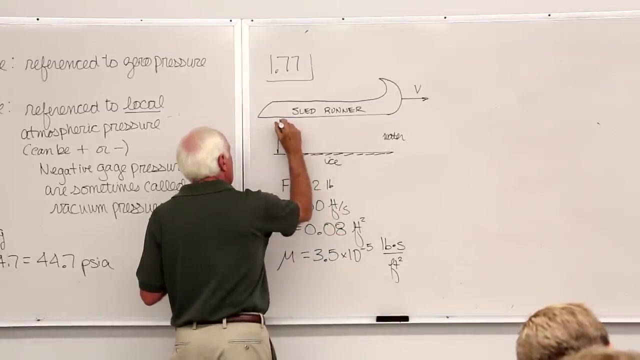 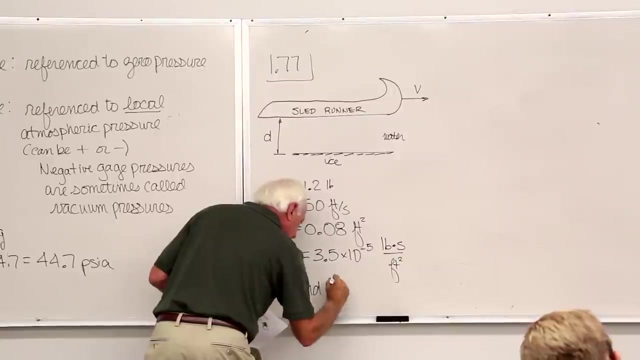 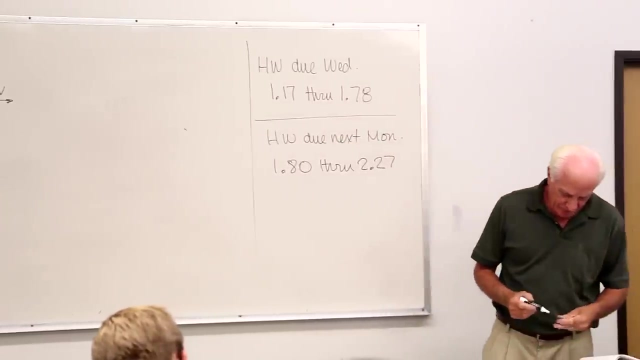 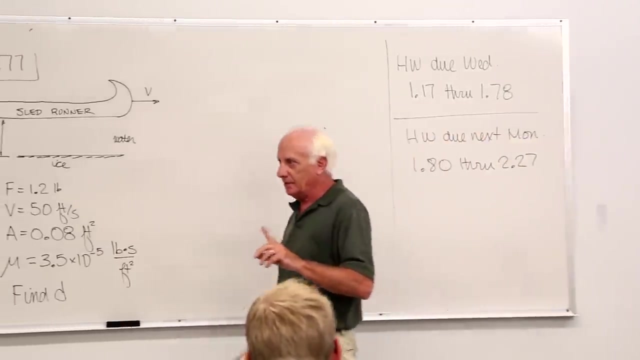 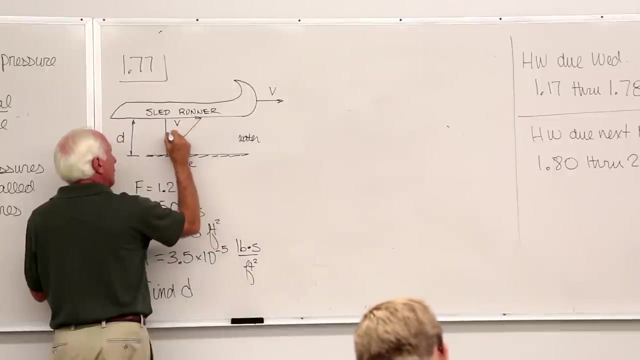 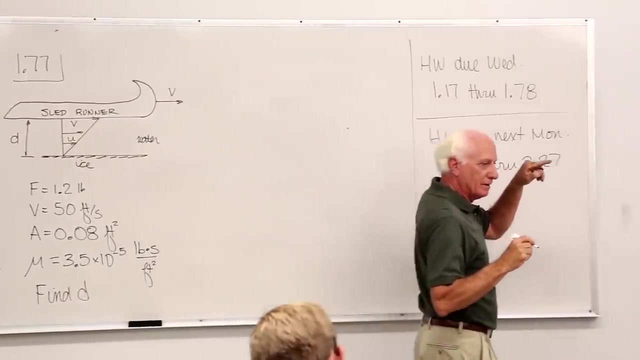 pounds seconds per foot squared. determine the thickness of the water layer under the run D. find D. keep reading. assume a linear velocity distribution in the water layer. assume a linear velocity distribution in the water layer. V is the velocity at the top of the water layer. it goes down to zero at the ice. 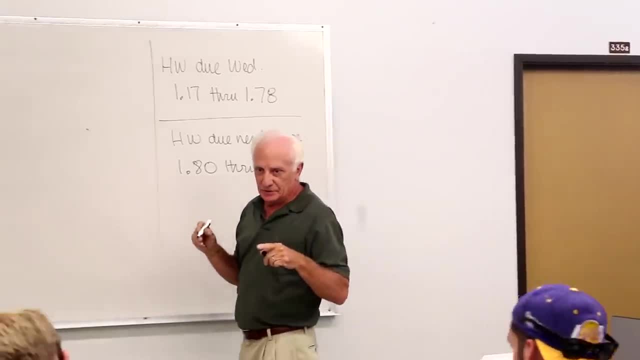 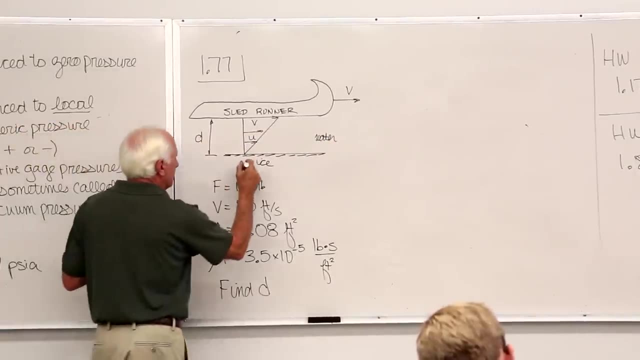 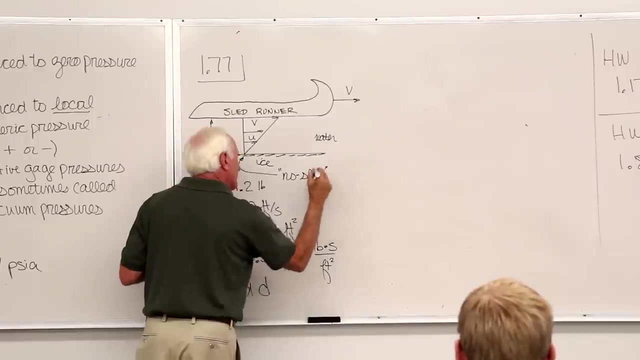 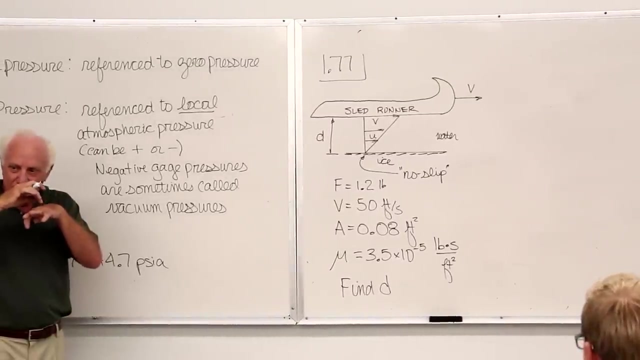 velocity at a solid surface is assumed to be at rest the water. it's called the null-state slip condition. right here this is called no slip. it means the water doesn't slip along the ice. the velocity of the water at the surface of the ice is assumed to. 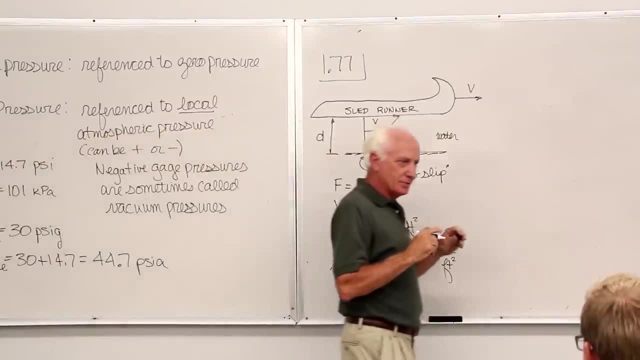 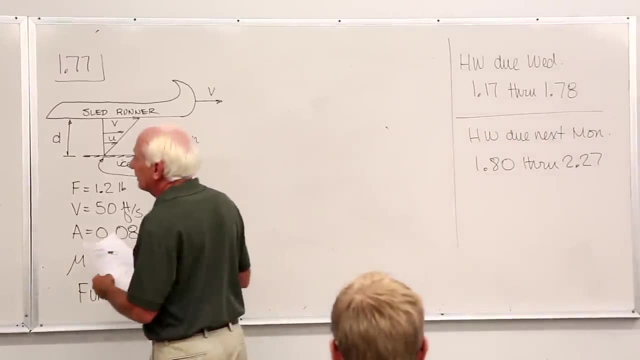 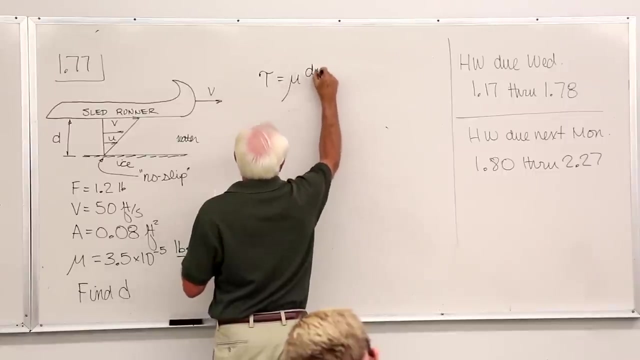 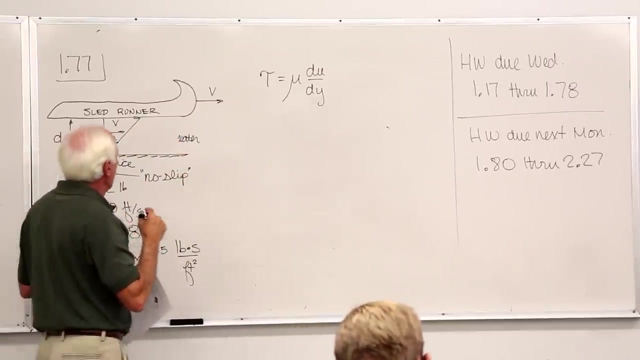 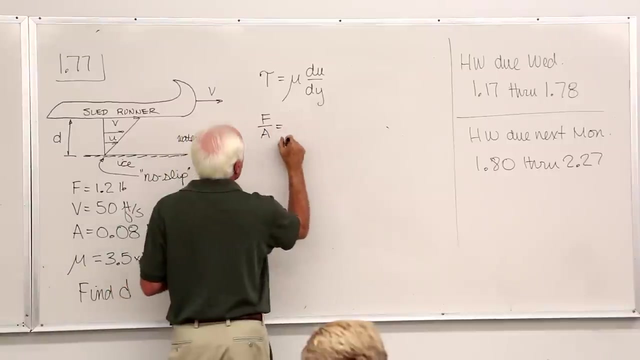 be zero, we'll make that assumption, pretty much drop this whole course. the no slip condition: okay, so I, recently I raised our equation. so I, recently I raised our equation. so we have our towel equal mu du 거야. okay, our shear stress, we know, is force over area mu du five. we're majoring why from here up like this: okay, force over area mu. we're measuring this, our G ratio, here also. we in this Linked衹, Mathuatejach, from what we use the volunteers will make. okay, our shear stress, we know, is force over area mu. du fear y. we're measuring Y from here up. and the amount accelerations that that let up and divided it from. oh we, you know, We had a Tau equal mu V Y and be Y ей, Carthage. we had not required and eating, we had a Tau equal mu V U by y. okay, our shear stress, we know, is force over area. Uits split the area. 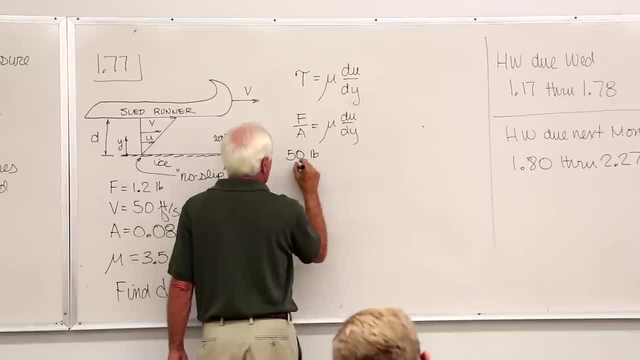 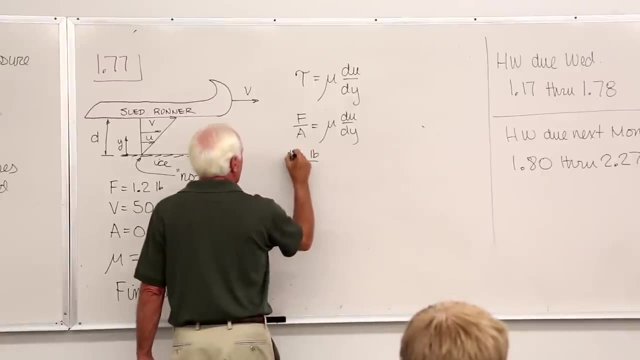 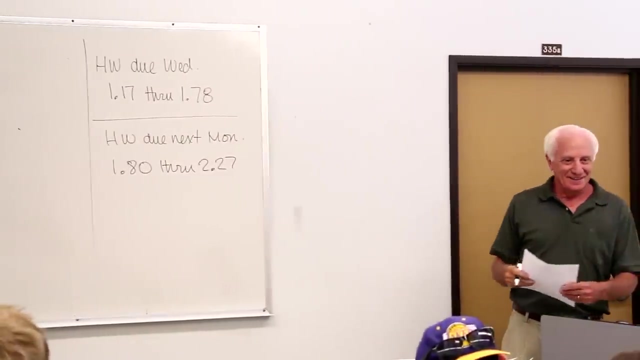 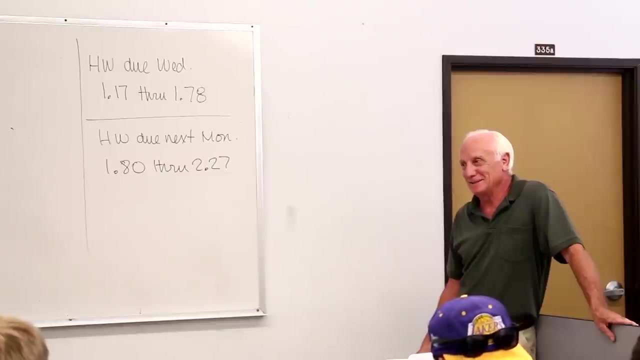 horse is 50 pounds. horse 50 pounds, Oh, 122 pounds. The last is 50. Which reminds me, if I put something on the board which doesn't make any sense to you, it looks like I made a mistake. Let me know right away. I don't want to have to copy the mistake on the paper and come back to the next class meeting and change it. So I don't mind, I've got to correct it right away And you know I'm not perfect, I make mistakes. 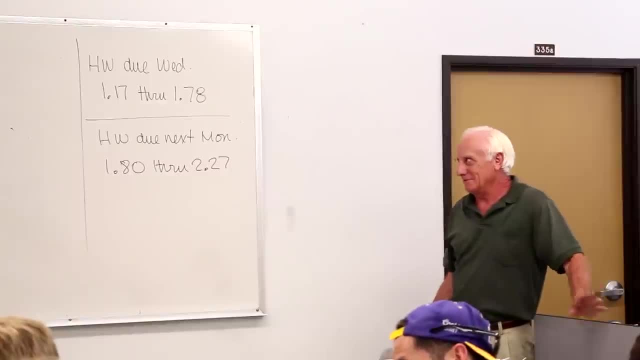 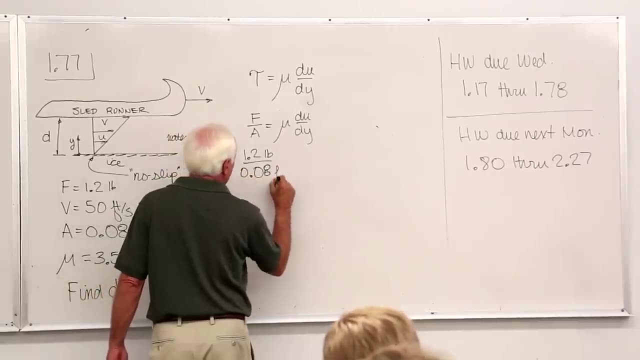 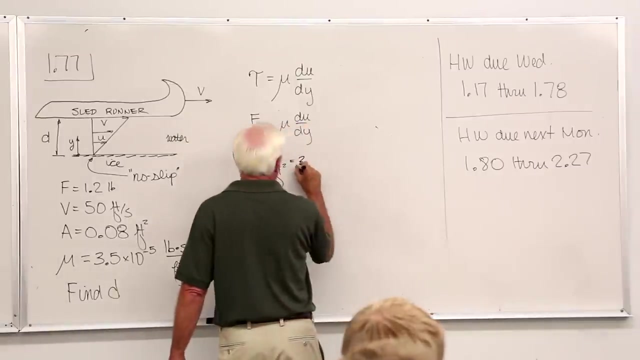 So just let me know and we'll change it on the board right away. Okay, 1.2 divided by area 0.08.. Equal mu- okay, there's mu right there. 3.5, 10 to the minus 5.. Pounds second or foot squared. 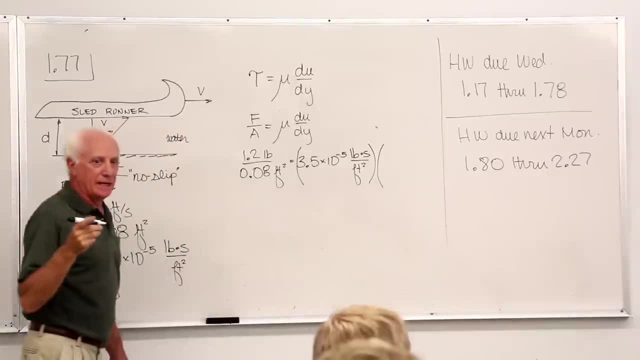 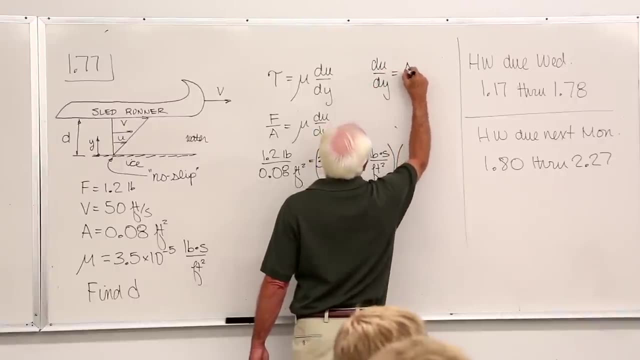 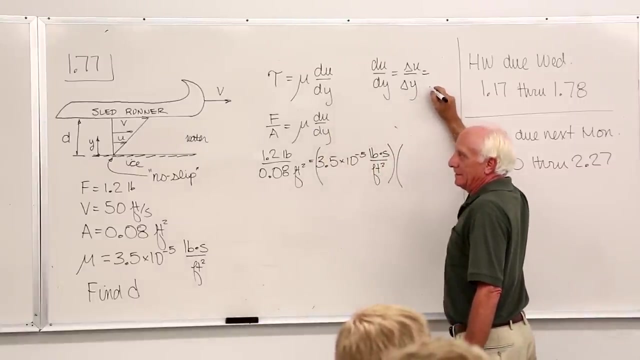 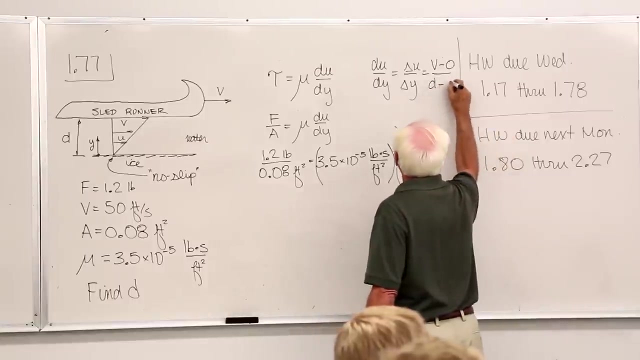 Multiply by du dy. Don't forget, it's a linear profile. So you know, lucky you du dy. if it's linear, equals delta u over delta y. Delta u at the top v at the bottom 0.. Delta y at the top v at the bottom 0.. There it is. 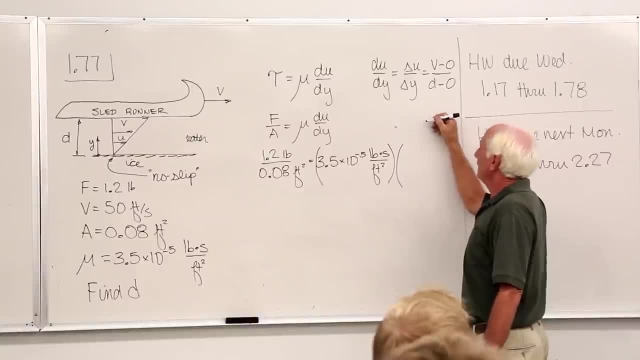 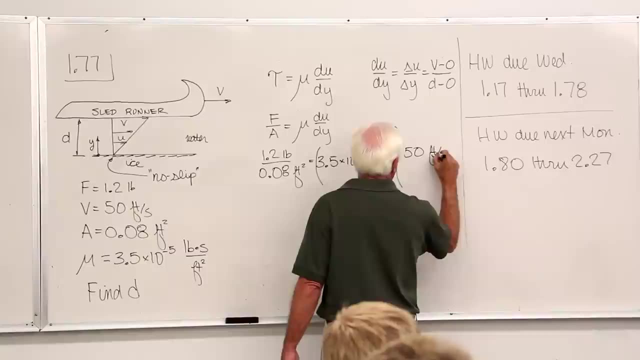 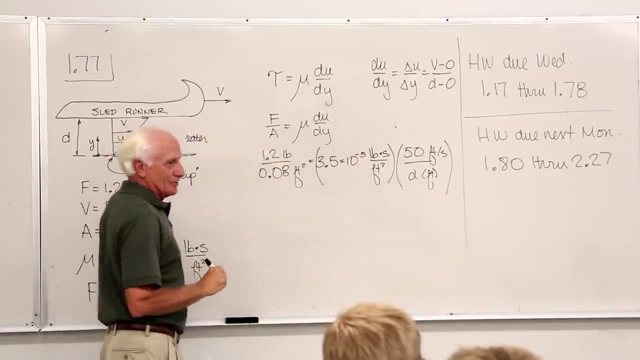 du dy is delta u over delta y. Delta u at the top, v at the bottom: 0.. Delta y equal v over d v 50.. d going to be feet. Check it out, It's going to come out right here. 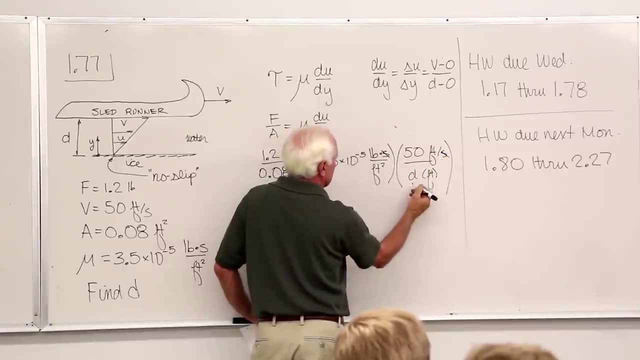 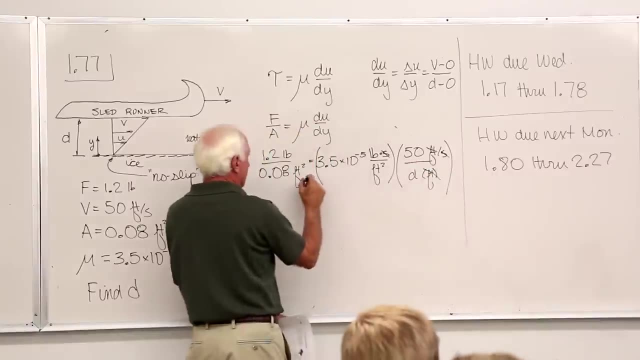 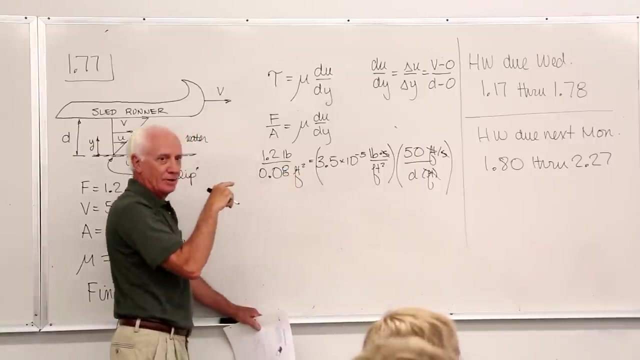 Okay, seconds divided by seconds. Feet feet squared. feet squared here. Feet feet gone. The right-hand side pounds per foot squared. left-hand side pounds per foot squared. good, We're good to go. It's all for d. It'll be in feet. 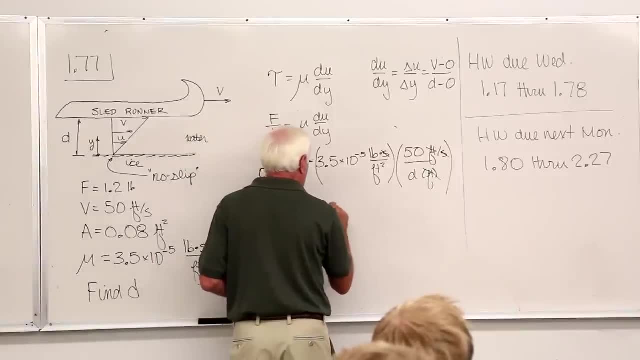 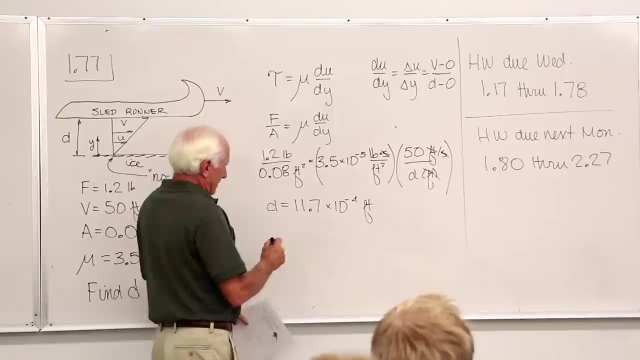 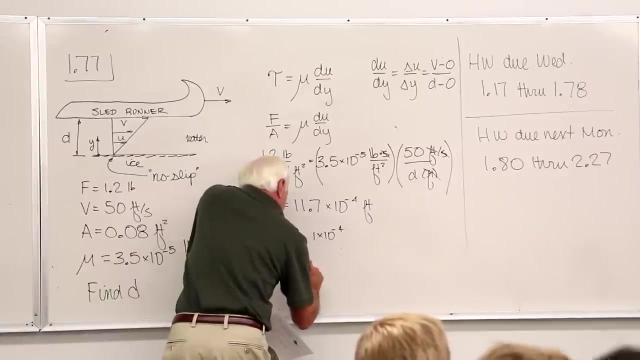 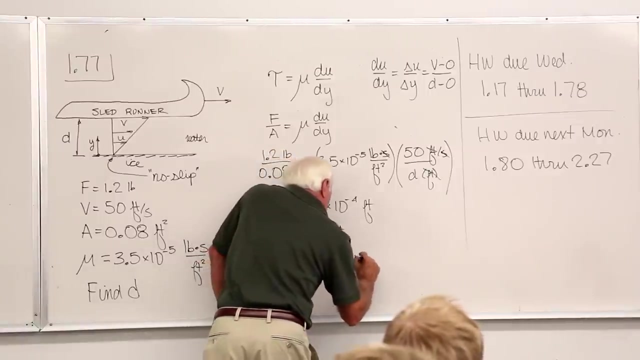 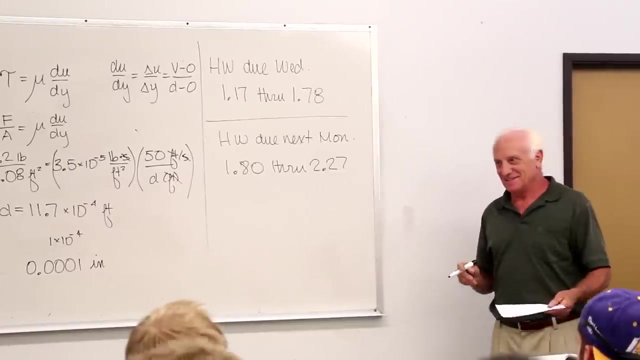 7.7, 10 to the minus 4.. 10.7 times Okay. 1.. 1, 10000th of an inch. 1, 10000th of an inch: That's the amount of liquid water between the blade surface and the ice in the King's Hawk and broom. 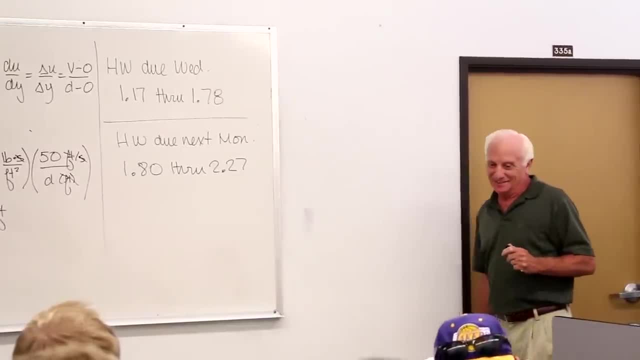 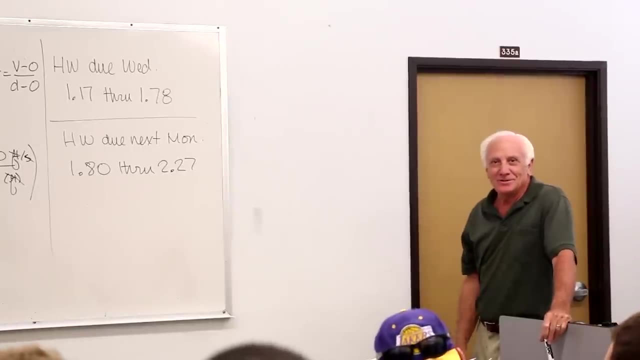 Not a lot, doesn't take a lot. It doesn't take a lot, but there is a layer of water under there, Out of out of here. Okay, I did that just to kind of show it. Matt, did you give me a signal? I'm sorry about that. 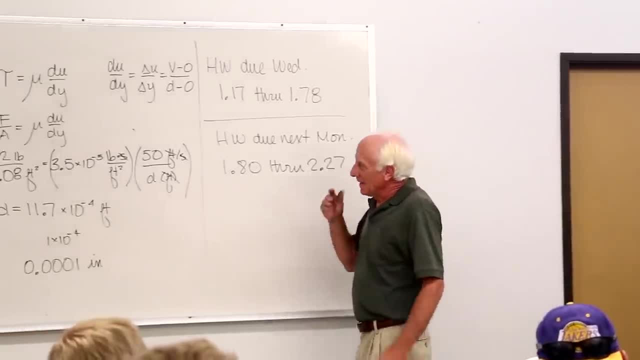 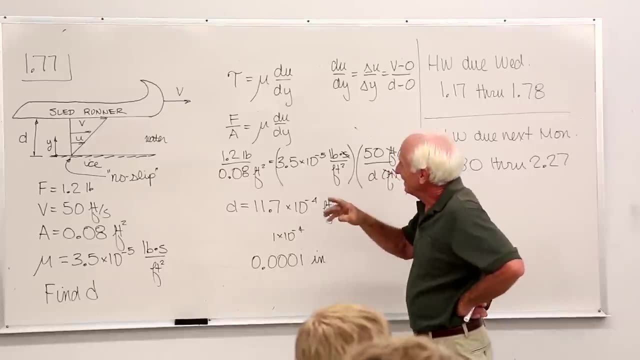 No, I got it. Okay, thanks. I want to show you how you set up the homework problems And I'll move it again when you pass your first homework statement. But do that? The first thing you do is you draw a sketch if it's appropriate. 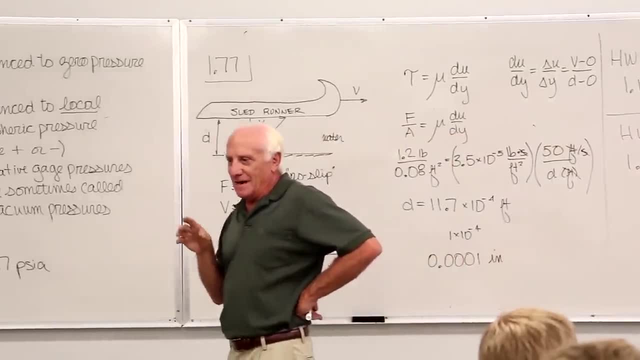 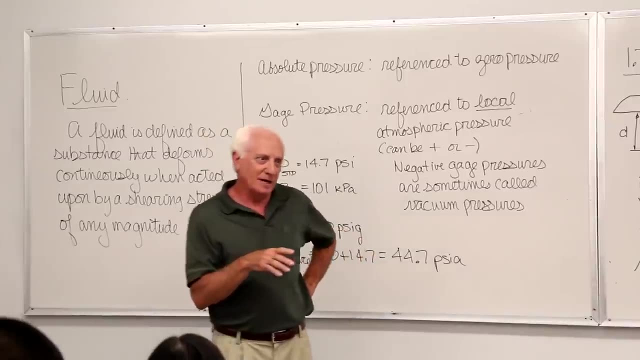 I mean, we're engineers, We love sketches. If you're a mathematician, you love equations and you hate sketches. You want the theoretical solution. If you're an engineer, you love pictures and you'll do the math because you have to do the math. 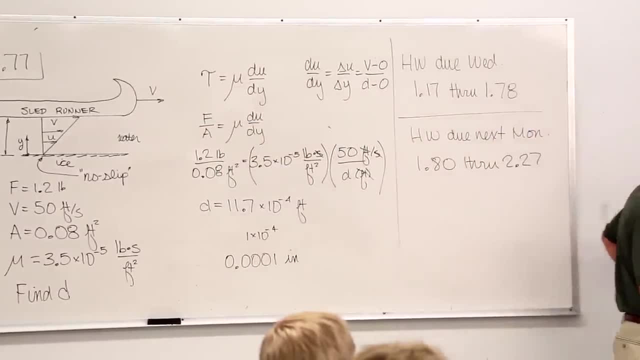 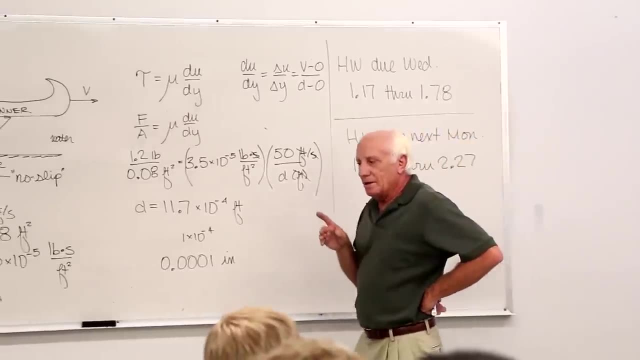 You don't love the math maybe, but you do it because you have to do it. Do your toolbox. So most engineers think more clearly if they have a picture On an exam. I guarantee that if you try and sketch something on an exam, 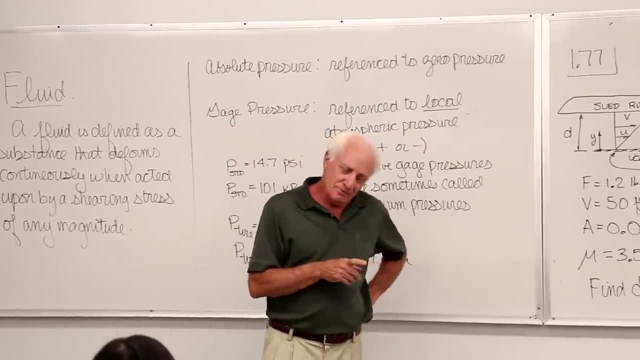 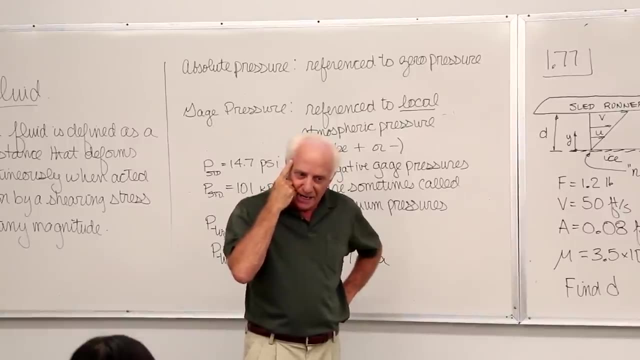 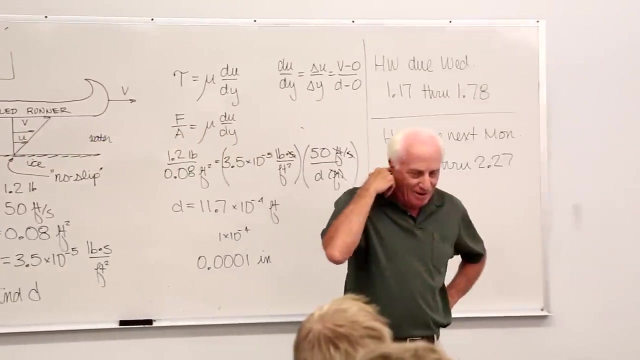 whether it's a pre-body diagram, which is essential, maybe 214,. what it does to you is it builds a time delay in your brain. You don't start writing down and putting numbers in something And you read the problem When you sketch it. your mind is working in the background. 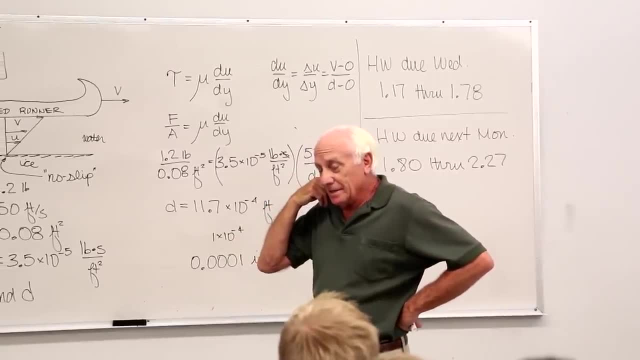 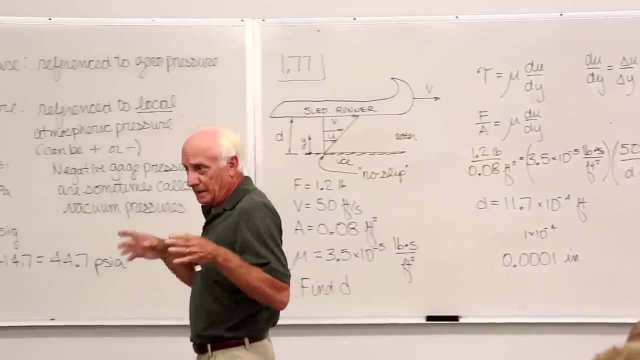 Believe it or not, And it makes life a lot easier if you do it that way. I guarantee it, Because the way you get flustered and frustrated is: try and start putting numbers on that hand-held calculator right away. Oh, that's just a story. 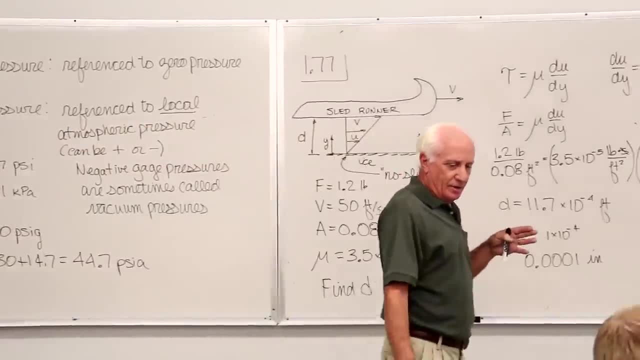 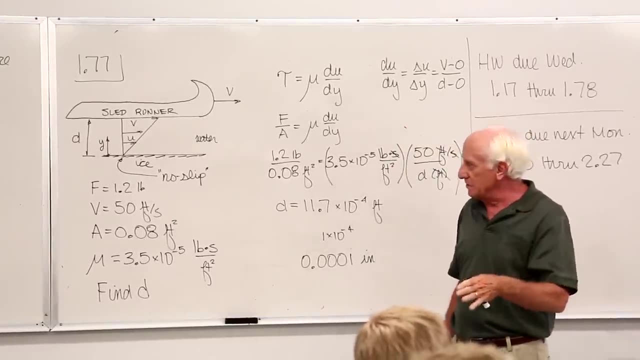 If you're unsure of yourself, that puts you down, way down. What you do is you build about a 60-second time delay in there. so your mind starts to think about that problem, And one of the best ways to do it is to draw a picture. 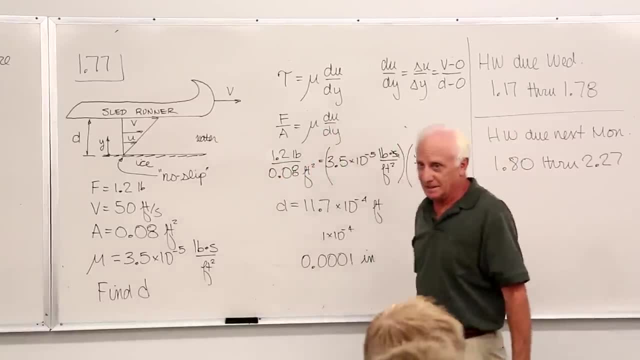 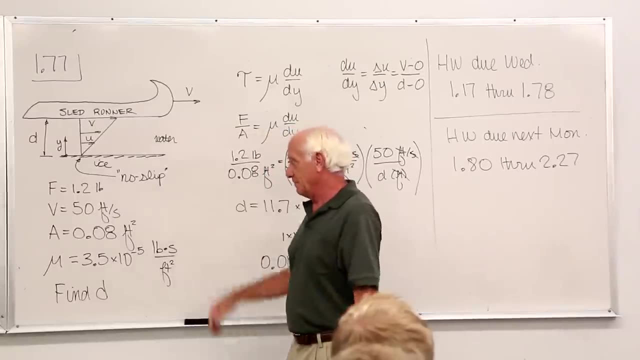 When you draw that picture, your mind starts to think: It's amazing, The engineering thought process. So anyway, if it's appropriate, draw a sketch. Once you draw the sketch, I don't care if the problem has it listed there in paragraph form. 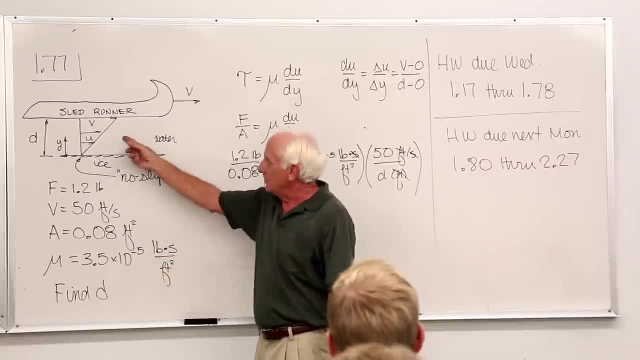 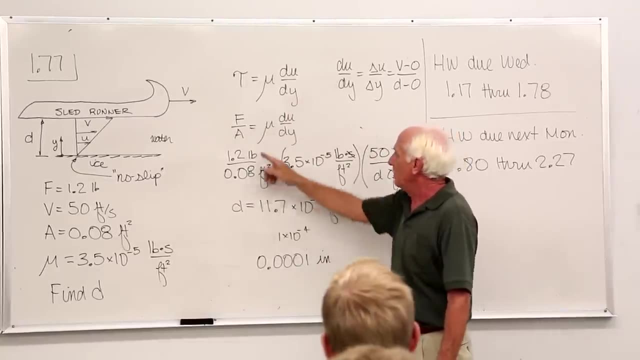 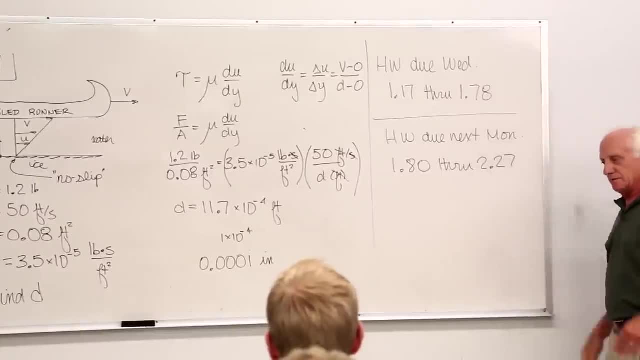 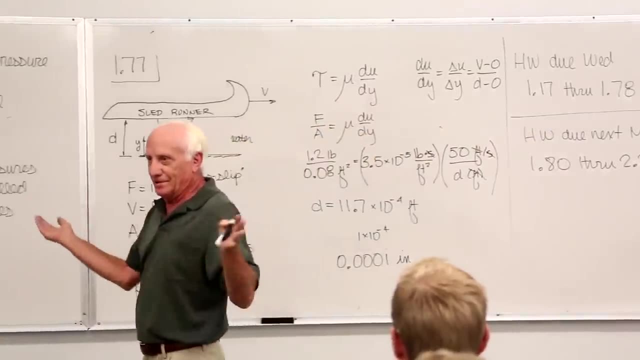 Your mind starts to think like that. So much of engineering is having an approach to solve a problem. We're not in the backyard, you know, in your garage making something. We're not doing that in your garage. We engineers are trained to think correctly. 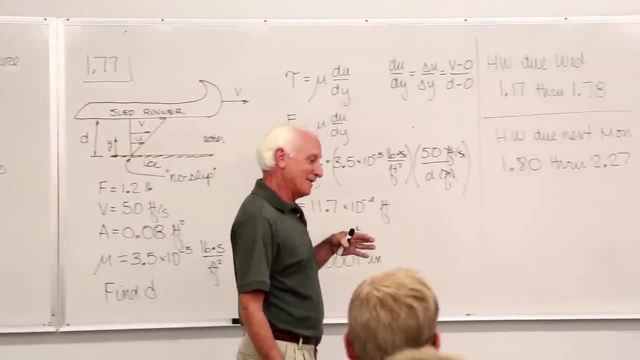 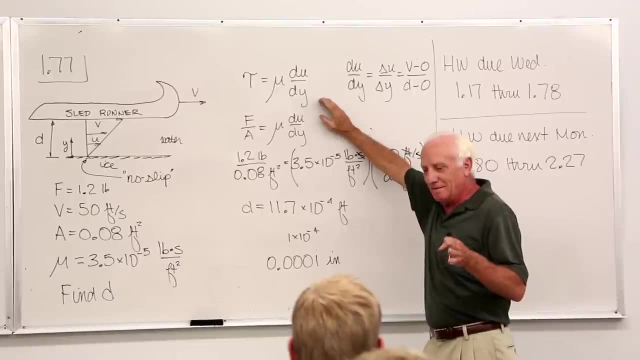 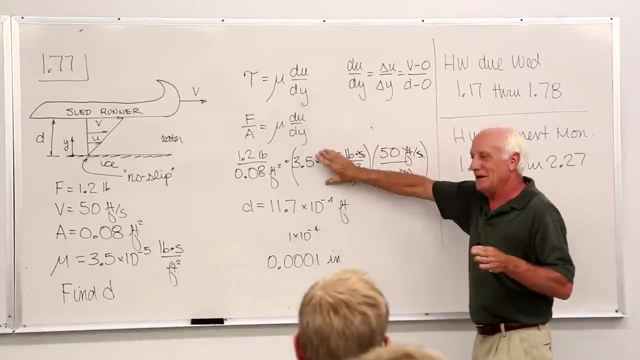 It's pretty fascinating, Pretty fascinating. Okay, next thing, you do Put the equation down in symbolic terms. I don't want to see any numbers in there until you write the equation down, so I know you're using the right equation. Then you put the numbers in. 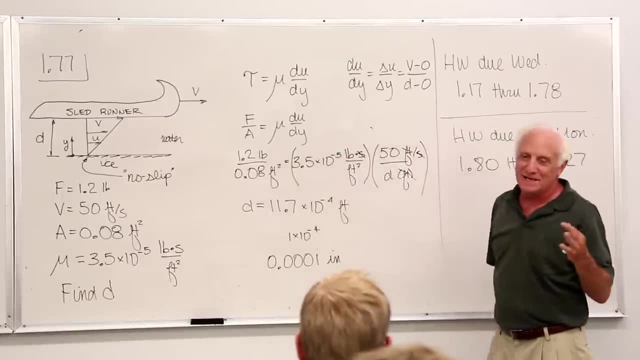 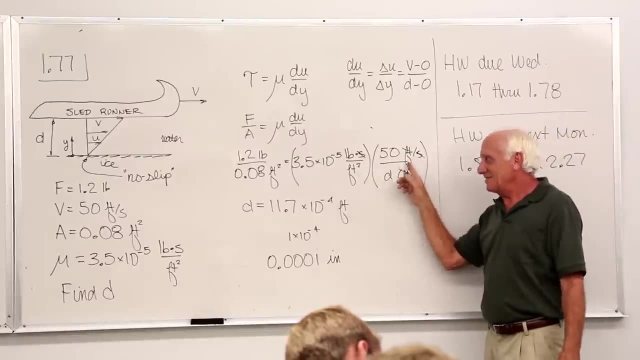 Then you put the units by each number. I'm repeating things I know have been beating your head for three, four, five years, But I'm going to do it one more time. Put the units in, Cancel them out, Like this: 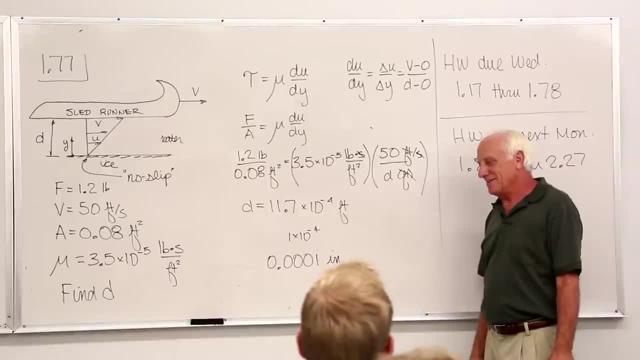 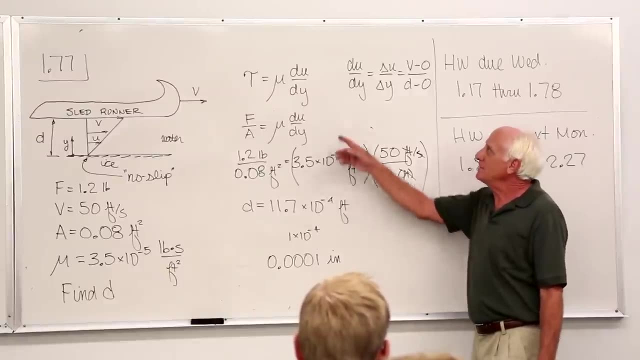 And end up with what you want. All those steps are important steps. If you do them in the right order. you may be amazed how things kind of fall out. There might be three or four possible equations. You might write down three equations. 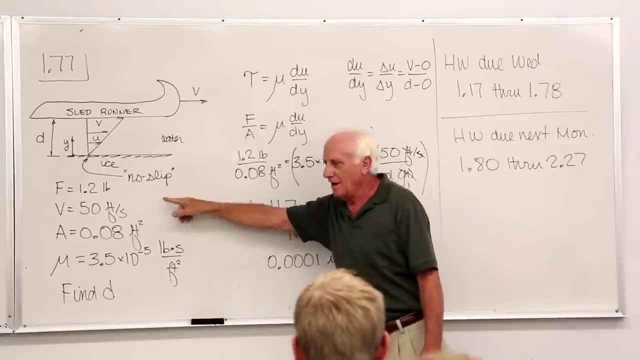 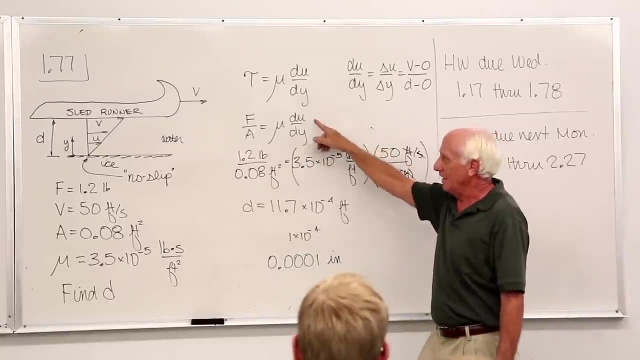 You look at the equations, You look at this over here. You say, no, that's not going to work. One equation, two unknowns: No, that's not going to work. One equation, three unknowns: Yeah, he's going to work. 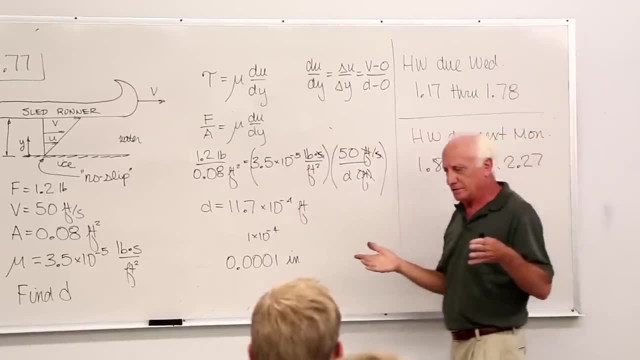 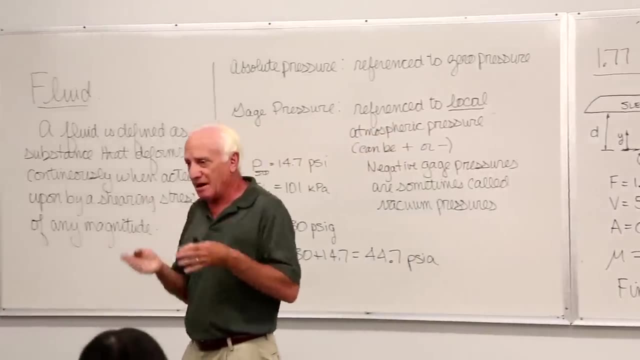 So you don't always know. You don't always know which equation might work at the start. Sometimes you do, Sometimes you don't. But if you don't write down the equations you think might work, and stare at them, Stare at them a while. 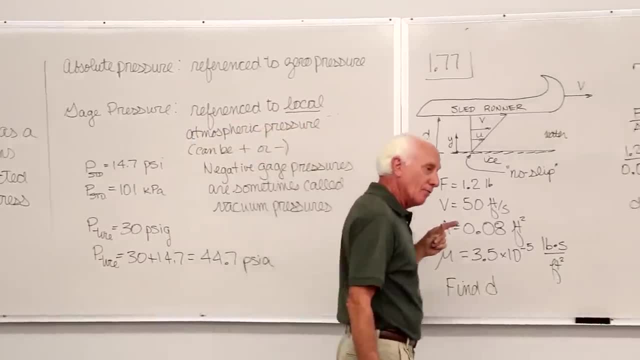 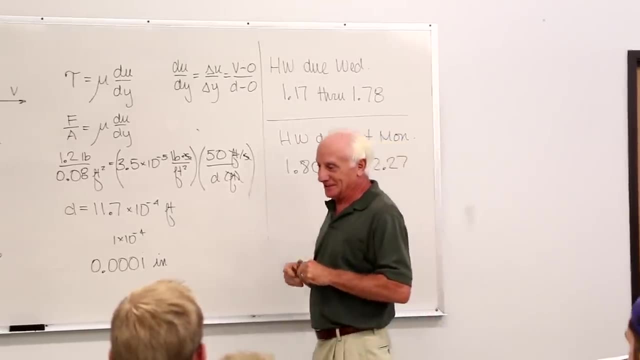 Maybe something will jump out at you, Whether it's homework or an exam, And I'll tell you something else: You don't get ready for an exam by copying solutions. many, No, no, no, I mean, you know, you know. 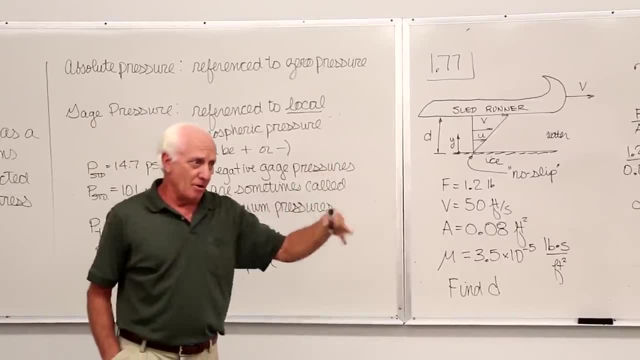 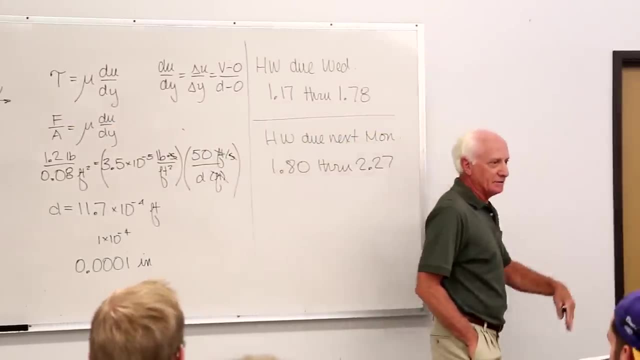 Tell Kershaw: you know, Did you read how to throw the curveball before the game? He said: are you kidding me? No, I don't do stuff like that. I throw it myself 50 times. on the sidelines I develop a new pitch, a slider. 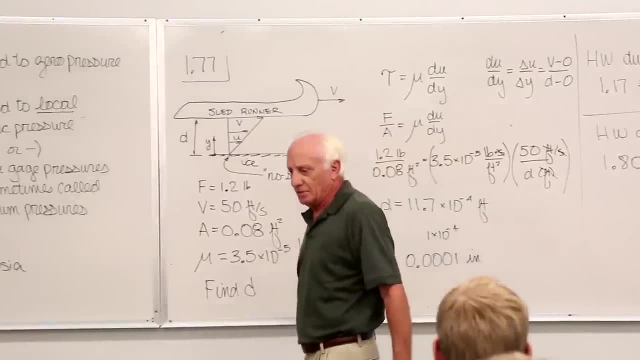 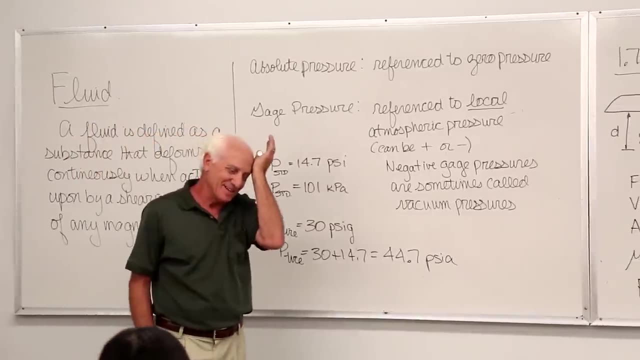 How? No? no, I practiced it. I threw it 1,000 times on the sideline. You don't get good until you suffer through some homework and say, gosh, I just don't get this. I went through that. 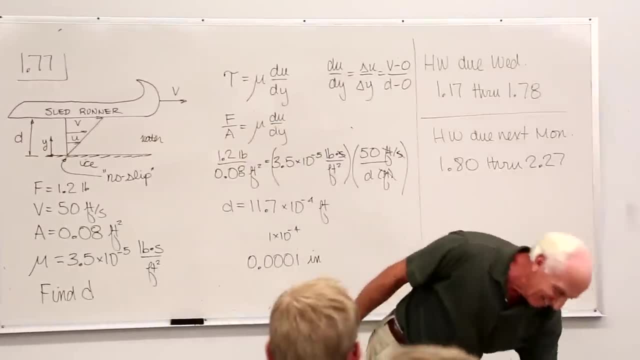 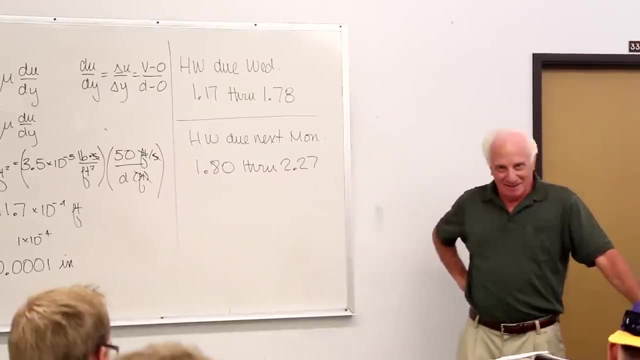 I get so mad sometimes I think like this: I go, I don't know why I'm not getting this At home. you know, nice music on touching my hand, But I still got mad. I got so frustrated and flustered. 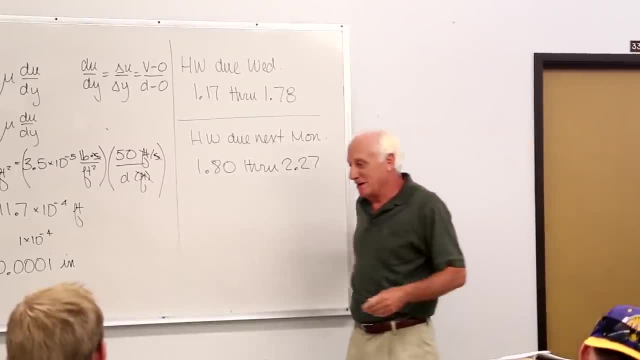 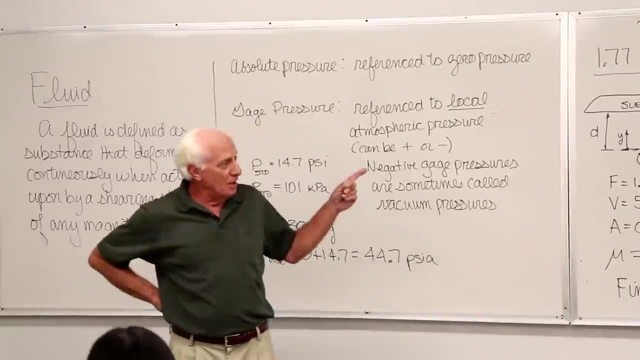 But I worked my way through it And boy, you're better for it. You're better for the pain. The way you get ready for exams is. you're not surprised. And how are you not surprised? You look at all the problems in working class. 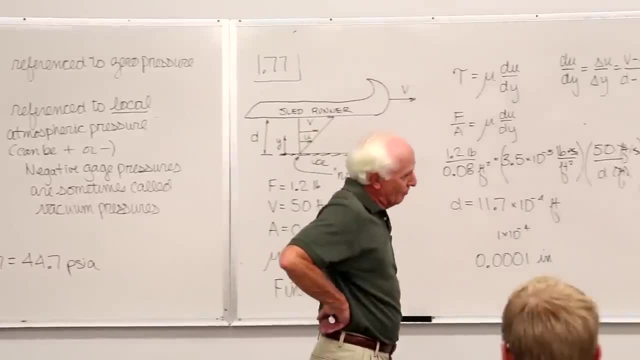 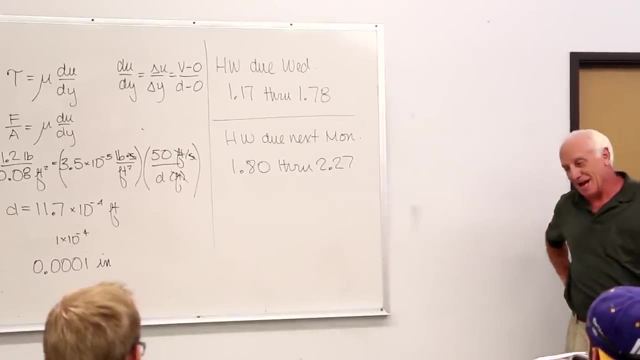 You read the example problems in the textbook And you go over homework. Don't read their solutions, Because you won't be ready for the exam. Oh sure, you've seen the solutions, But on an exam you won't be ready. 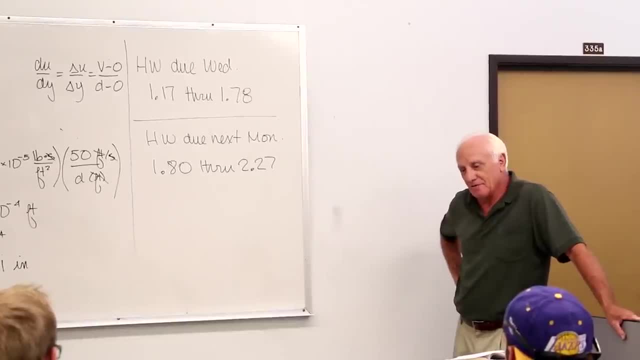 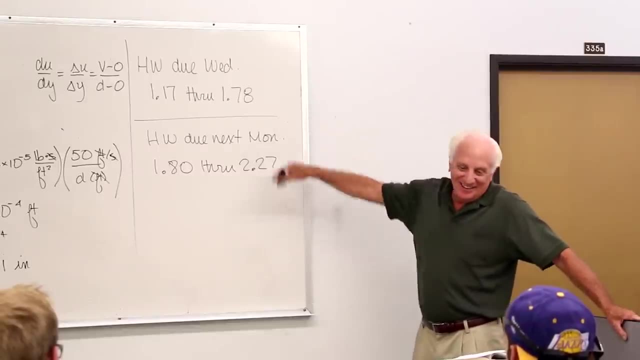 You've got to practice yourself And put yourself in a tough spot, In a real tough spot. Okay, We have finished Chapter 1.. Here are your assignments for the next two class meetings. Oh, by the way, my office hours I can make other times: Monday, Tuesday and Wednesday. 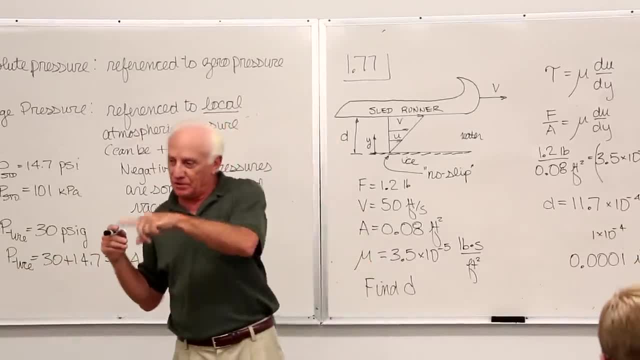 I'm here all three days. If those office hours don't match with yours, let me know. We can meet another time. We can meet another time of day. That's fine, All right, We'll see you then on Wednesday. Bye. 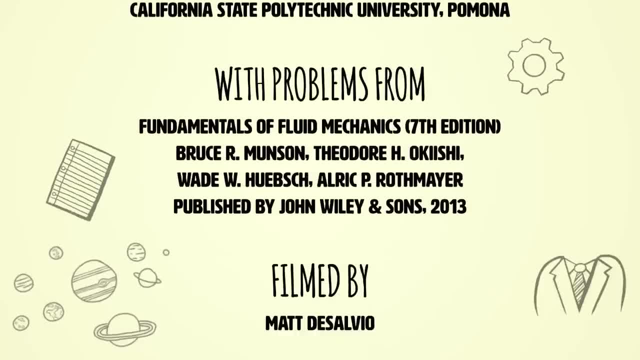 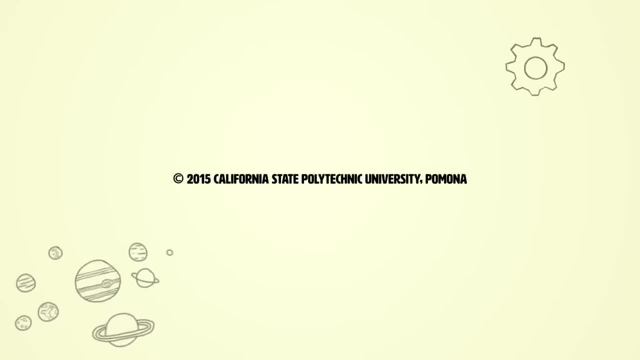